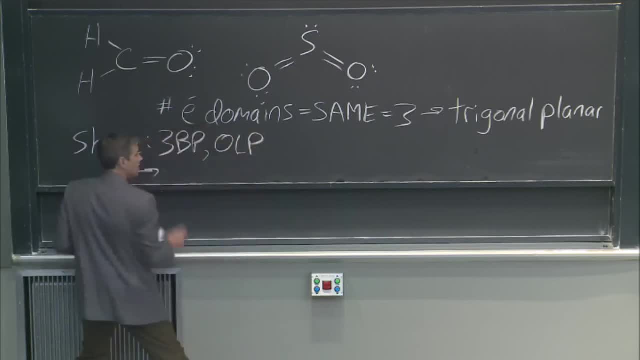 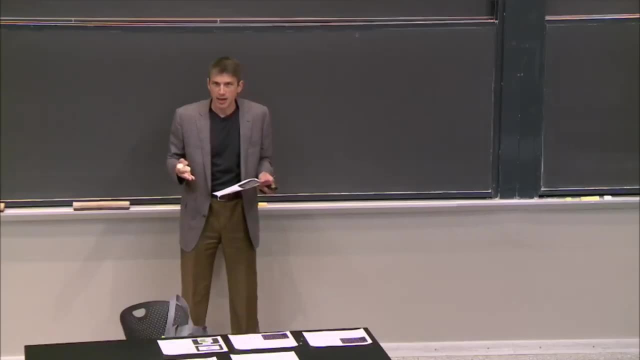 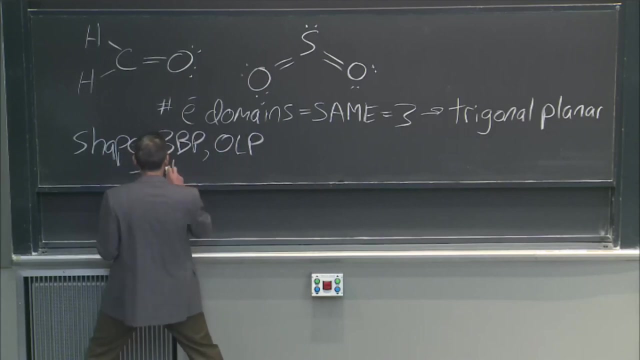 what the table was about was the number of lone pairs. Okay, The number of lone pairs. And so if I've got the three bonding pairs and no lone pairs, then it's going to be a trigonal planar shape. So that is trigonal planar, And over here I've got two bonding pairs and one lone pair. 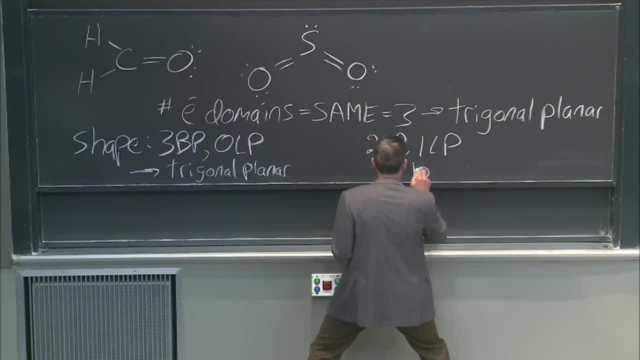 And so this shape is called bent. Now, what I did is- I use that word, Oh why, I don't know. But you know you make mistakes when you're in the arena. you keep going, And if you make a mistake, you admit it, you leave. 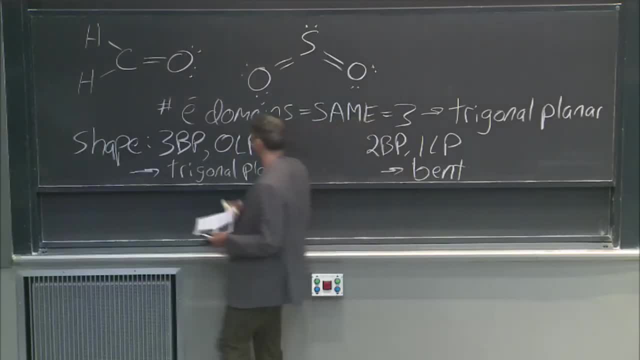 it all there. You do your best, Forget the rest. That's all you can ever do. Now here's the thing I said: bent. I said the word bent, And what I was talking about was how that bends a little bit. 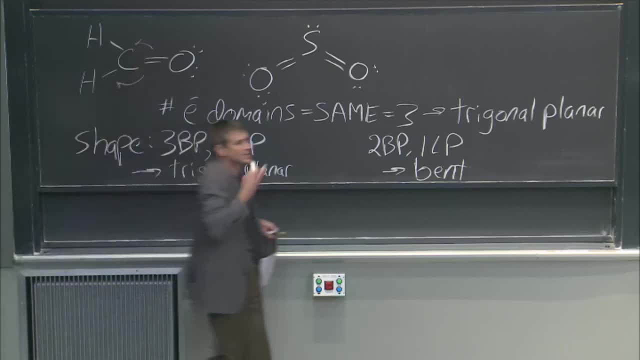 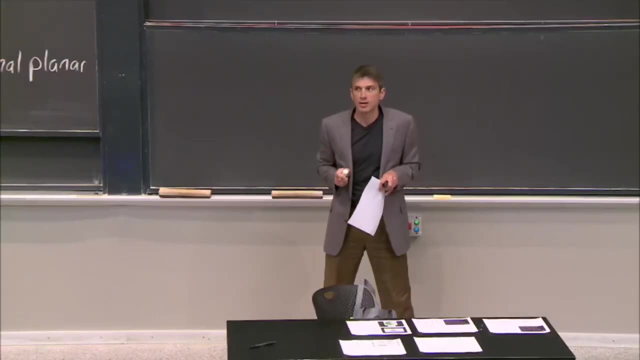 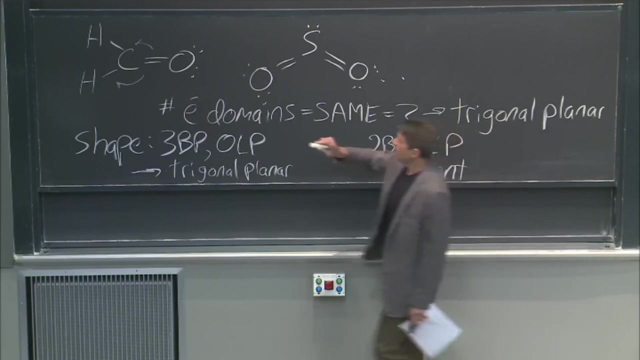 because of the repulsion order, Yeah, But that that shape is not bent. I want to be real Clear about that. That shape is trigonal, planar and it's a little bit distorted. Okay, This shape is bent. That shape is bent, and because it's a, it's got a lone pair. Remember the shape. 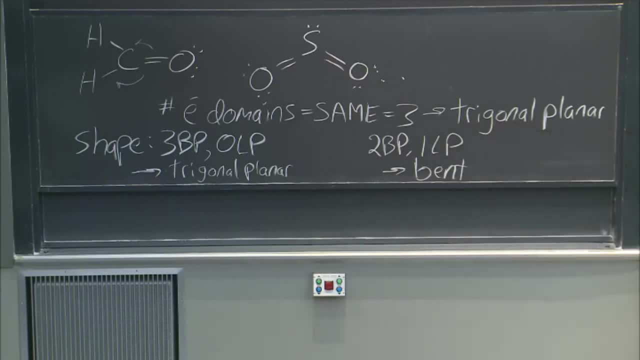 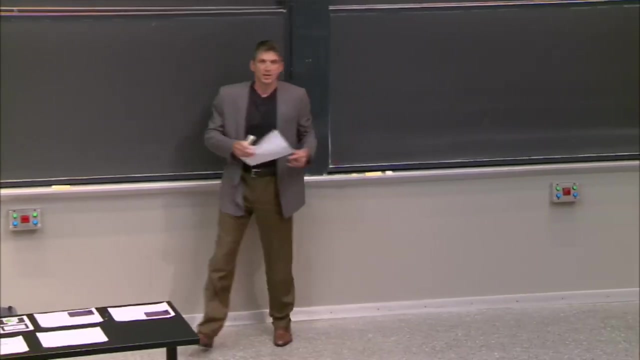 is about where the atoms are, right, But it's also a little bit distorted, right, Because the lone pair pushes on those guys a little bit more, All right, Okay, So that those are the two concepts that I was saying all at once And I want to make sure we understand them. There's trigonal planar. 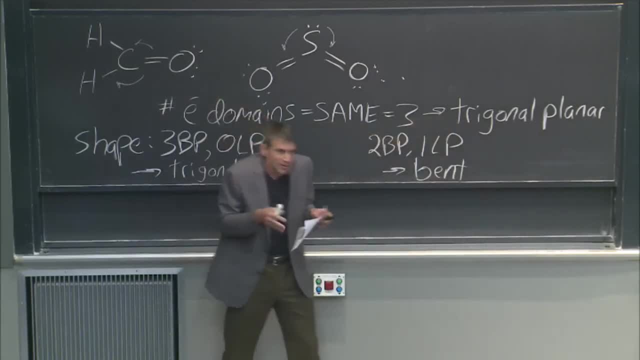 there's bent and then there's repulsion order, which talks about a little changes in the angle from those parent shapes. Okay, good, All right, Now onto today. Now here's the thing. In all this stuff with Lewis, it's a really good way to think about molecules, But this tells me that there's 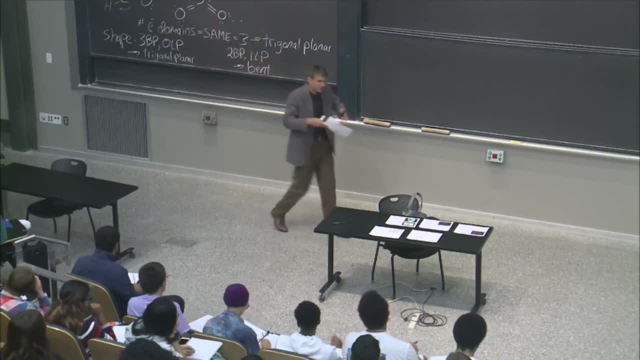 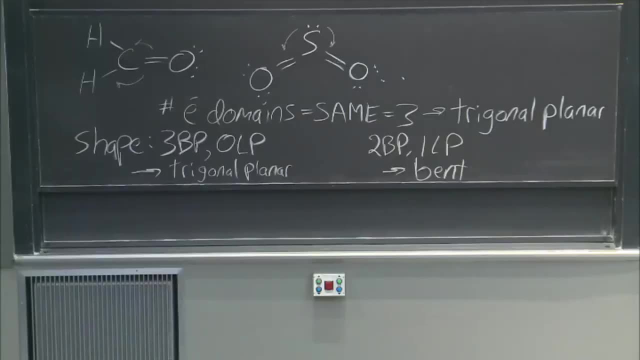 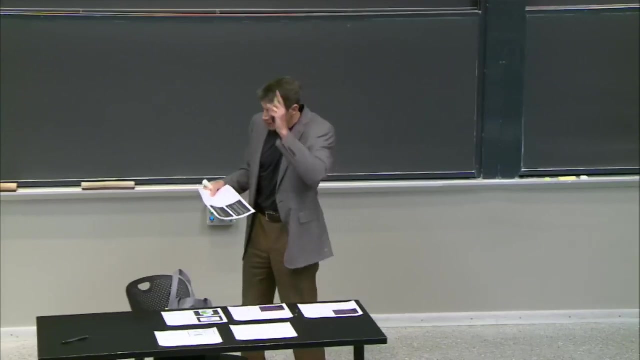 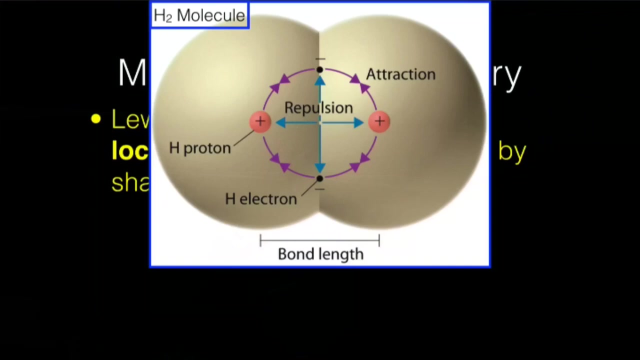 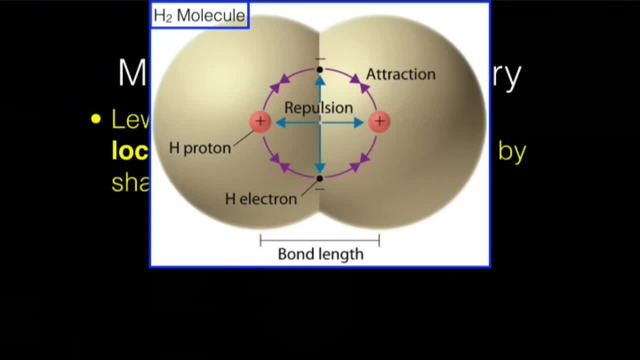 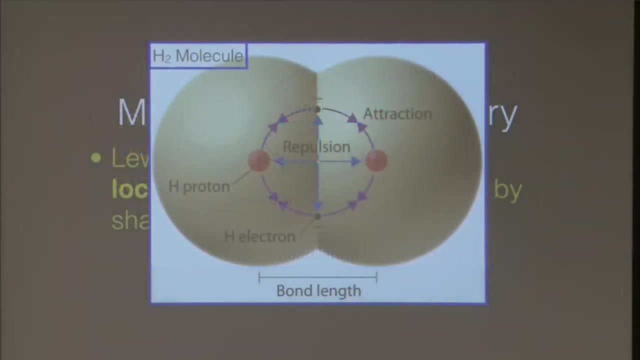 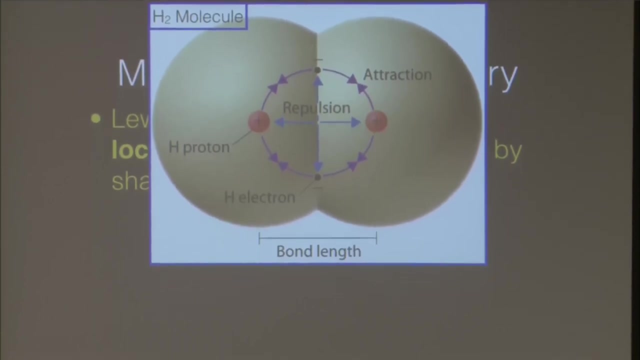 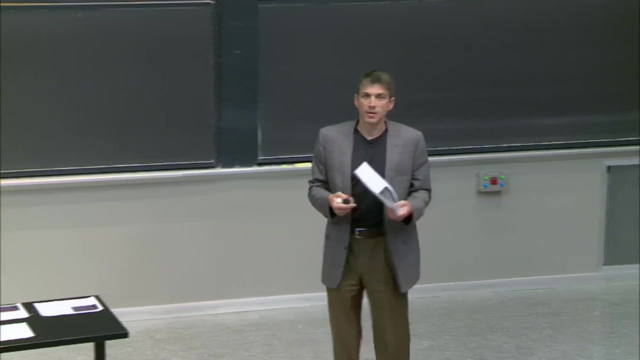 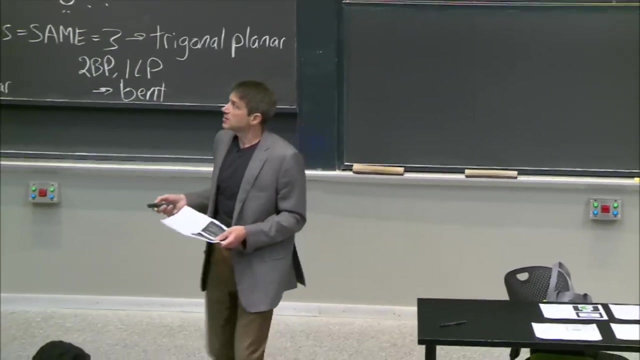 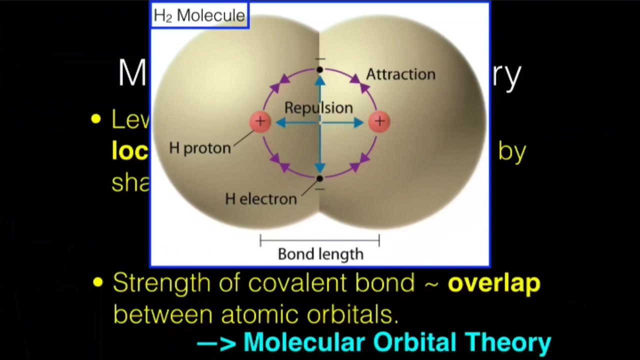 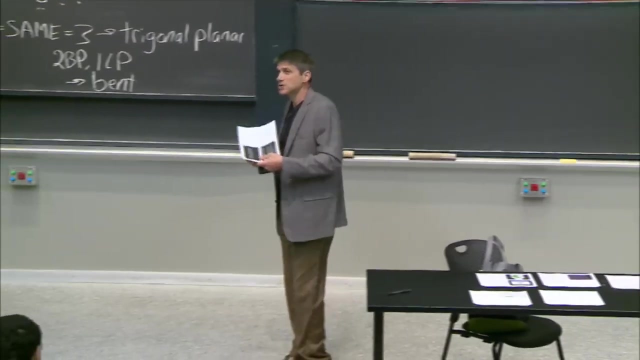 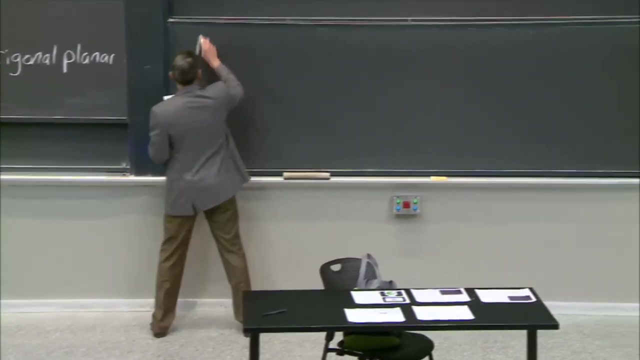 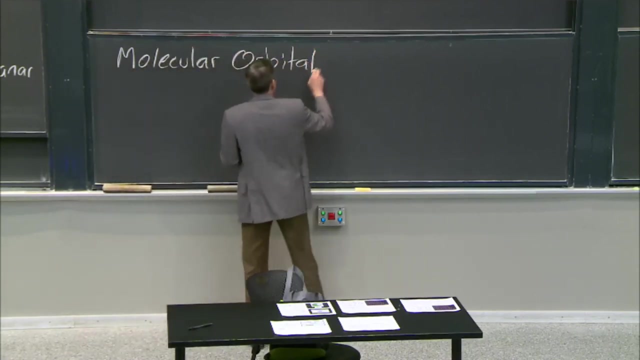 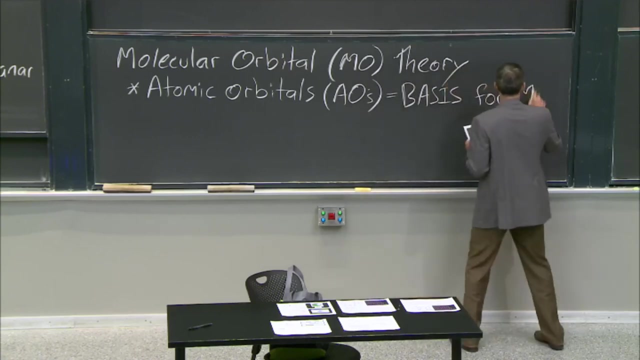 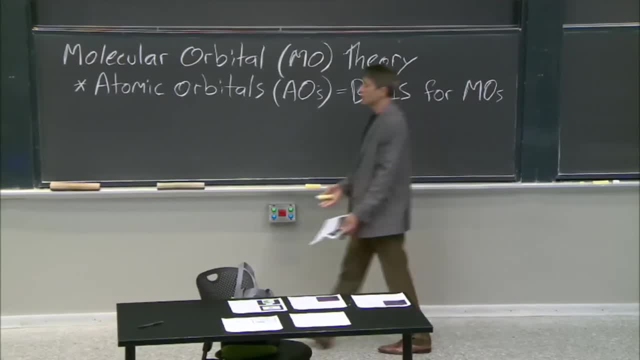 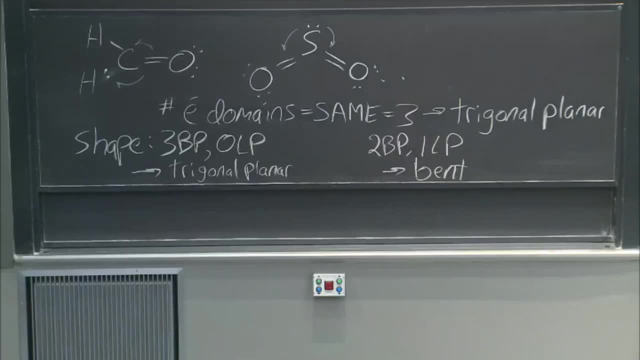 I didn't have to write it again, right? Okay, so what does that mean? Well, it means that I'm going to construct the MOs from the AOs. Now, the AOs are the things we've been playing with and making right. 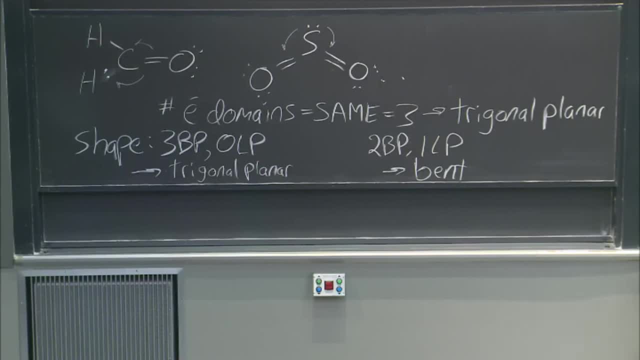 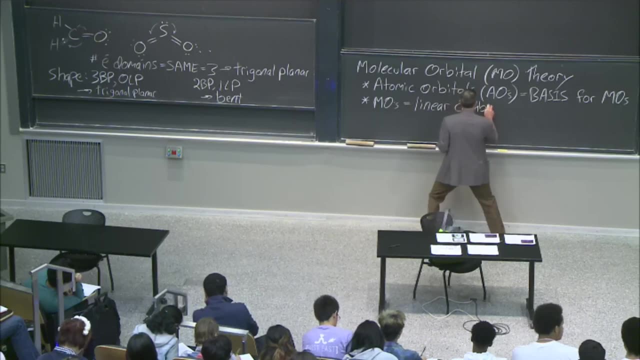 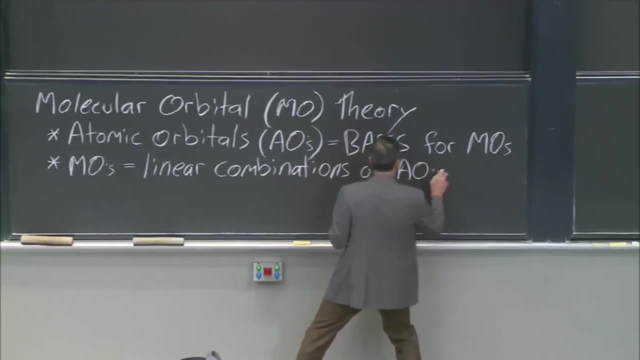 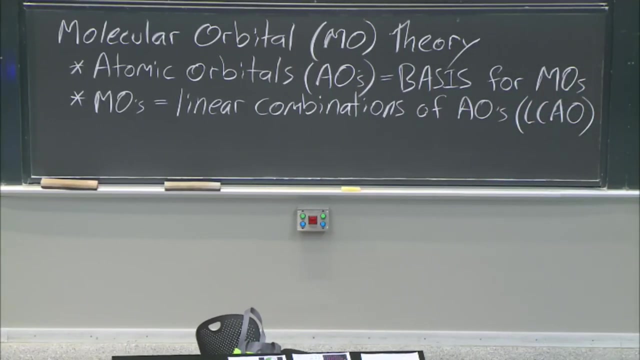 We solved the Schrodinger equation. So the MOs, okay, are going to be linear combinations, All right, combinations of the AOs, And that's why you might see this, in fact, called LCAO theory. LCAO- linear combination of atomic orbitals. 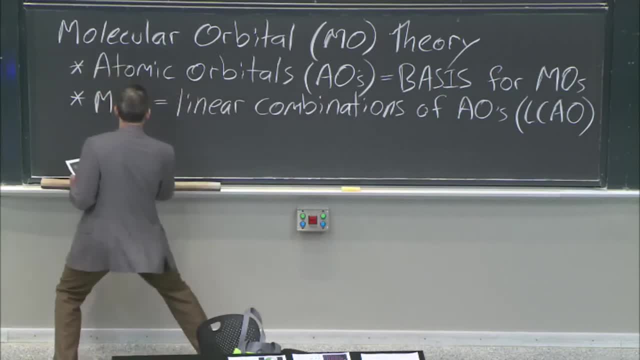 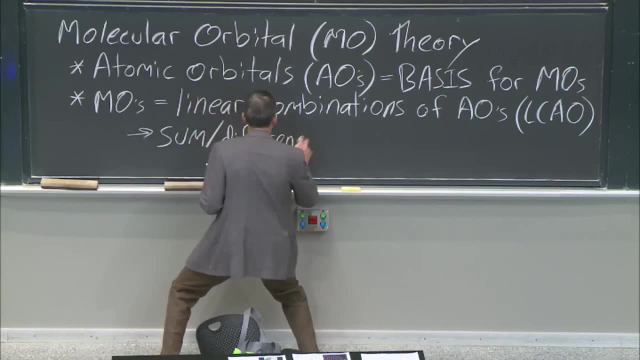 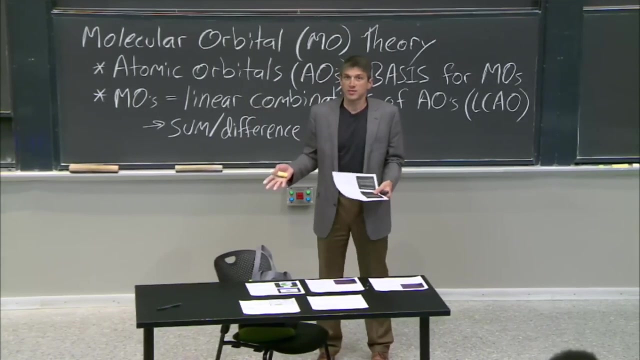 Okay, And, in particular, sum and difference of orbitals is what we're about, Because, you know, this is like what we talked about before. These are waves, right, These are waves. Waves can either constructively or destructively interfere. 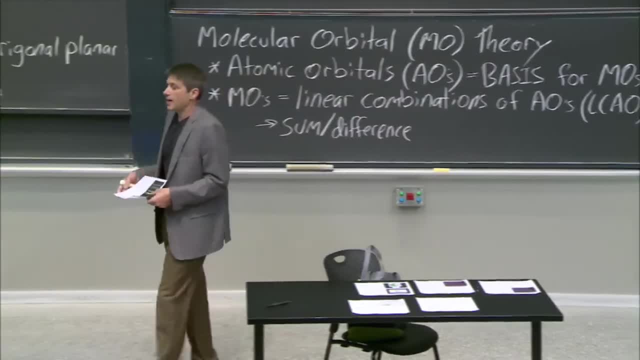 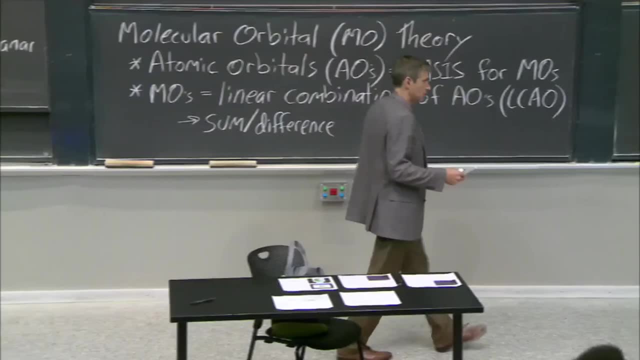 And that's what we're going to explore in MO theory, By adding or subtracting, By subtracting these wave functions, these orbitals, these atomic orbitals. So that's enough to start, Let's see. So look, basis. 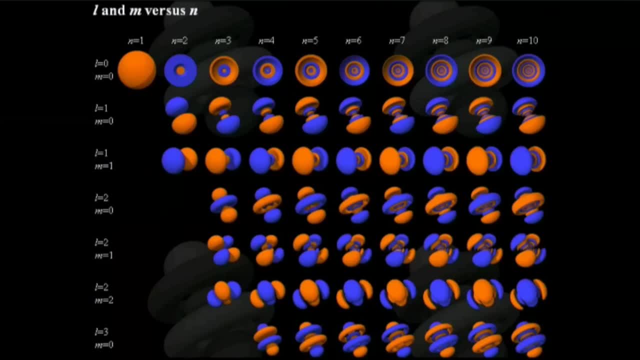 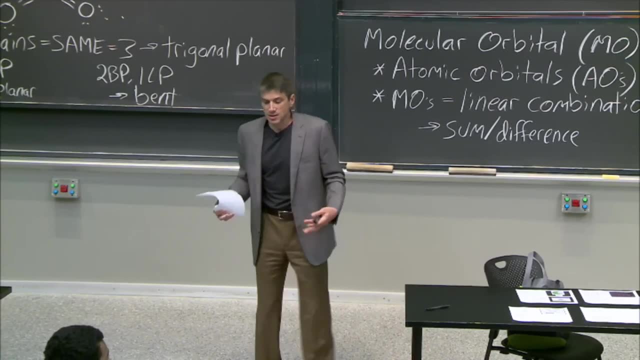 A basis is nothing more than the things that I'm going to use to represent the things that I want. Right, And the things that I want are these molecular orbitals, And the things that I'm going to use to represent those are these. 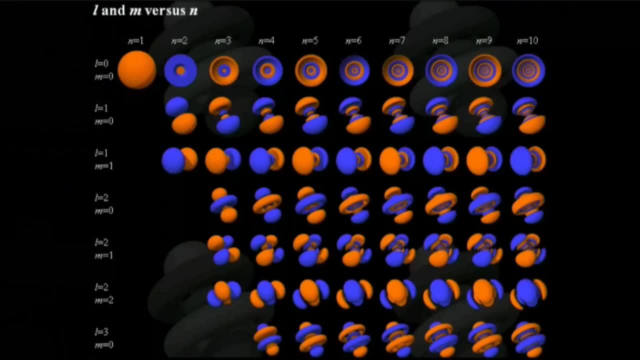 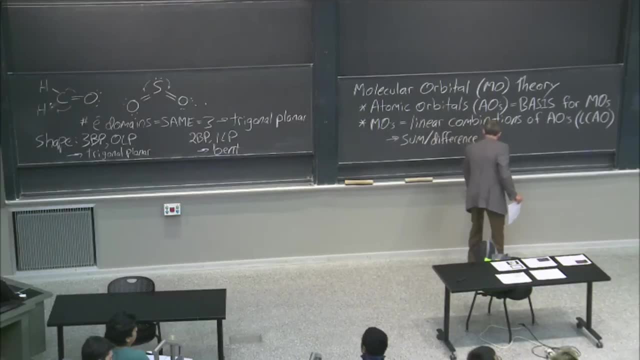 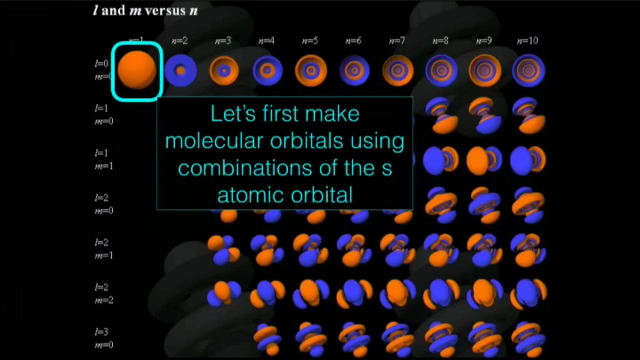 These beautiful atomic orbitals that we spend a lot of time understanding and developing. We'll start with the simplest case, which is: well, I think I have, oh, I even highlighted it And I said: let's first make molecular orbitals using combinations of the? s orbital. 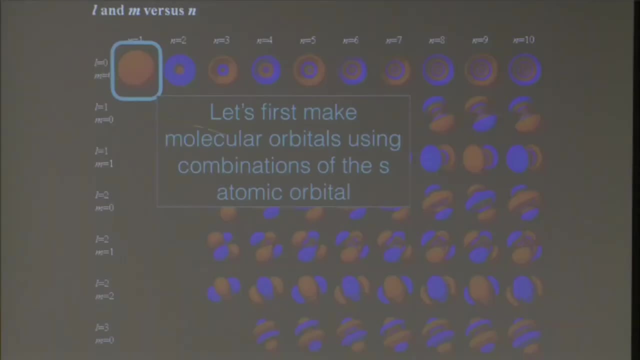 That's the s orbital. That's the one s orbital up there, Remember, by the way, blue and orange is just the sign of the wave, right, This is not a charge. Please don't make that, Uh, that confusion. 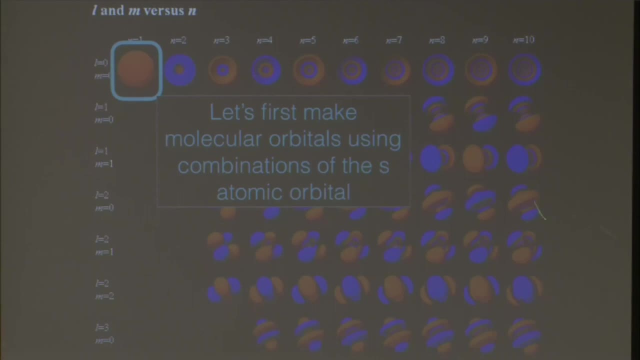 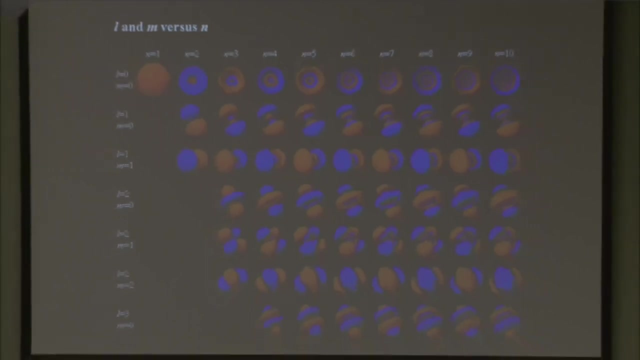 These are just waves, right, Waves, Okay, And the p orbital has. let's go back and see it. P orbital has a plus and a minus. It's a wave, All right, And the s, the 2s orbital, has that too. 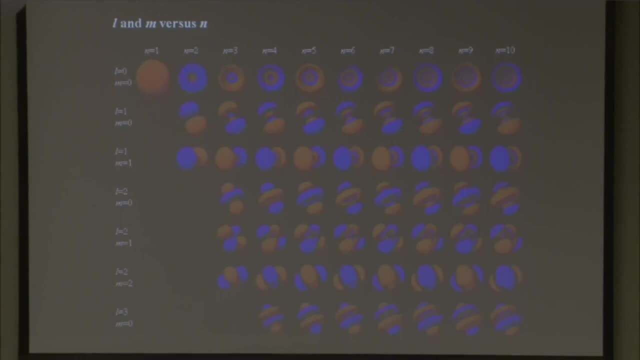 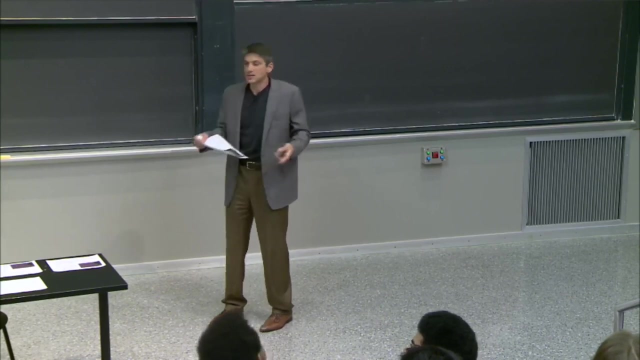 And you square it and you get the probabilities Right. Okay, So we'll start with 1s, where it's all just one sign And I can add it. I can add an s and another s, or I can subtract it. 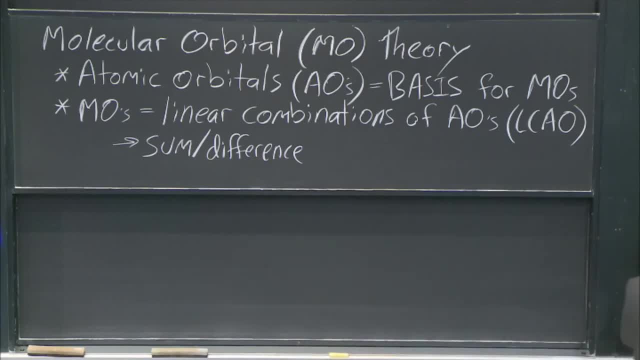 So let's do that Right. So we'll do that over here. All right, Oh, Let's see. So we'll do that over here. So if I take a 1s orbital and I add it to another 1s orbital, 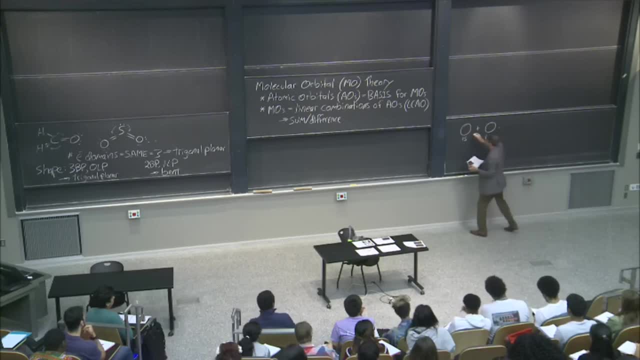 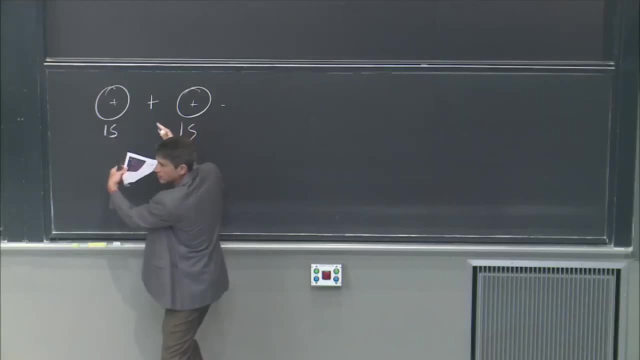 well, you can see, as I bring these close together, if they have the same sign, these are waves. So if the waves are both positive and I bring them together, they can constructively interfere. So as I bring them closer and closer, 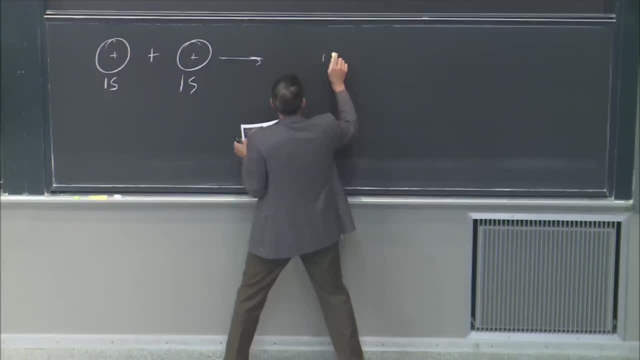 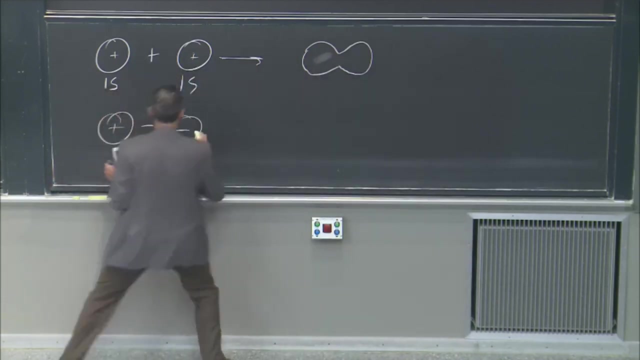 well, I might actually get the picture that I showed you. right, I might actually get something that looks like this: Okay, I might actually get something like this. Now, if I subtracted them, then, as I bring these orbitals closer together, 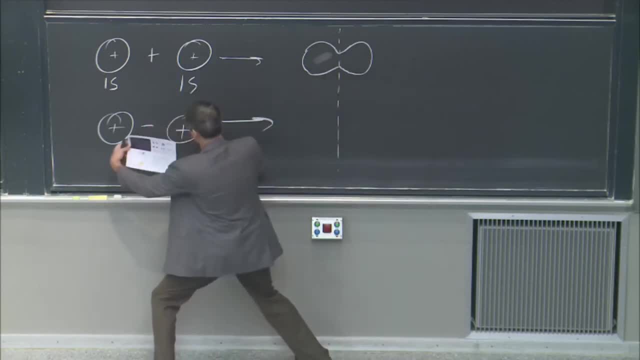 they're going to cancel each other. And you can see right here, if I bring these orbitals, by the way, which are coming from two different atoms, right, The whole point is we're talking about? we're talking about molecules, molecular. 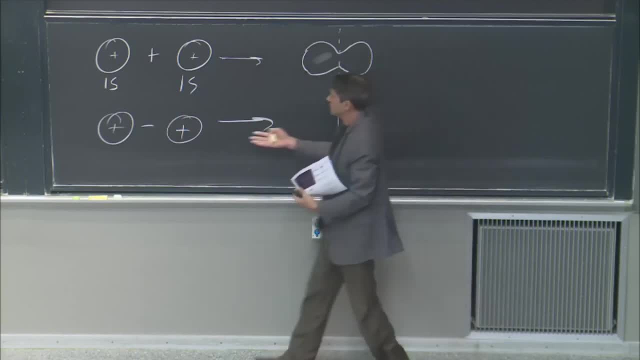 So if I bring them together now like this, but I'm subtracting these orbitals, then you can see that right at the interface, right between them, it's always zero, Because I've just subtracted the same amount. No matter how close they get, it's zero. 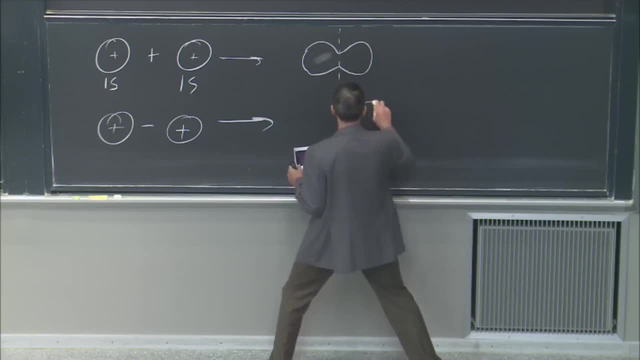 That's a node right, And, in fact, what you're going to get is something that looks like this: All right Now. so what I've done is I have, I have, I have added and subtracted the same AO. 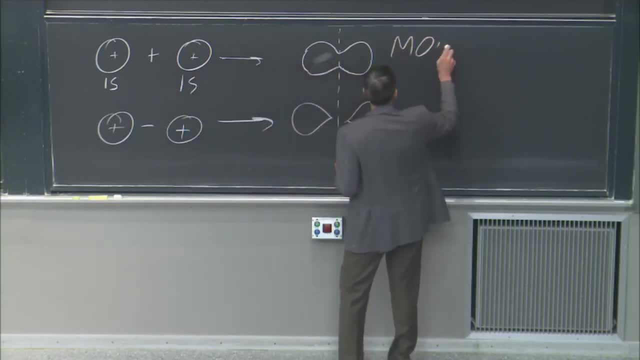 And I've created two MOs. So these are my MOs and these are my starting AOs. That's about the simplest thing you can do in MO theory. I'm using these as a basis. Now there's something very important, which is that this is: 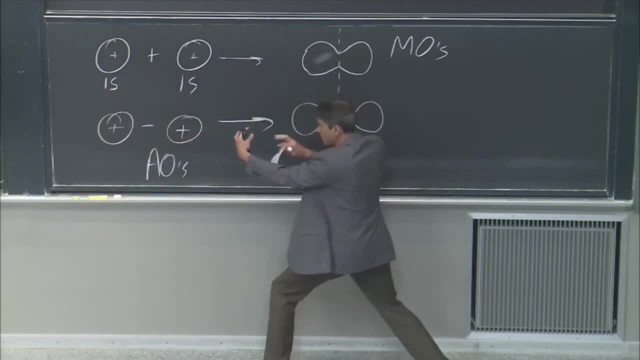 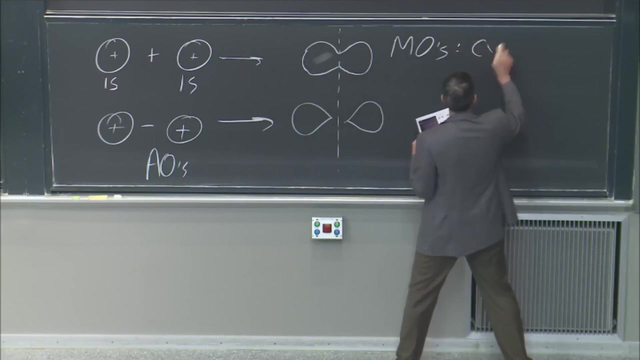 I kind of already alluded to this. These are two atoms coming together to make a bond. This is the bonding axis. This is the bonding axis. Okay, Now, if an orbital, if an MO is symmetric, okay, so if it has cylindrical, cylindrical symmetry, about that bonding axis. 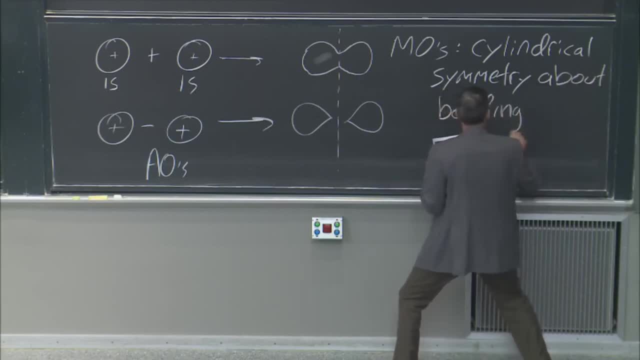 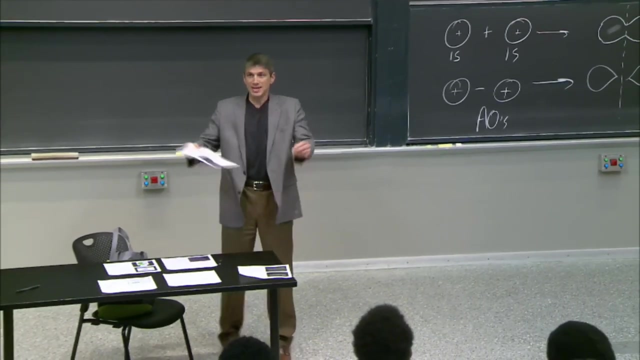 then it's called the sigma orbital. It's called the sigma orbital. That's the MO. Sigma is a notation, A sigma orbital is one that has symmetry around the inter nuclear axis, The two, ah ooh, We're coming to that very soon, because these are just the orbitals. 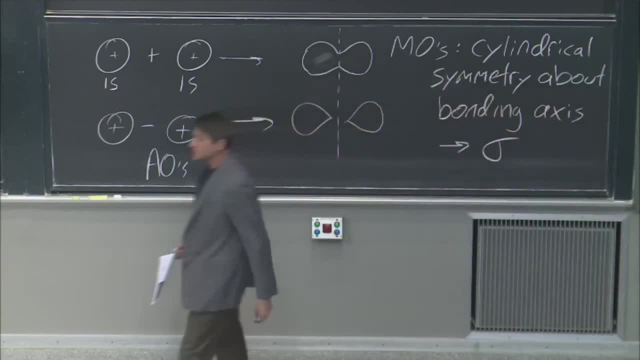 I got to do something with them. It's just like over here I made all these orbitals but then I had to fill them. Oh, that got me excited. But then, see, you can see right here When I add them up. when I add them up, there's charge in between. 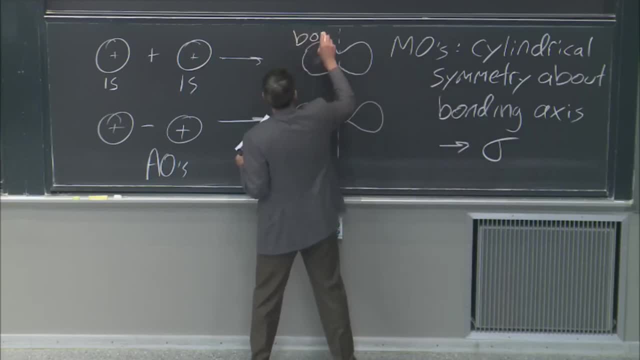 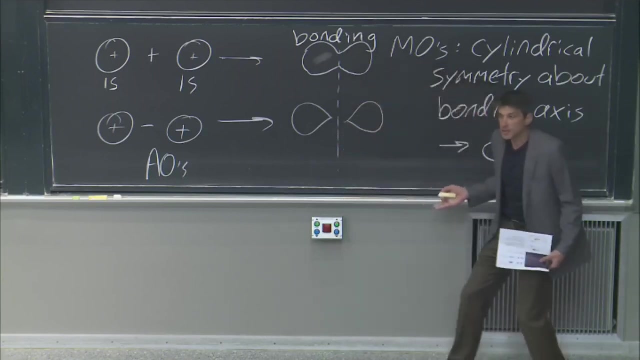 So this looks like it's going to have a bond- That's a bonding MO. but if I subtracted them, this doesn't look very happy in terms of like electrons being in between and the carrying and sharing principle of a covalent bond. 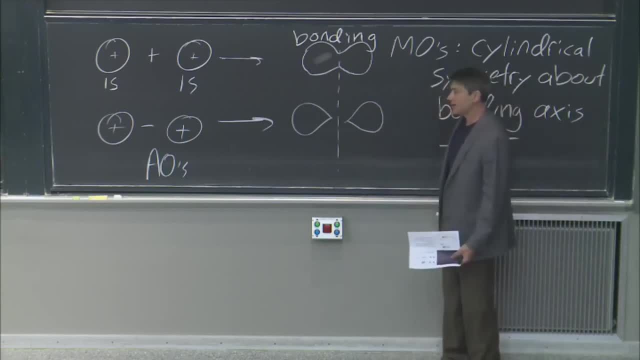 Okay. So if I were to put them together, this would be, you know, a bond. If I were to put an electron in this MO, it doesn't look bonding, In fact it looks anti-bonding. It's actually not quite non-bonding. 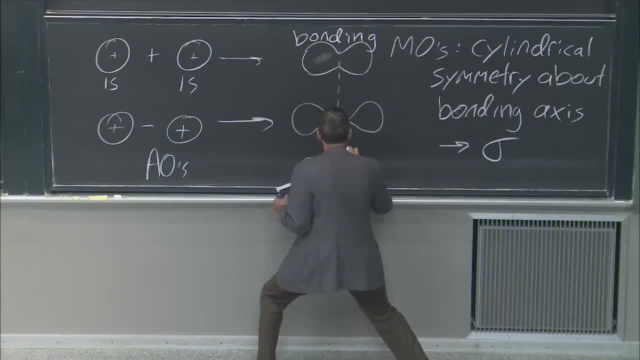 We'll get to that later. This would be anti-bonding. Why? Because there's not even a chance of electron density in between. That's your starting principle of the relationship Let's try to share. Oh, by the way, right halfway, no chance. 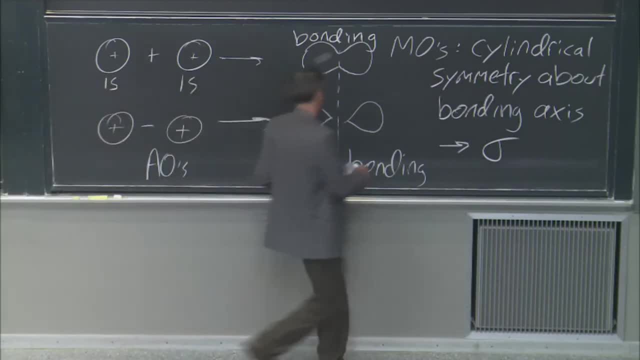 That's not a very good way to start And you can see why this is an anti-bonding: It's the opposite. You're actually pushing charge away from the bond if you're in this orbital, if you're an electron in that orbital. 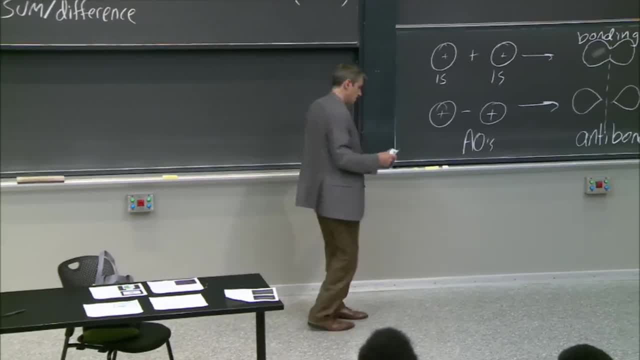 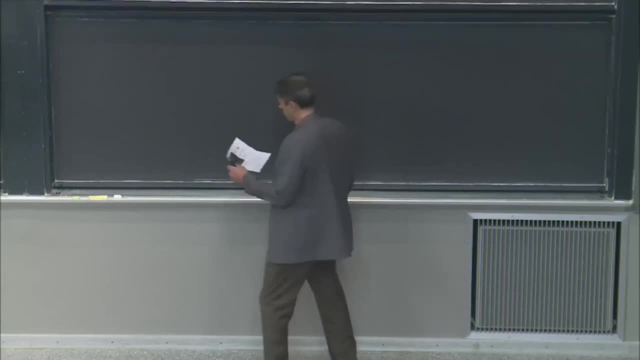 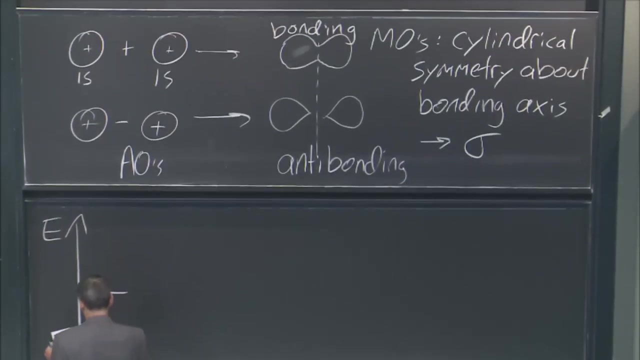 So that's an anti-bonding orbital. Now we get to the question: what do you do with these orbitals? Well, you make them. I made these with 1s, And the way that we typically draw this is: we go back to the same picture. 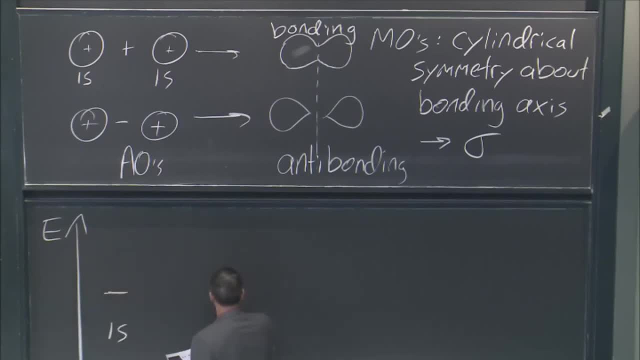 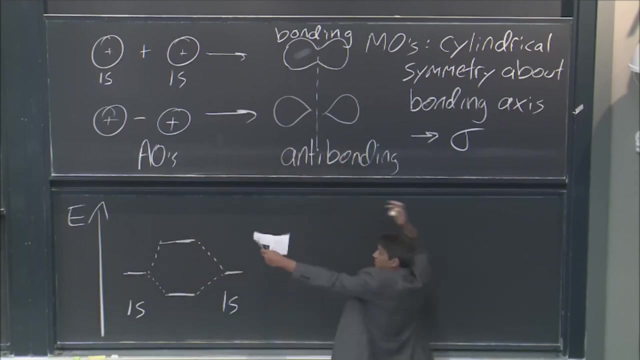 that we've been working with 1s here and 1s here And I brought those orbitals together And I formed one that lowered the energy of the system and another that actually raised the energy of the system, Because the electrons are repelling 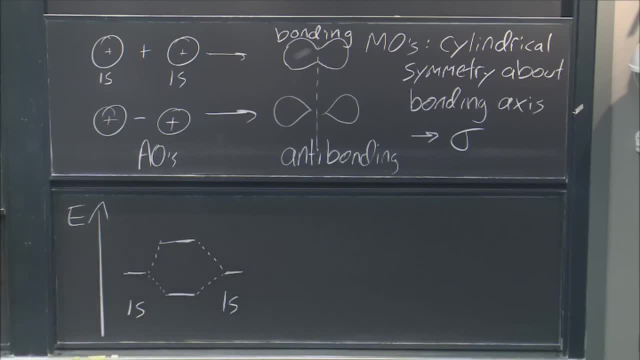 They're actually less bonding. They're anti-bonding Right. So these are my MOs, Those are my AOs, Right, AO, And now this is called a sigma orbital And the way we refer to the anti-bonding orbital. 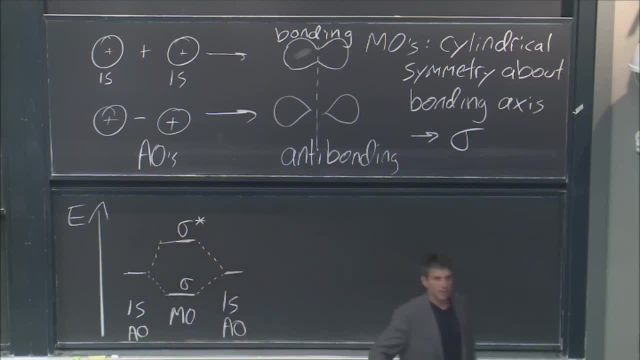 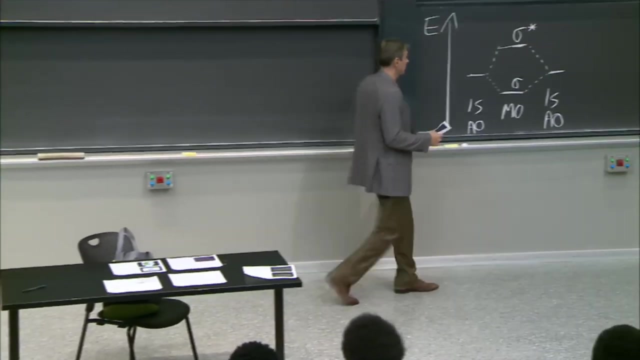 is with a little star. They're both sigma because they both satisfy that Right. They're both sigma because they both have symmetry around the inter-nuclear bonding axis. But now see, OK, so that's good, But now let's fill them. 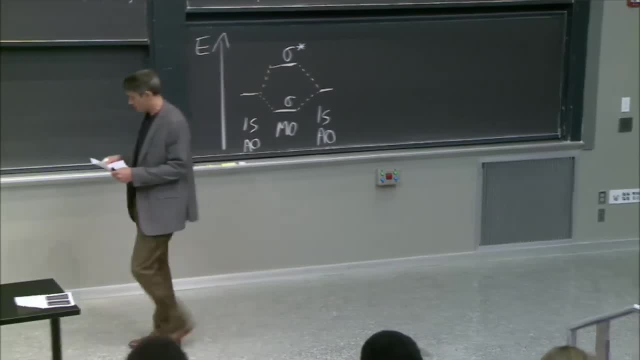 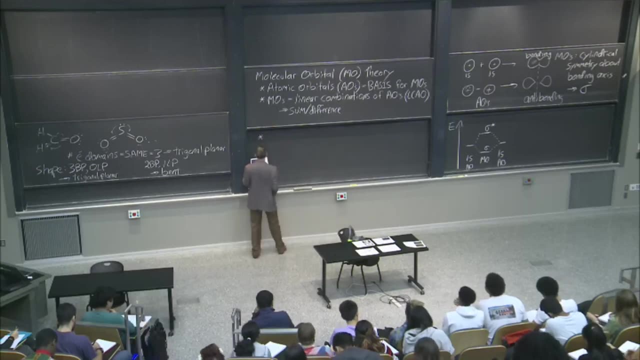 Let's fill them Right, Because now Let's write down the rules and then we'll fill them for some examples. OK, So I'm going to keep going on my MO theory list Right. As you can see, when I do it this way, 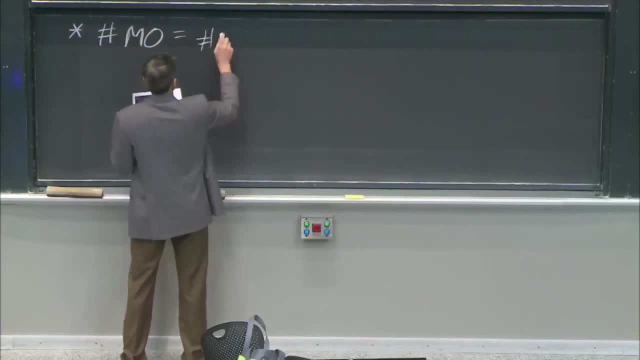 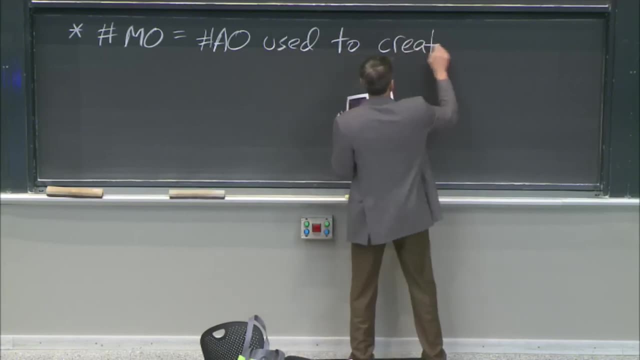 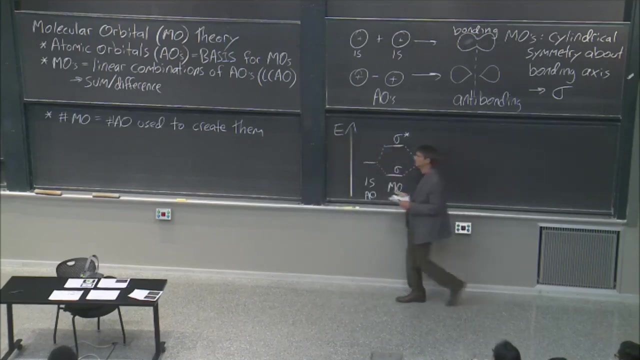 the number of MOs equals the number of AOs used to create them. So that's one thing that we can see right away. Right, I used two AOs. I added and subtracted them. I got two MOs. Good, 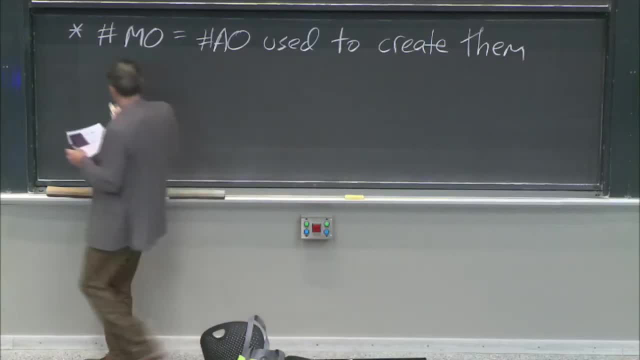 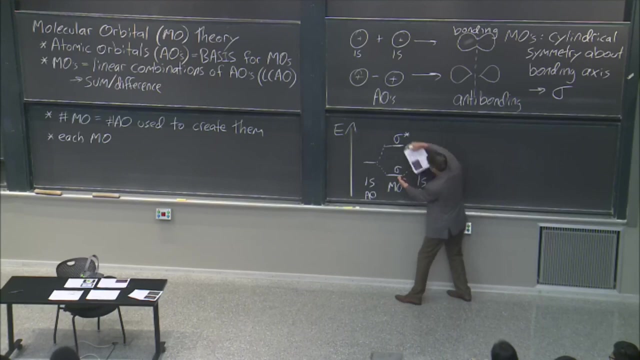 All right. Another thing is each MO will be just like an AO, Right? It makes a lot of sense. I had room for two electrons here. I had room for two electrons here. I got to have room for four, Two here, two here. 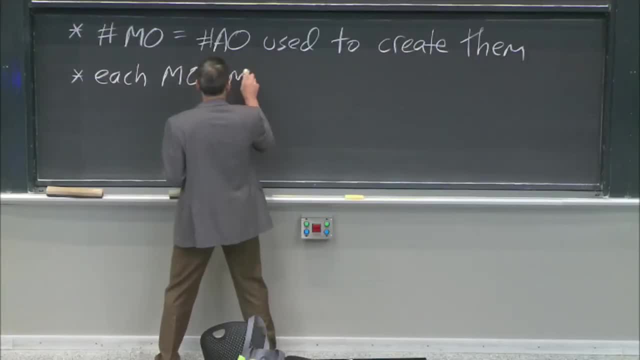 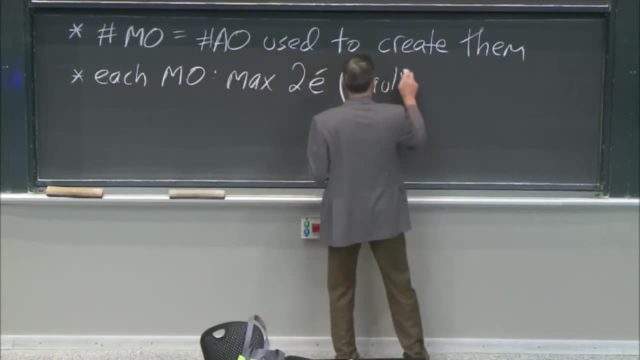 Right. So each MO has a max of two electrons and they must obey. They must obey Pauli, just like in AOs, They must obey Pauli. You can't mess with quantum mechanics. Uh-uh, Still electrons, They're still quantum mechanical. 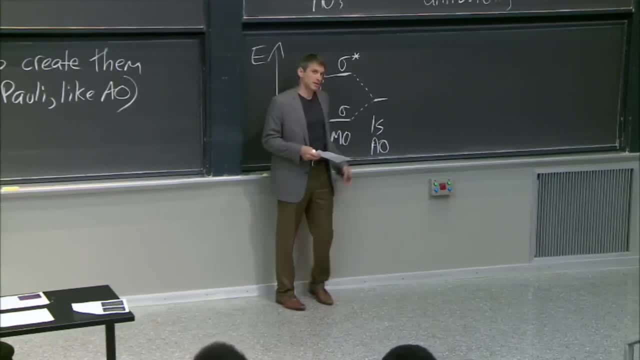 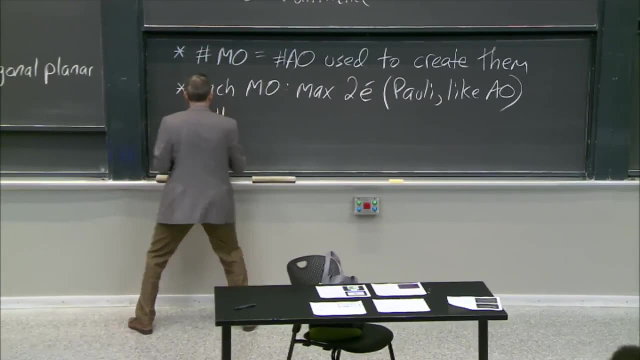 Right, You're just making their wave function more sophisticated, But they still have to follow the Schrodinger equation and the principles of quantum mechanics, And so, finally, what we're going to do is we're going to fill them. So we're going to fill the MOs. 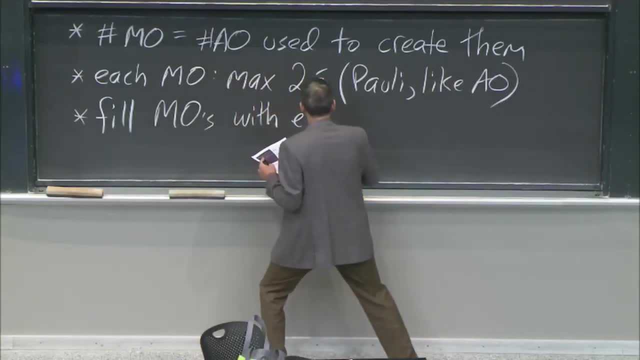 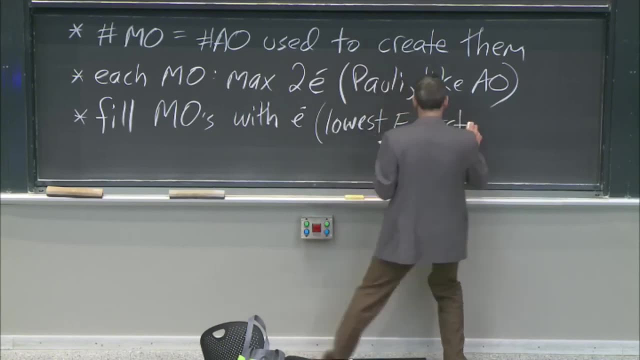 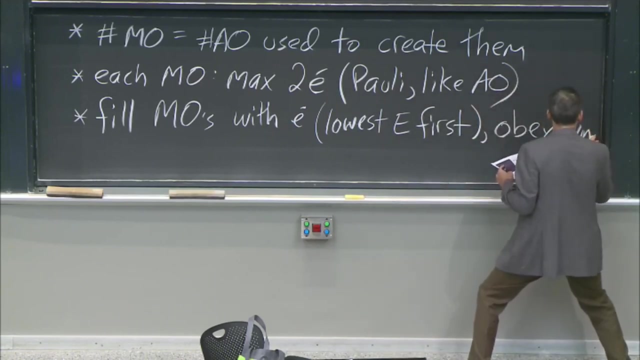 With electrons, With electrons Starting with the lowest energy, just like we did for atoms. Lowest energy first. OK, And one more thing: just like we did with atoms is we're going to obey Hund Ah Hund, Hund's rule, which tells you about how. 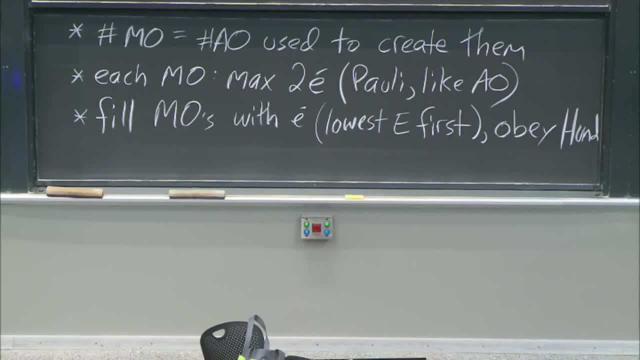 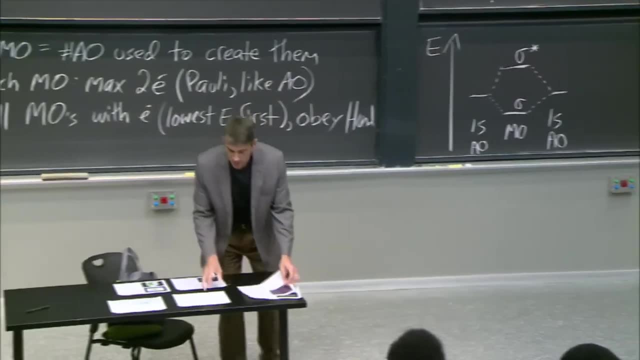 to fill degenerate orbitals. Well, we're going to have degenerate orbitals here too. We don't yet, but we will, So we're going to fill them. So let's fill them For the very simplest cases. 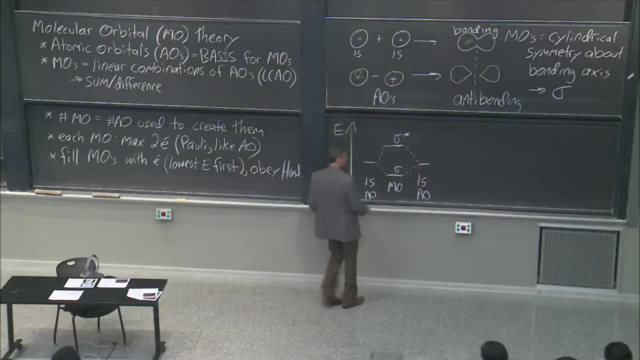 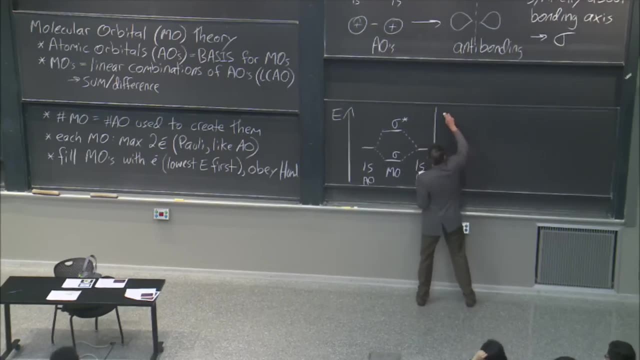 OK, so we'll do some cases together And we'll see how that goes right. So what I'm going to do is four cases, just so we can compare. So first we're going to do H2 plus OK, that's the first one. 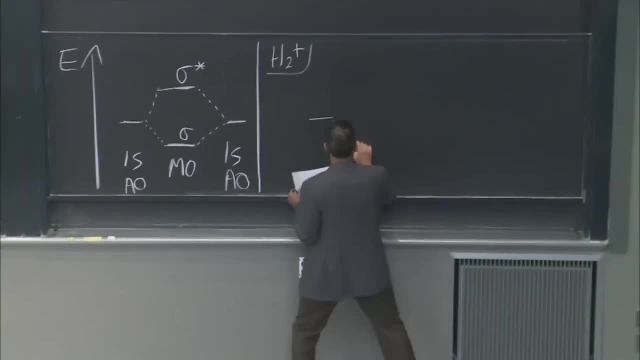 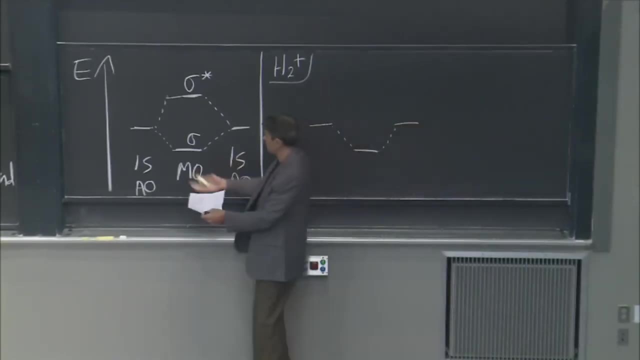 And here what we have is the same graph, But now over here, I actually can label it. now, This was just an orbital, But now Gesundheit. Now I say, OK, Well, this is the H. This would be like H and H plus. 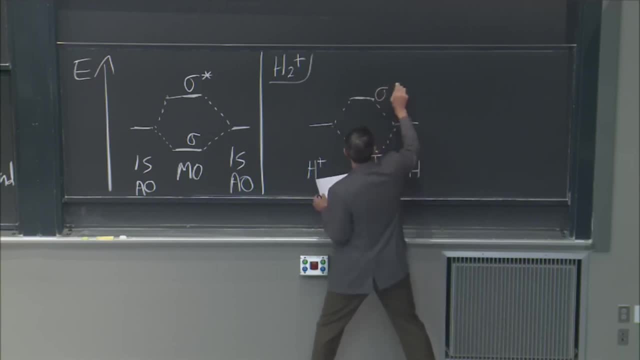 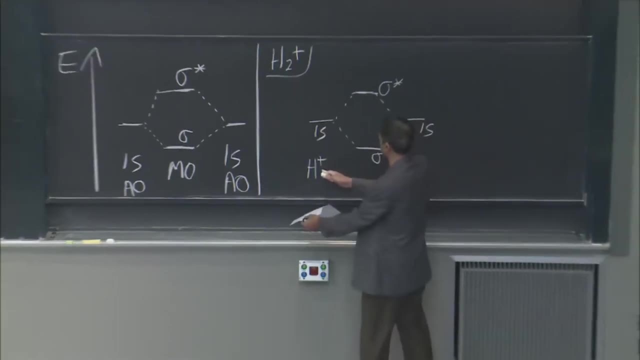 OK, these are my MOs: Sigma, sigma, star, 1s, 1s, Oh boy. But if that's H and that's H plus and they're coming together to make H2 plus, that's what's in the middle there. 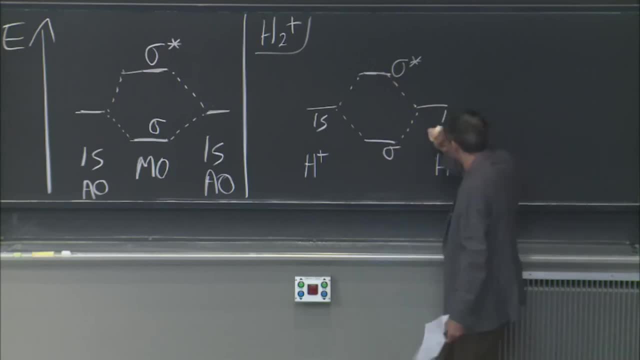 That's the molecule. Well then, I also can now fill in the starting AOs. So let's do that, And that's it, Because this one lost. Somebody had to lose an electron to start with. We'll just represent. So now, when these come together, you fill. 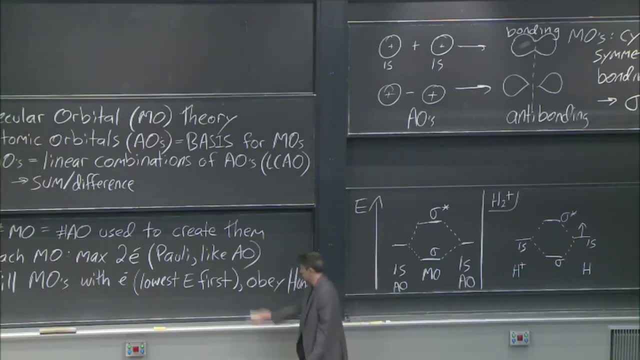 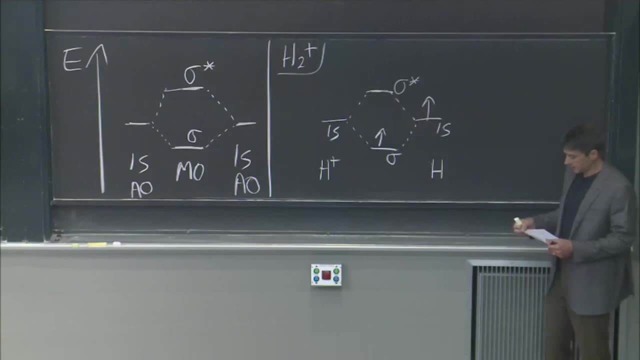 You obey the Pauli exclusion. You fill from the lowest energy first. You say, well, I only got one electron. There it is, That's my MO diagram, populated by electrons. OK, now there's a principle that comes out of this. 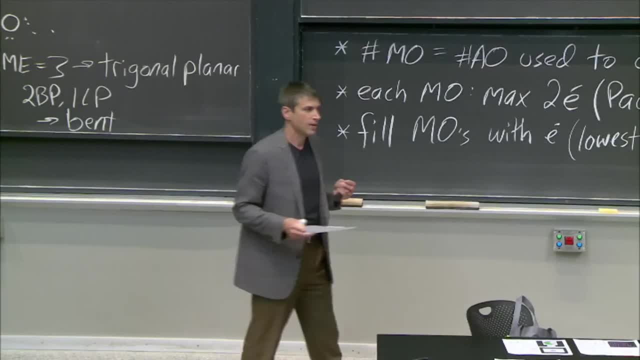 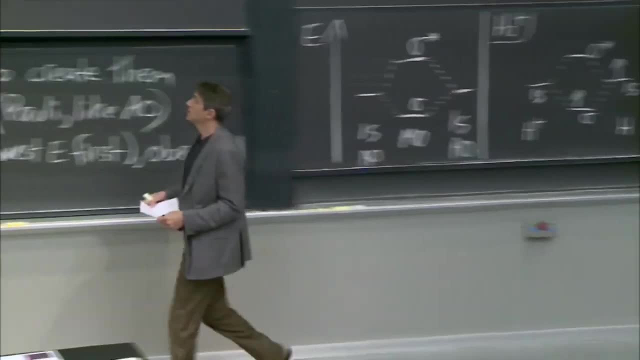 There's a way of understanding bond strength. now, There's a way of understanding bond strength And that is a very important concept. Let's put it here in our list. Let's put it here in our list, OK, And it's a concept called bond order. 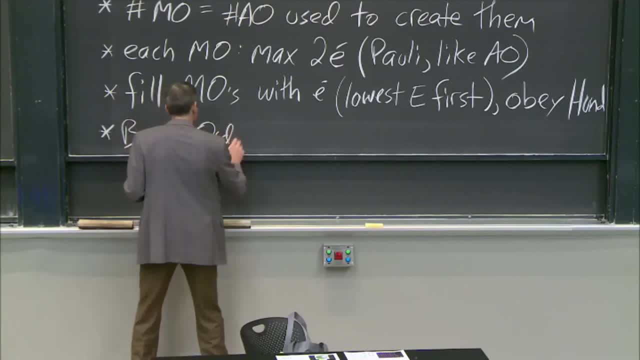 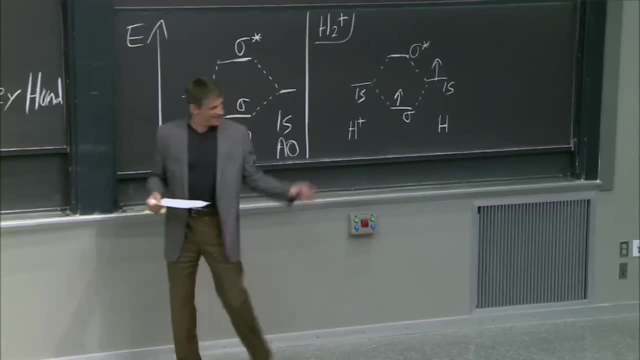 Bond order. Now this one. I really want to write BO, but I don't know if that's a good idea, So I'm going to keep. I got lower than that one, OK, And that's going to equal. There's a definition for this. 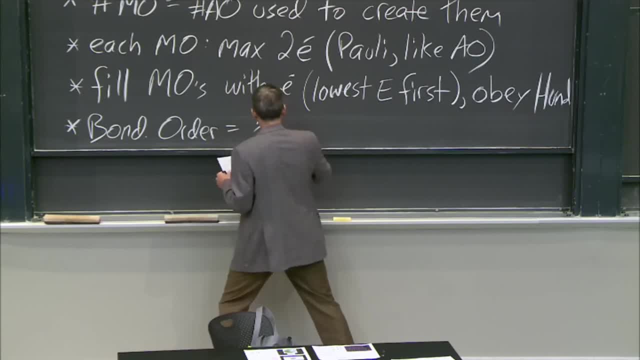 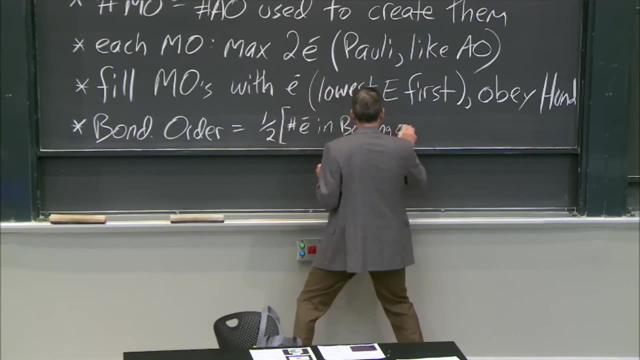 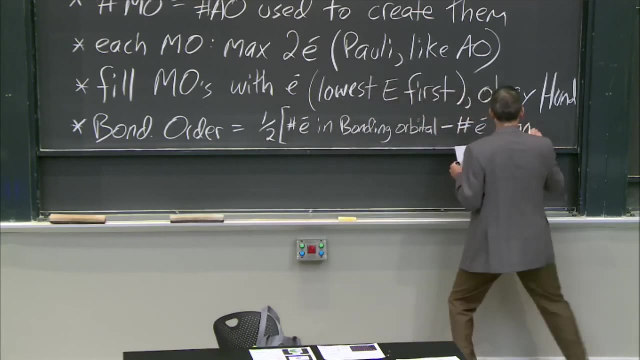 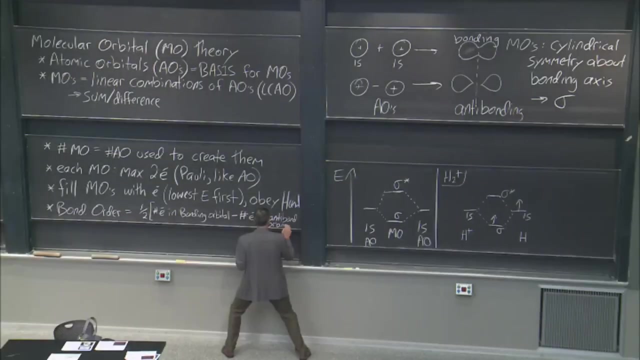 It's going to equal 1 half of The number of electrons in a bonding orbital in a bonding orbital minus the number of electrons in an antibonding orbital. Sorry, this is a little bit small here, But we'll do a bunch of them so you can see what this means. 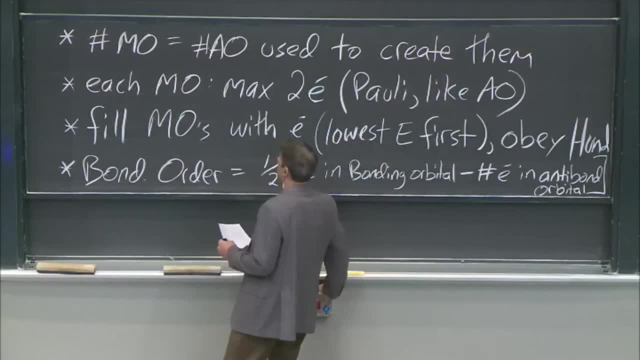 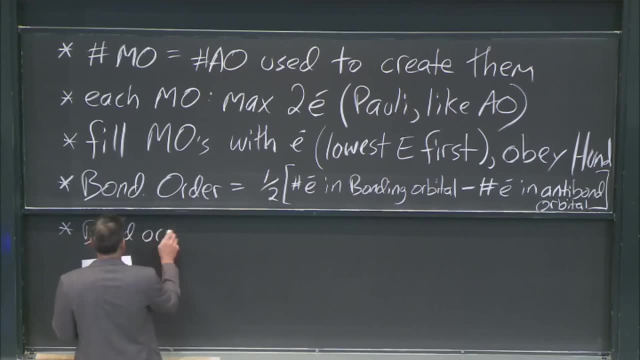 Right. So the bond order is important because the bond order of a molecule, Right. So the bond order, bond order if it's higher. if it's higher, then stronger bond And it has to be greater, And it has to be greater than 0 for stability. 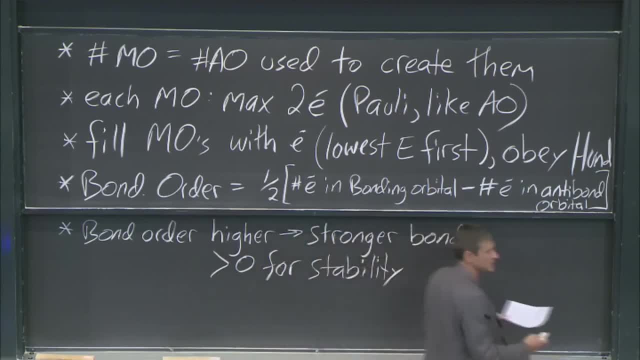 Let's see how that works, And I mean we'll see this intuitively as well as we fill these in. Let's see how this goes up. So if I count the bond order here, oh, I'm going to do it. 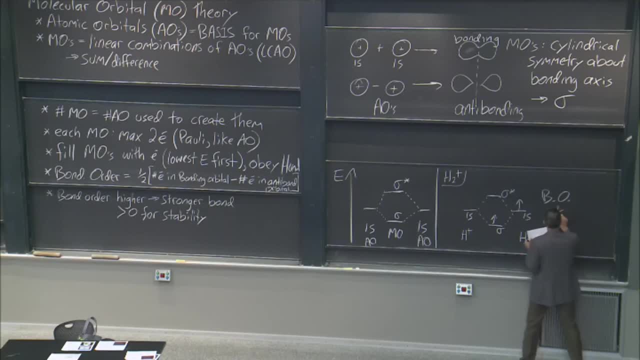 I don't feel like writing it out. The BO on this one is 1 half times 1 minus 0, which equals 1 half. OK, good, It's 1 half. Well, it's greater than 0.. So right away, I know that the H2 plus molecule. 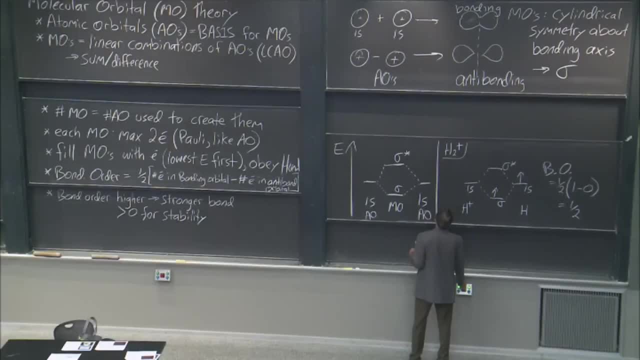 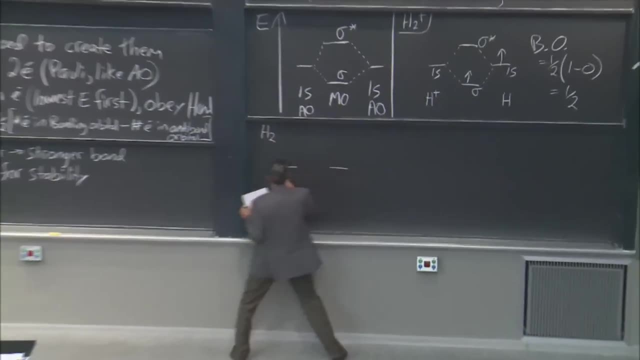 is probably stable. That's good, But let's go to some more examples now. Let's do a few more. All right, Now we're going to work our way to H2.. In this case, energy is always going up in these diagrams. 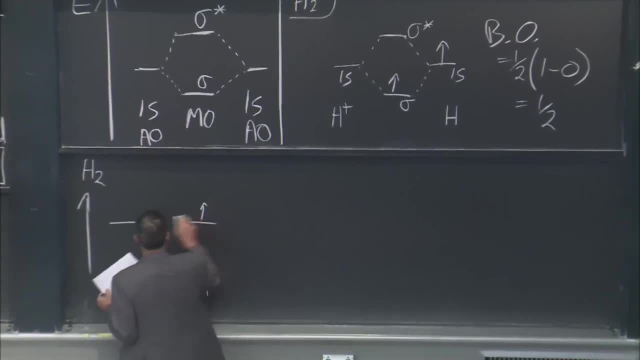 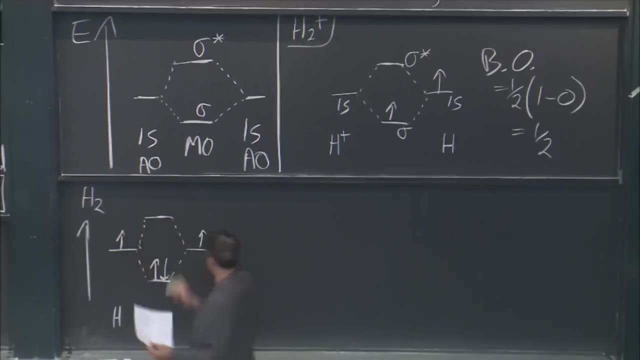 Now, each of these H atoms is bringing in an electron. There's no charge to the system. And so now, different quantum numbers, Pauli. different quantum numbers, but same sigma, right. And so now that's the H2.. Now the bond order here is equal to 1.. 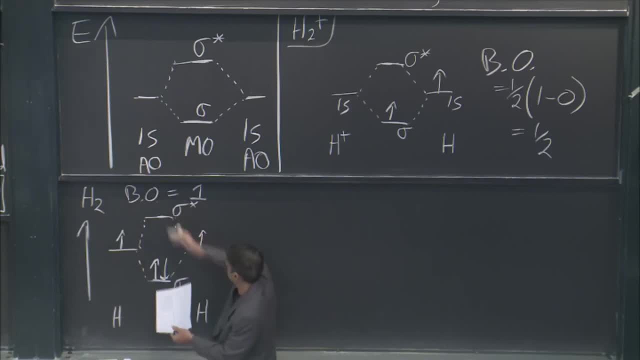 Right, I didn't have any electrons in an antibonding orbital, But you know what's coming. I'm going to do He2 plus next, And here what you're going to see is OK, if I were. let's just put it here for comparison in real time. 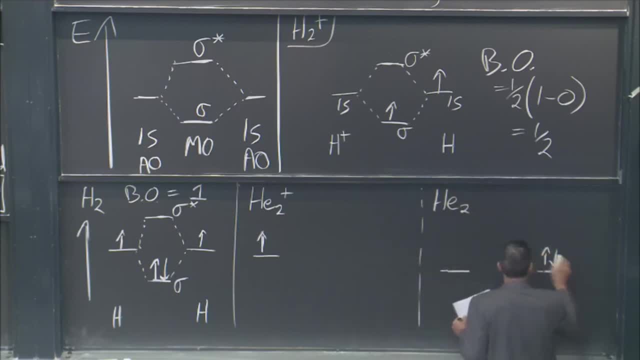 If I were He2, each of these would be the AO occupation of an He atom right, And since I'm He2 plus, one of them is missing an electron. So this is what you're going to see. These are both He atoms, still, but one of them. 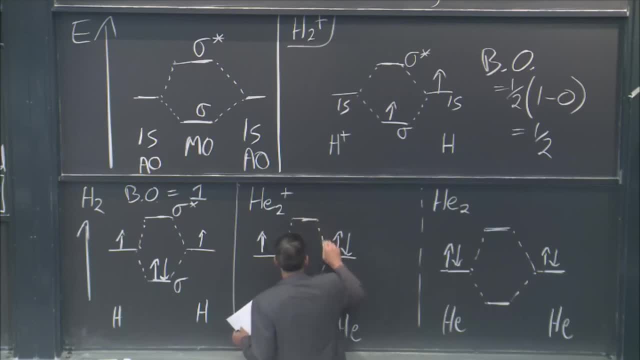 is plus in this picture. But see now, OK, I've got three electrons, They're going to go here. I've got to put one up here. I have to because I had three. I've got to keep on filling, just like in an atom. 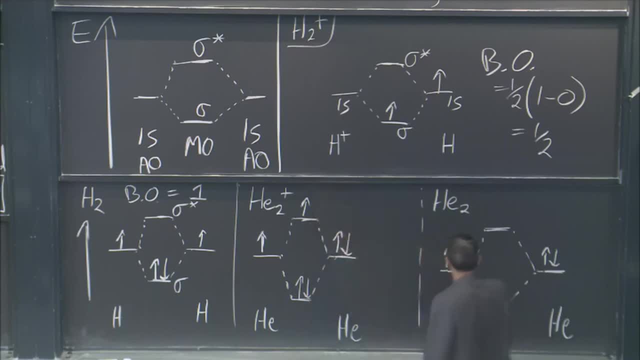 But now I'm filling bonding and antibonding orbitals, All right, And here I've got this and two up there. So if you look at the bond order, here the bond order is still positive. Here the bond order is 0.. 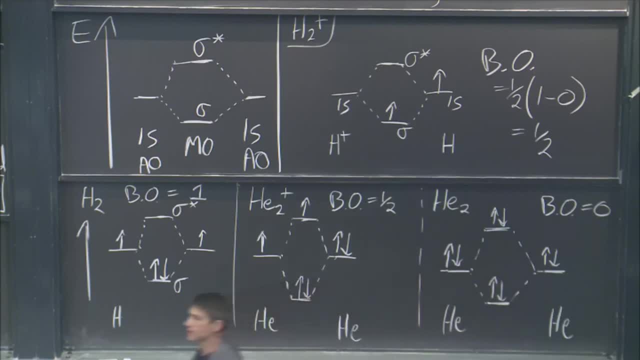 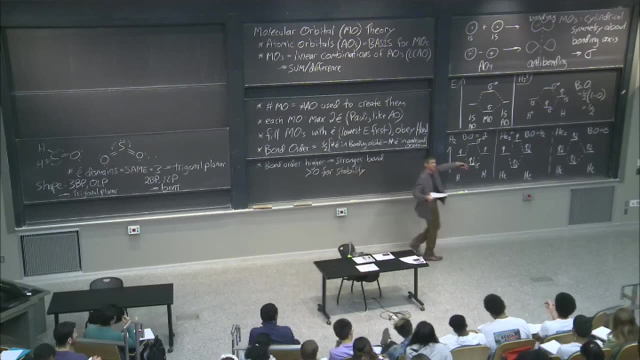 And in fact that's why He2 is not a stable molecule, Because you're putting just as much charge on this thing that wants to bond it as you are on this thing that doesn't want to bond it And at the end of the day, it leads. 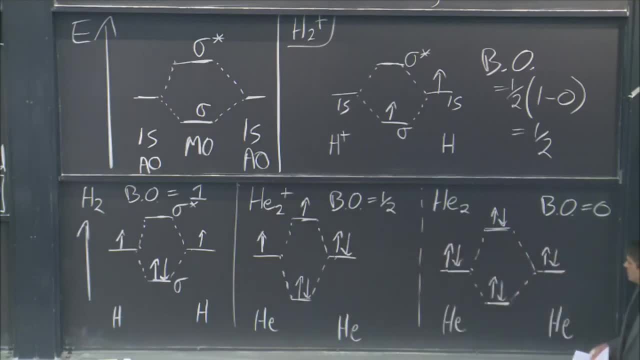 to a molecule that is not stable. So that would be He2.. But He2 plus has a bond order. that's similar. right, That's similar. Did I get something wrong? He2 plus 1 half. OK, Now, because this weakened it, right. 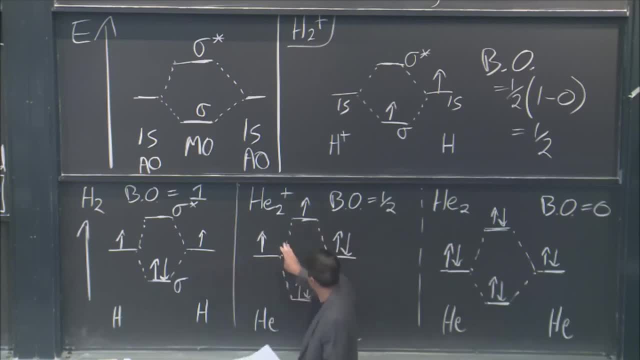 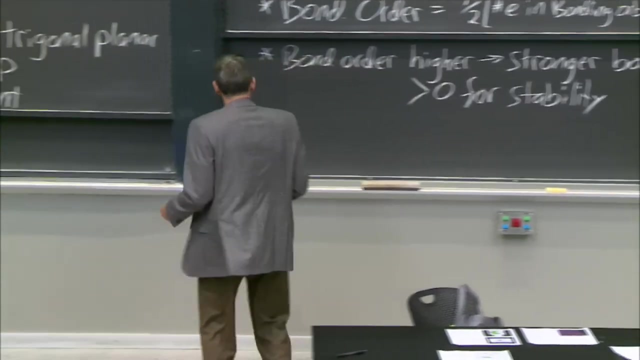 This weakened the molecule compared to this, because now I added charge to an antibonding orbital, So you would expect from the bond order that this one is more stable than this, And in fact this is what you find. The H2 molecule has a stronger bonding energy. 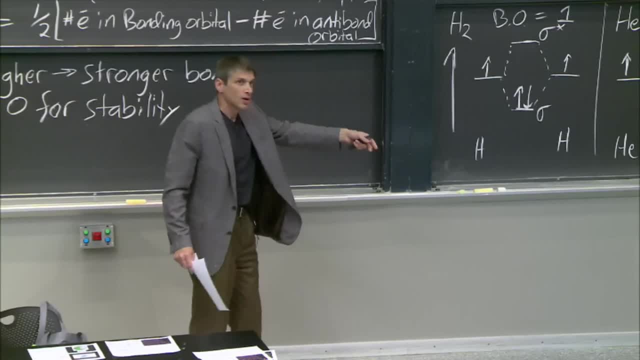 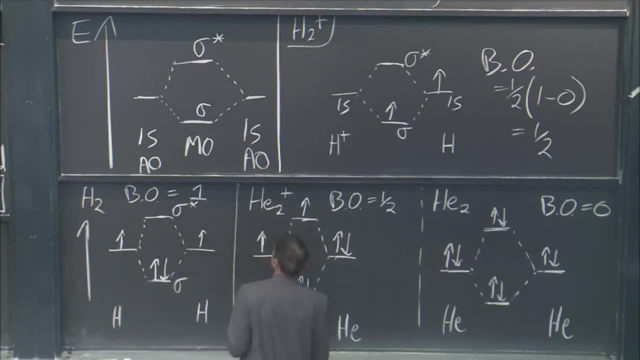 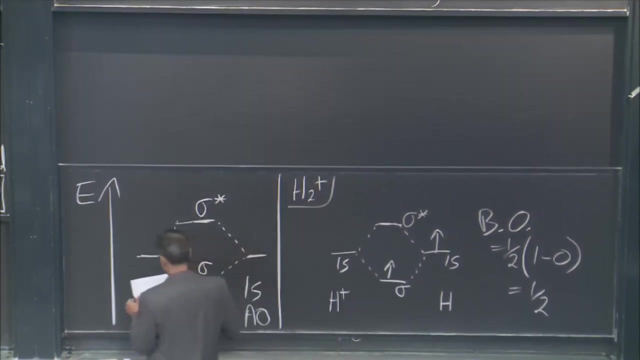 Now we can write the molecular orbital configurations just like we did with the atomic orbital configurations. OK, And so like for here. ah right, So for this case I'm going to write it up top, if I can fit. So here. 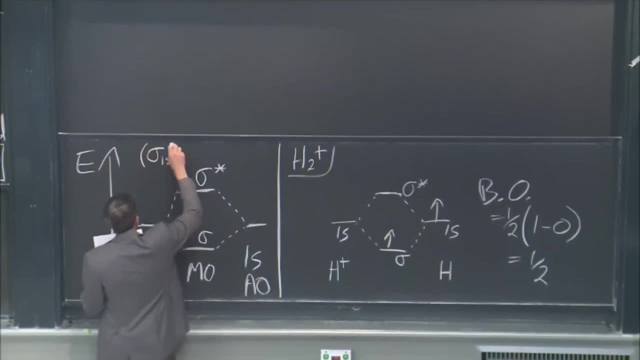 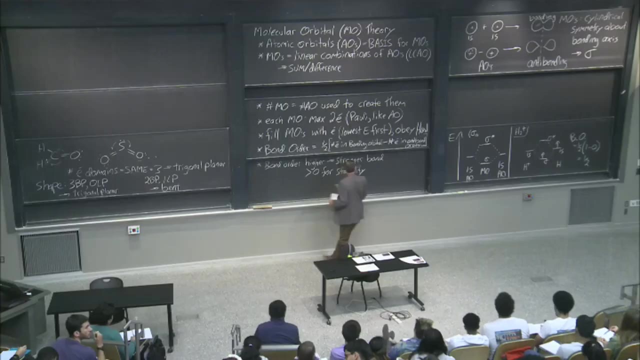 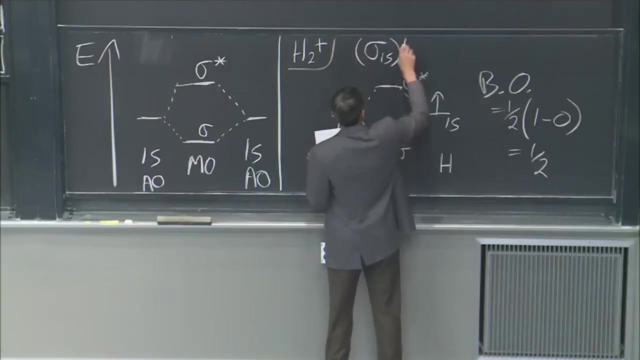 Here we would have sigma 1s and we're populating it with ah. That's not my example. This is my example. Sigma 1s is the orbital and we're populating it with one electron right. So that's how we would write that. 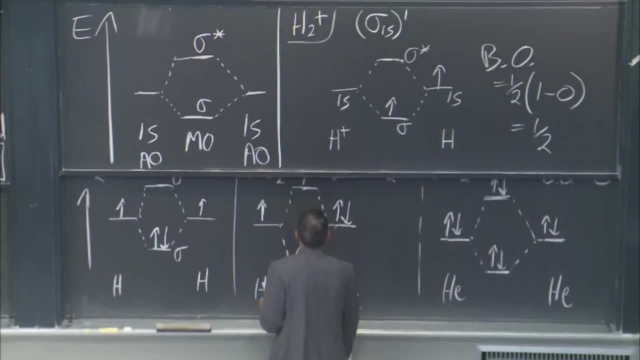 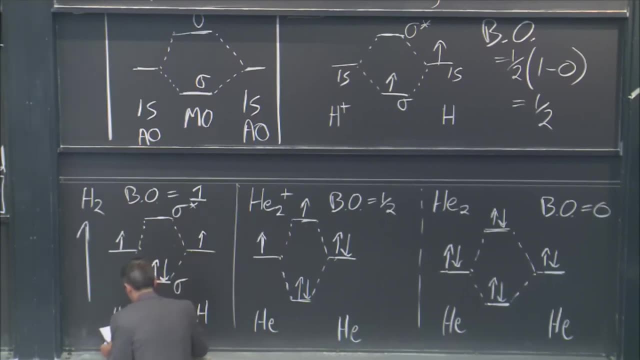 Now, if we go to the next examples we would have. this one is This molecule? you would write as sigma 1s2.. So this would be sigma 1s2.. And oh, now I've got sigma 1s2.. 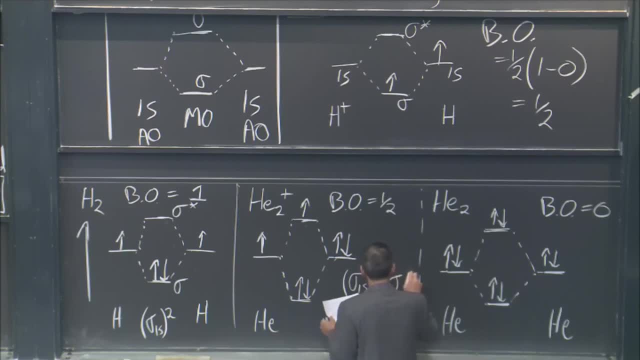 Oh, this is getting interesting because now it's sigma star 1s1.. Everybody see that I populate and this is just like SPD. But now I'm just filling those MOs up and I'm showing you what the molecular configuration is. 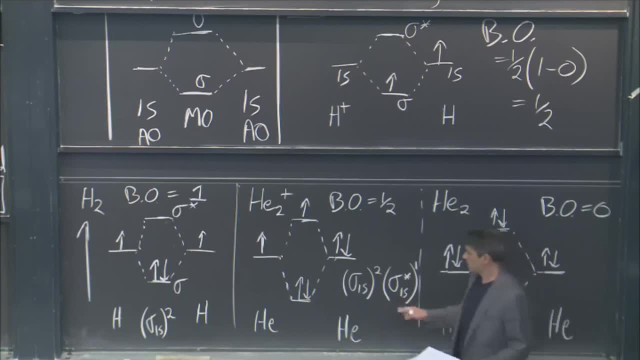 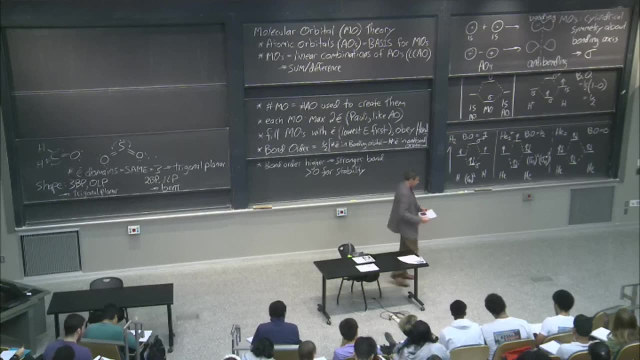 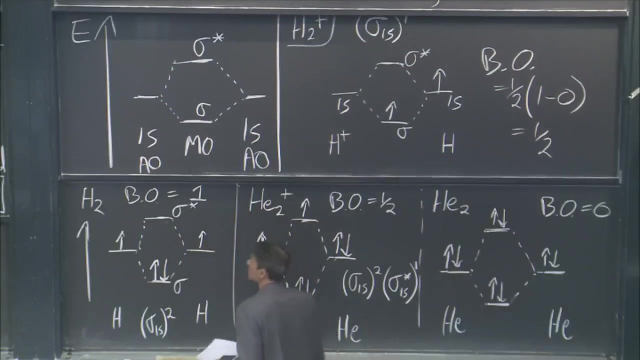 with those molecular orbital names: Sigma 1s, sigma 1s, star. OK, good, Now we can keep going. We could do this all day. Actually we kind of will, But we're going to move on, don't worry, from sigma. 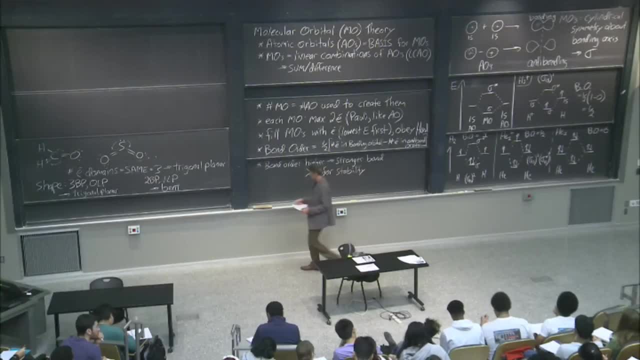 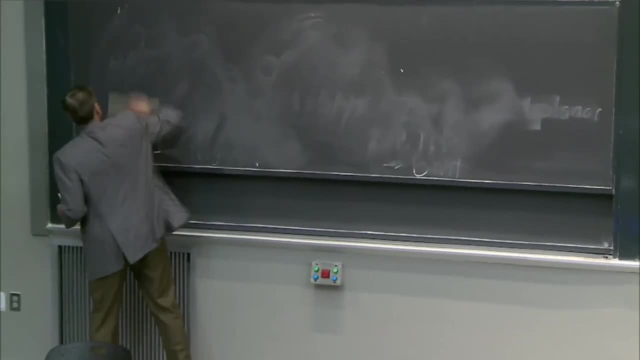 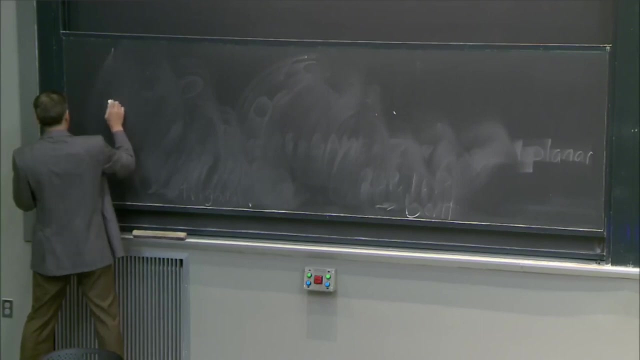 Let's see, Let me go over here. There's another concept that I want you to know about: MO theory. So If you know, so, if I kept going, I could have, for example, let's do lithium, OK. so now lithium 1s, oh 2s. 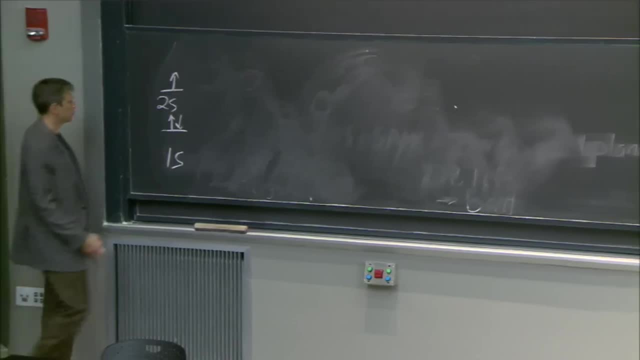 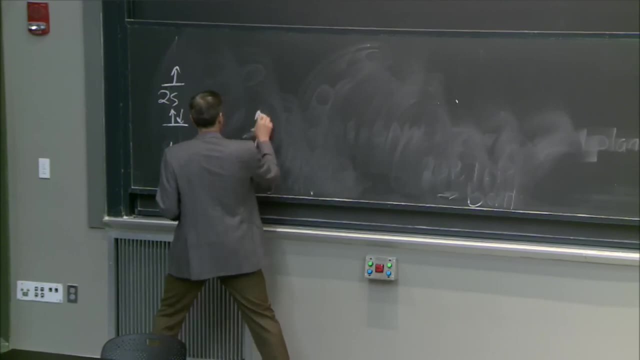 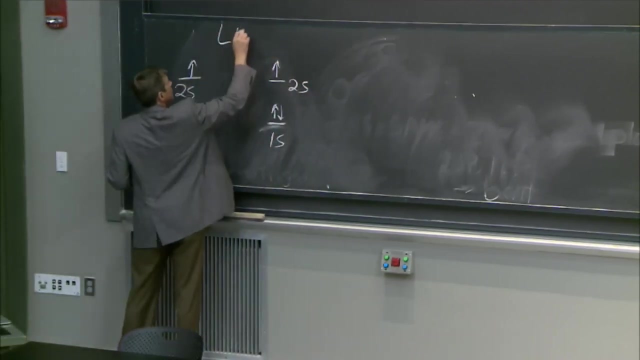 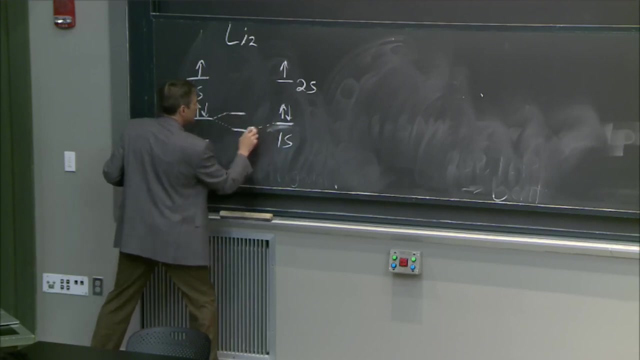 Lithium brings this. What does it bring? It brings three electrons, And over here 1s and 2s- Three electrons. So this would be the lithium dimer. But I want to make an important point. When you would draw this one, here's how I would draw it. 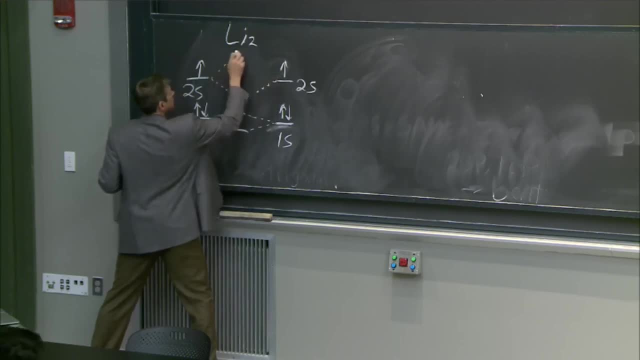 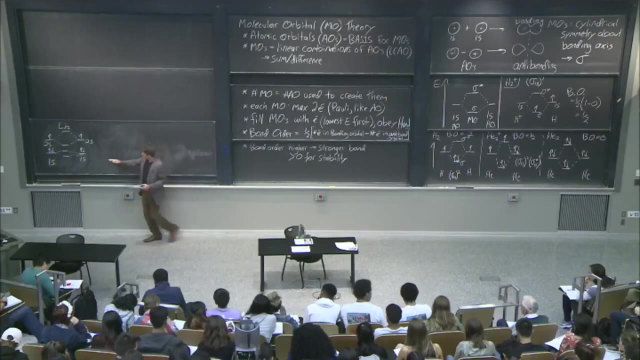 Whereas when I would draw this one, I would draw it like this: OK, Now those are supposed to be the same spacing. I'll tell you in a second Notice that the distance here between the bonding and anti-bonding orbital is larger than it is here. 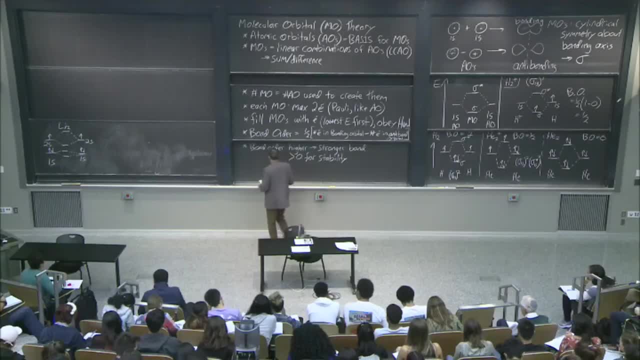 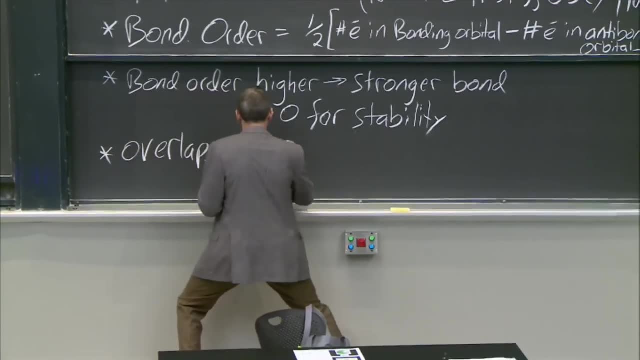 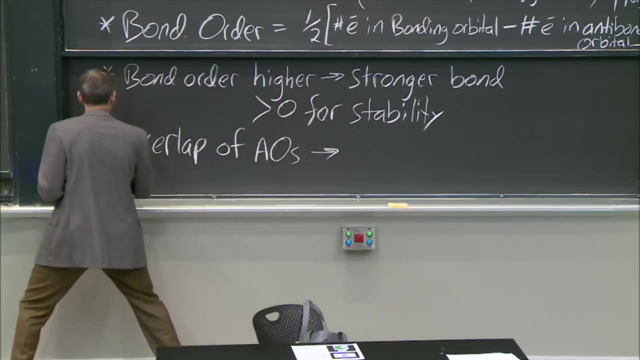 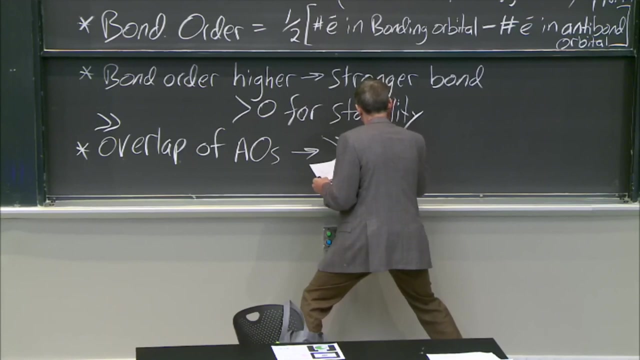 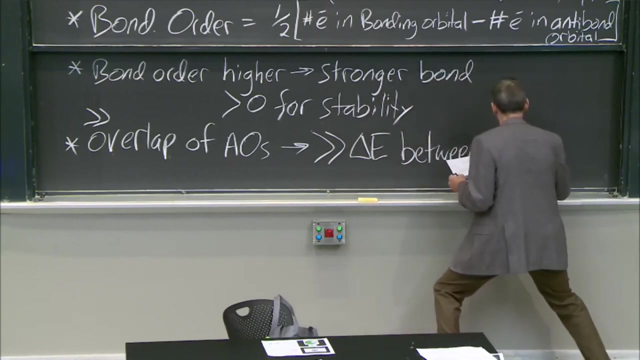 The reason is because it's related to the overlap. So there's another point, which is that the overlap of AOs is related. So the greater the overlap of AOs, the greater the change in energy. So that's the difference between bonding and anti-bonding. 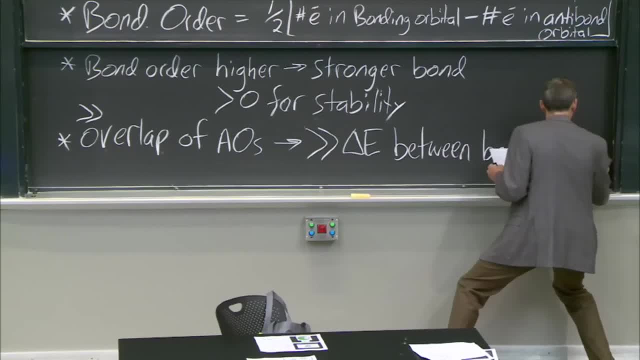 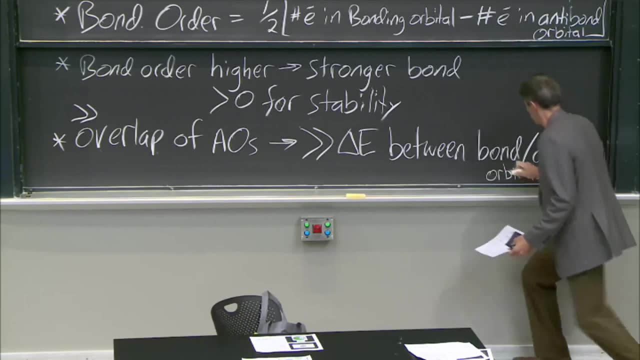 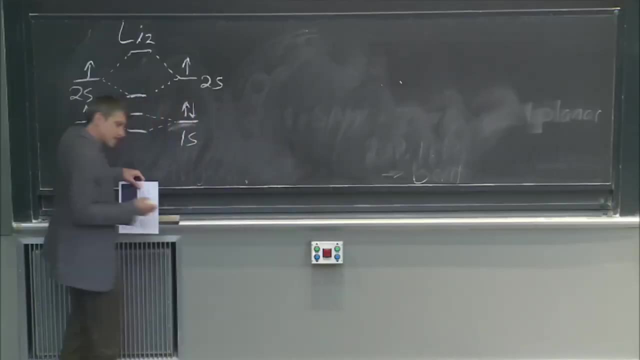 orbitals Between bonding and anti-bonding orbitals. And let's be clear, those are molecular. Well see, you can see like if I'm lithium those 1s's aren't going to overlap too much. 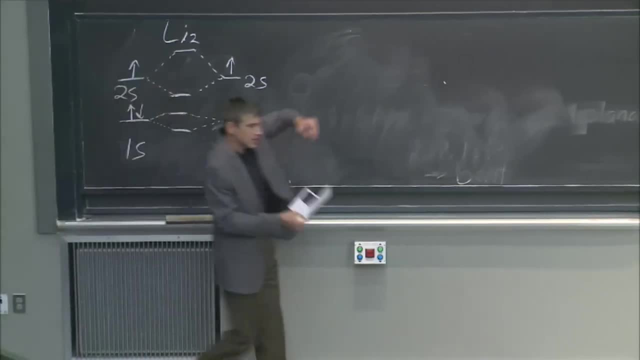 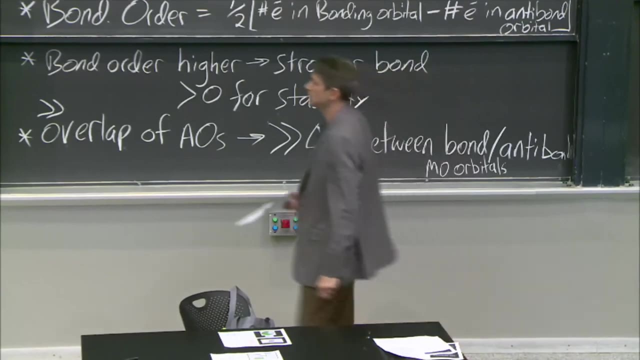 Right. They're kind of close to the core, So you do get MOs there, But the MO, the difference that you watch. these electrons are near in energy and overlapping, So the 2s can overlap a lot more OK. 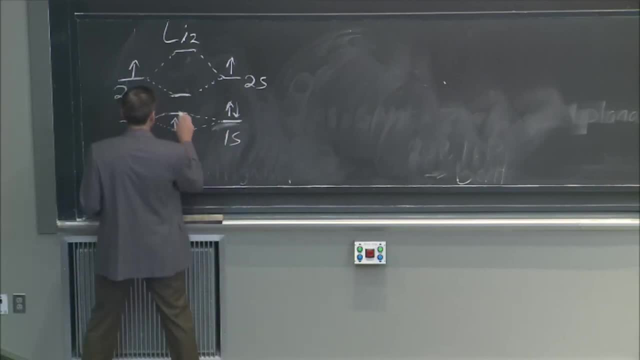 Now, if I were to fill this up, we would get something like this: It's all these sigma 1s's, Oh, sigma 1s, What do you think? these are called Sigma 2s, Sigma 2s? 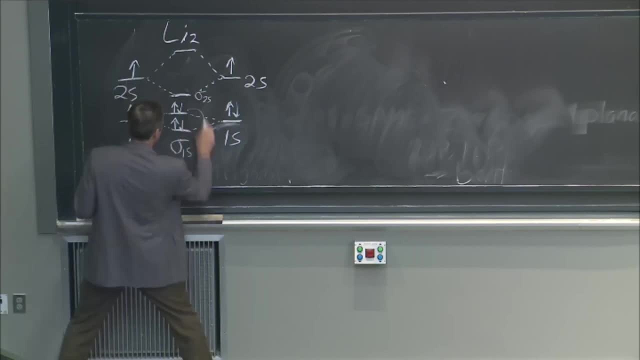 Sigma 2s And this. OK, this is getting a little bit. I'm going to draw this out here. That's the sigma 1s star, right, And this would be the sigma 2s star. Well, what am I going to occupy? 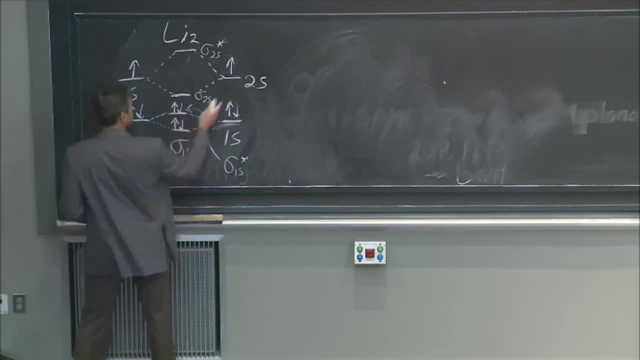 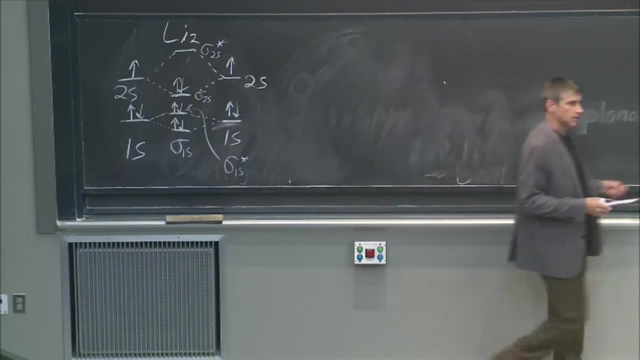 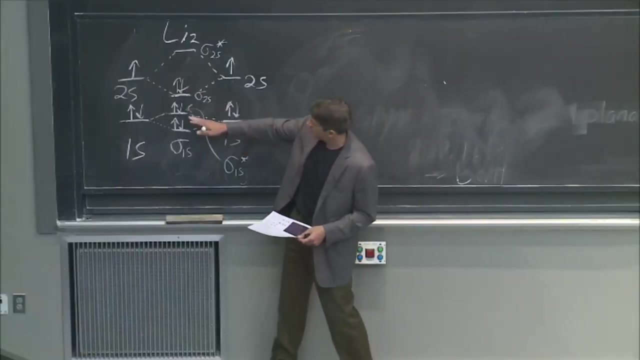 Well, how many electrons do I have to pour into the molecular orbitals? Mm, mm, mm, mm. Lithium. lithium 2 is stable because its bond order is: you see bond order: number of electrons in bonding orbitals. 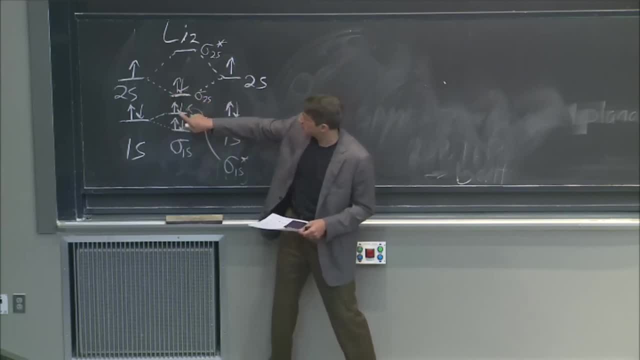 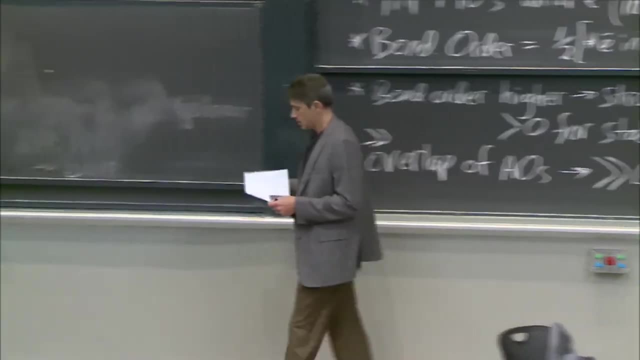 1,, 2,, 3, 4, minus number of electrons in anti-bonding order, minus 1, 2, divided by 2.. So the lithium dimer bonding order is 1, right, And then you can go on and you can say well. 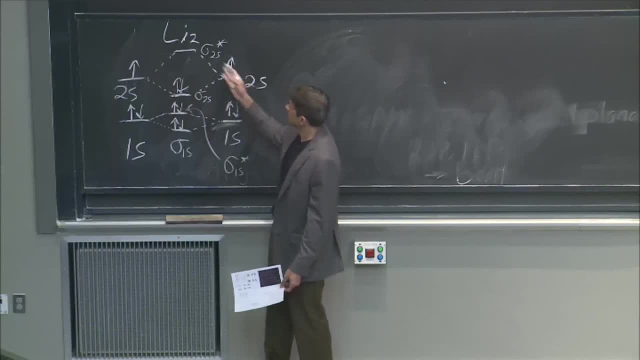 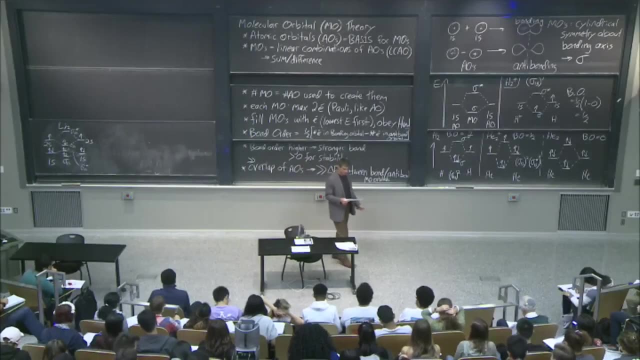 if I had beryllium, I'd have another electron here and here And I'd fill those anti-bonding orbitals up again, like in the He2 dimer, And I would have again an unstable molecule, which is in fact true. 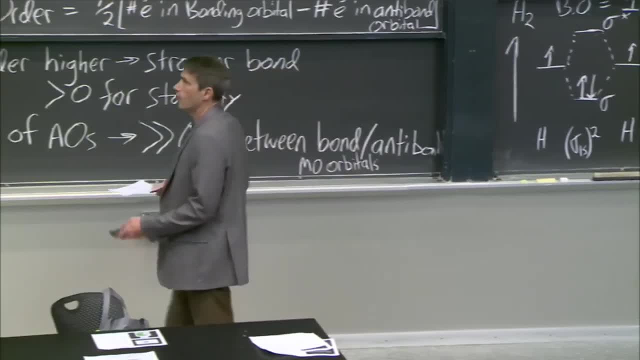 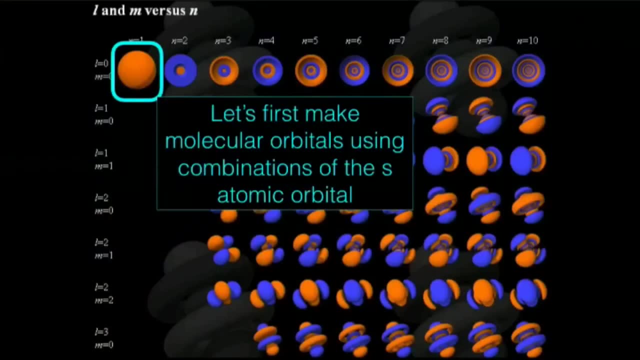 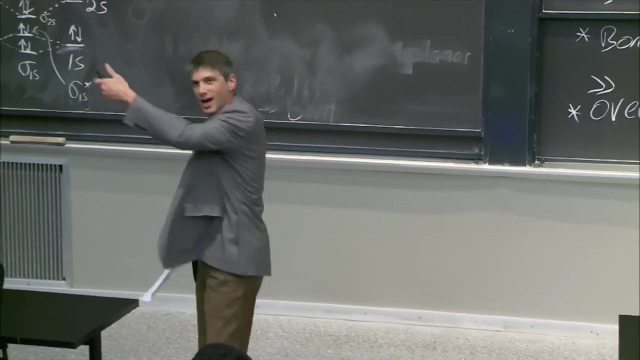 OK, This is sort of the simplest way you can think about molecular orbital theory, because it's the simplest orbital. But you can go, you can spend the whole night And it is a Friday. What else do you have? This is what you do on a Friday. 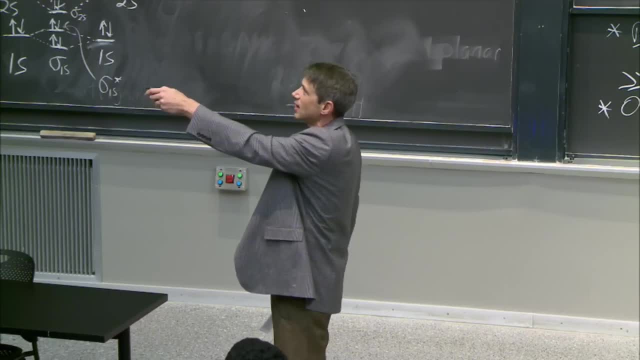 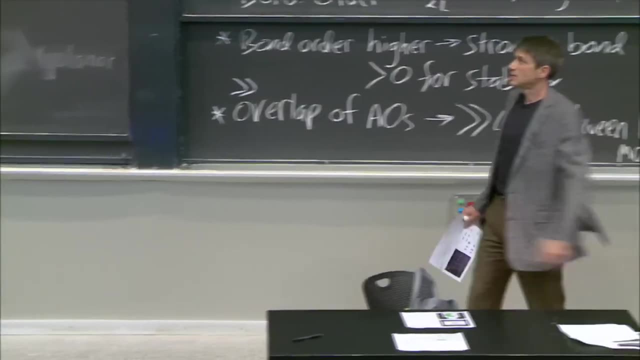 After I watch Dr Quantum, I'm going to just add every single one of these. with every single one, It's finite. It's not going to take forever, Let's just do p. So OK, Now with p orbitals, there's something. 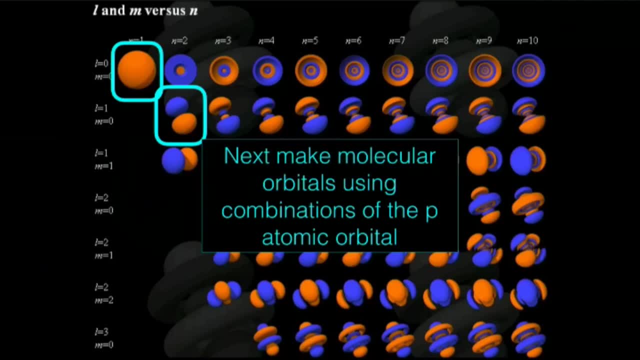 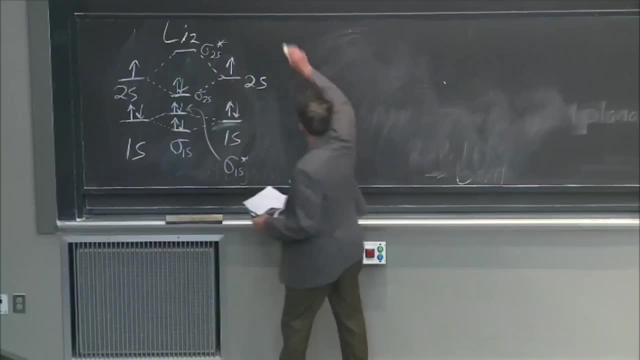 interesting that happens, Because now that sign you see how the p has a plus and a minus right, And so you've got to kind of think about that a little bit. OK, If I take a p orbital, and I'm going to take a, 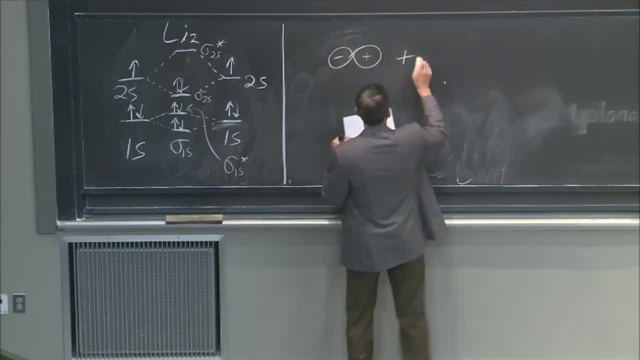 I'm going to do it like this: minus plus, And I'm going to add it to a p orbital that looks like this. And notice, I'm taking these and I'm adding them along an axis, where they're kind of both along the axis. 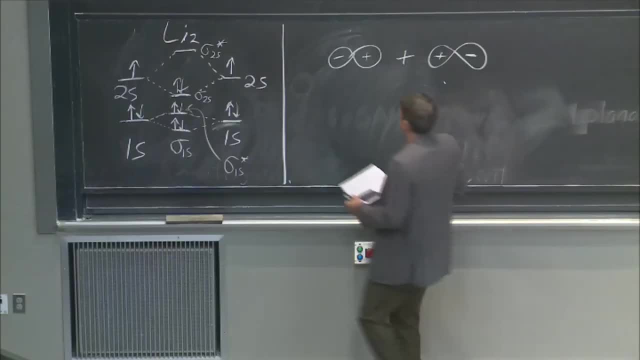 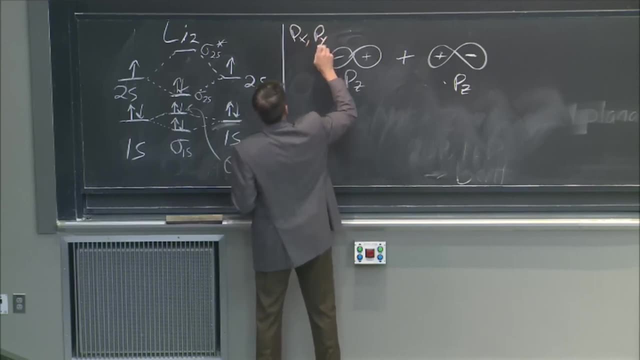 They're both along the axis And by convention we'll do the pz as the one along the axis. Remember there's px, py and pz When we solve for the p orbitals. those are the m's. Those are the m's. 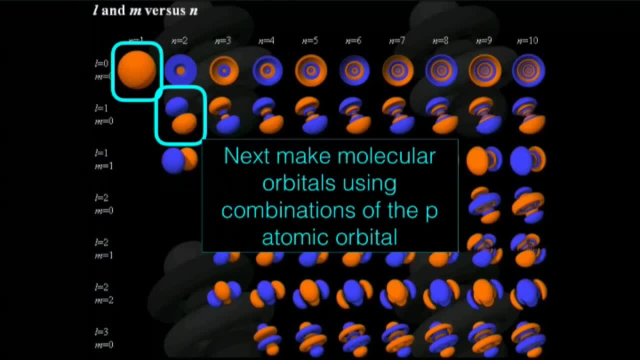 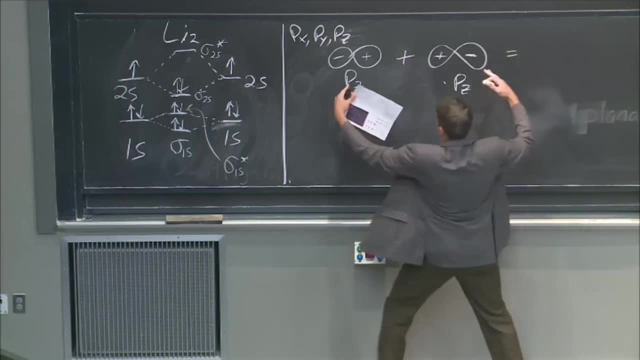 1, 0, minus 1.. Now, by convention, we put the pz along the bonding axis And you can see right away: If I do this, I'm going to start adding these wave functions constructively, And what you're going to get is: let's see if I can draw this. 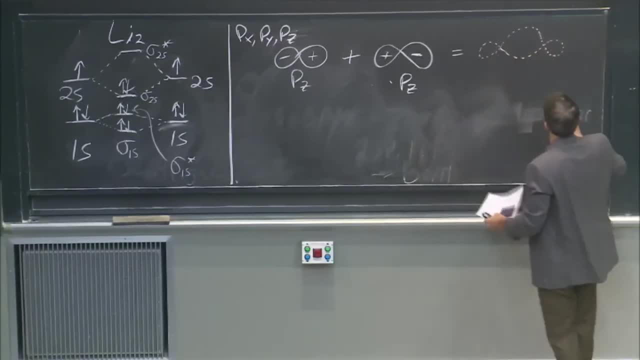 is something that looks like that and where this is actually going to be plus and this is minus. And notice, I'm going to have nodes in there. right, I had nodes in the original orbitals, but I got a lot of bonding in between. 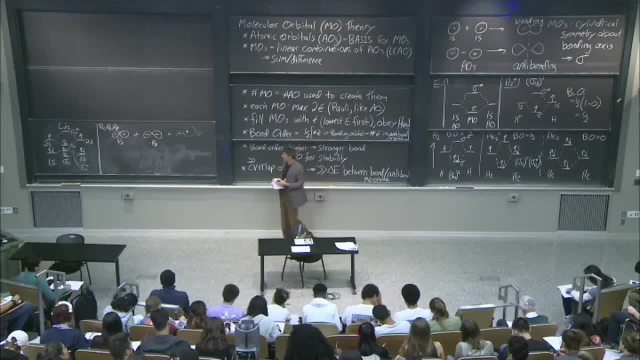 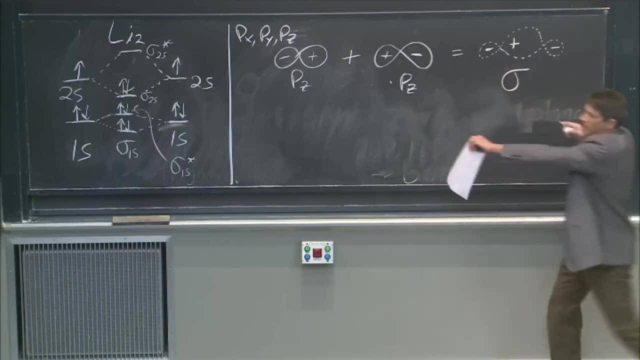 I got a lot of bonding density in between. That is a bonding orbital. That is a bonding orbital, And the other thing we see about this is that it is symmetric around that bonding axis, So it's actually a sigma pz orbital. It's a sigma. 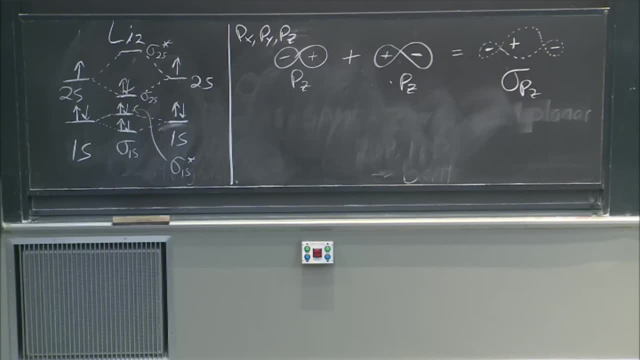 We call it a sigma because it's symmetric around the bonding axis. Now, if I were to take a px, oh well, let's subtract these. OK, so minus plus minus. Now what you see is something very different, right? 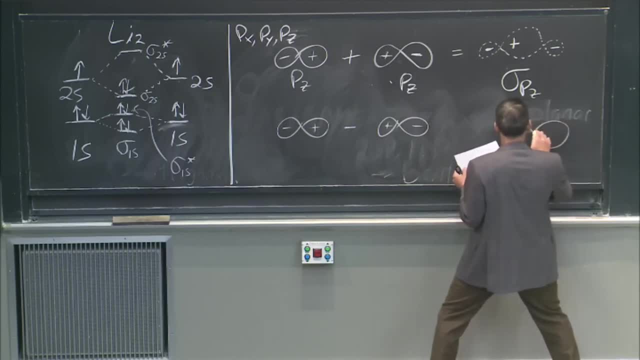 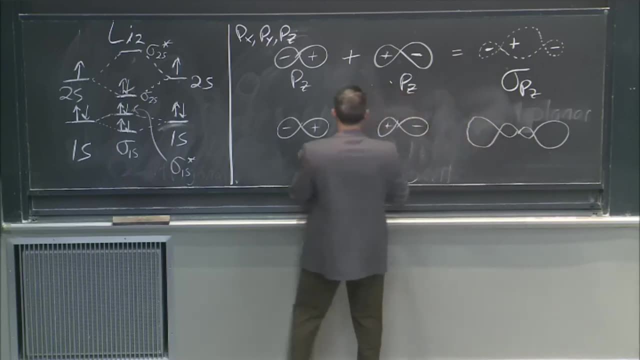 So now, oh boy, can I draw this? Maybe, I don't know. OK, I'll take that right. And so now, what you see? so I'm subtracting these, And so the density goes down, And now you're going to get minus minus, plus plus. 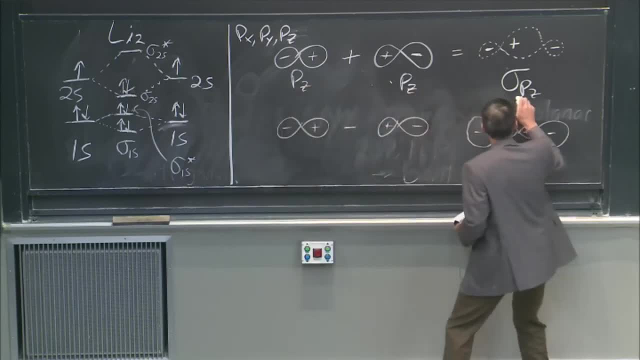 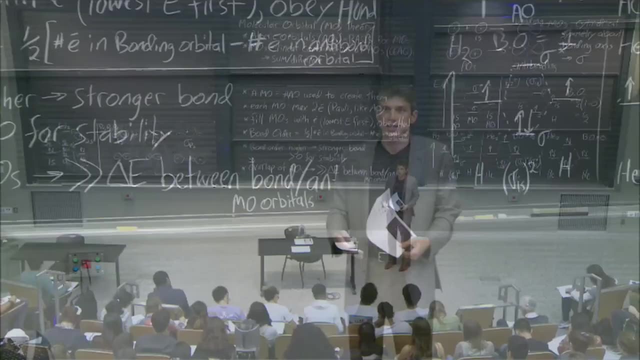 But I've reduced the electron density And even worse, I'm back to that situation where, right in between, where I want to share the most, I'm saying no, no probability density there, And that's an antibonding sigma p orbital. 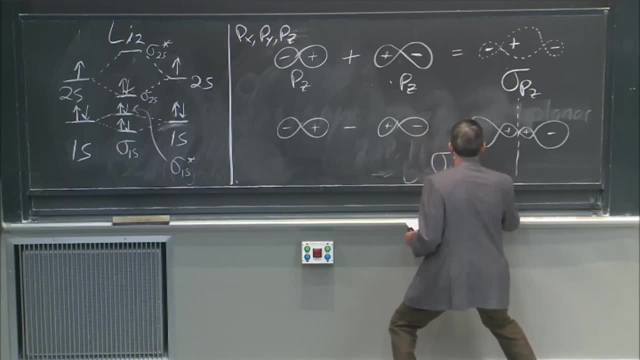 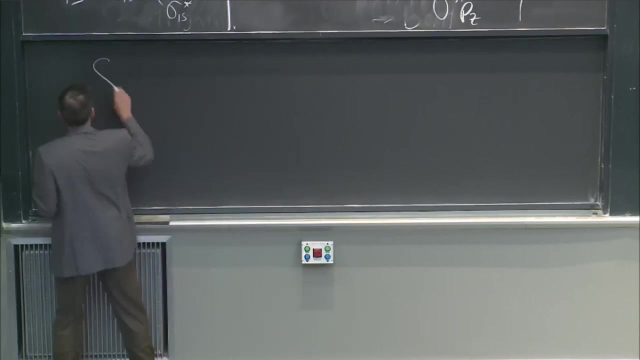 So this would be sigma star pz. OK, Sigma star pz. Now the other thing that you can do is look at the other directions, right, And so I'll just take one of those really quick, And if you do that, you see something different, right. 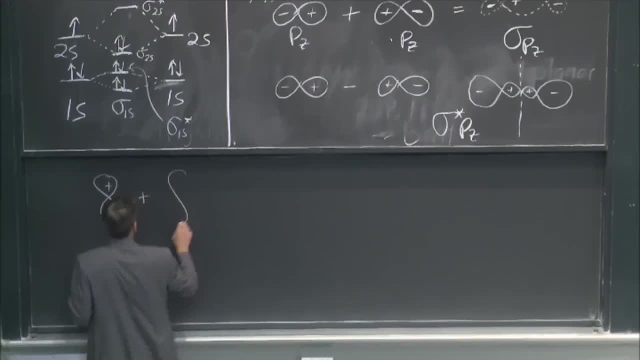 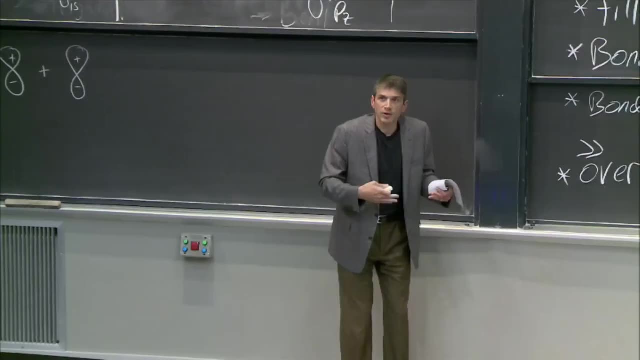 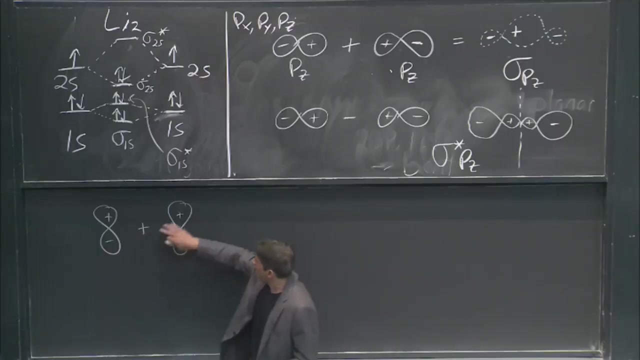 So now let's combine these like this. By the way, some textbooks we're adding and subtracting, We're constructively interfering and destructively interfering. Yeah, So sometimes you'll see a textbook add like this, or add the other way, which is subtracting, like this: 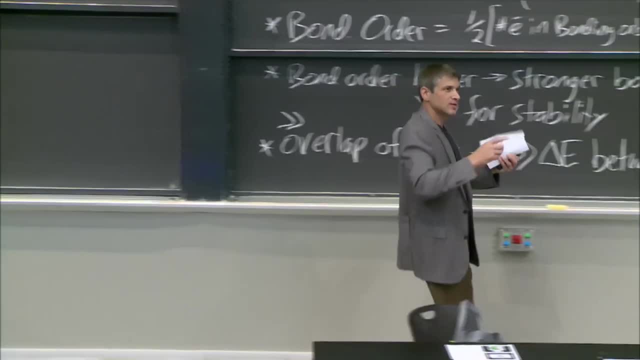 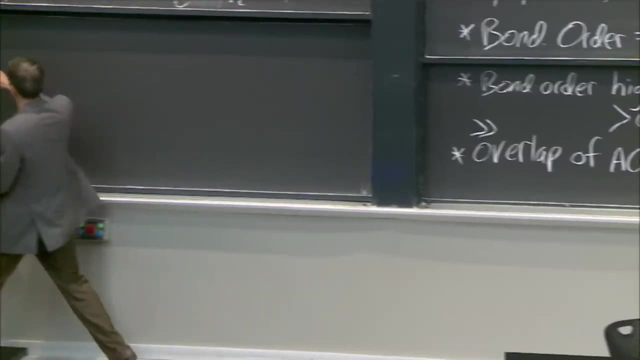 It's the same thing, right? You can decide how you want to orient it, But we're adding and subtracting constructively and destructively. That's what we're doing. So I'm going to choose to add it like this, because then you just see if I do this. 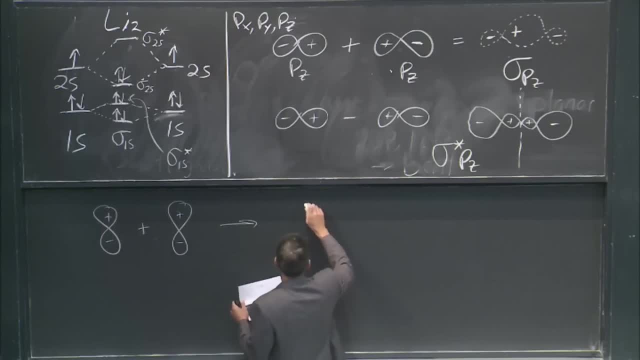 then those are going to have some kind of overlap, right. Those are going to have some overlap of plus up here and some overlap of minus down there, And that is called a pi orbital. Yeah, Yeah, but if I subtracted them, then what you would see? 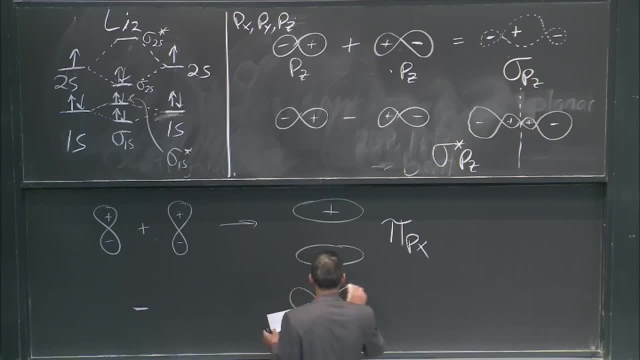 is something that looks more like this, where you got that node in between again right, And this would be a pi star orbital. This would be for like px orbitals. Now notice: these cannot be sigmas, Because the pi orbital is not symmetric. 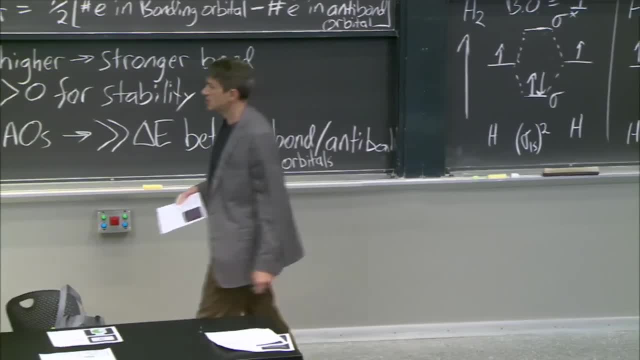 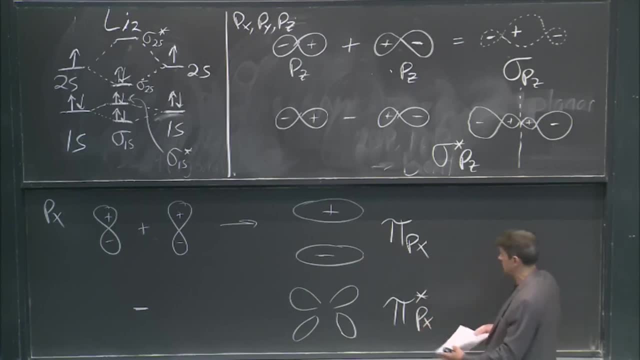 around the bonding axis. OK, These cannot be sigmas, But that's why we have another symbol for them. Luckily, we've got a lot of symbols, And the chemists are geniuses at naming things, And so these are called pi orbitals. 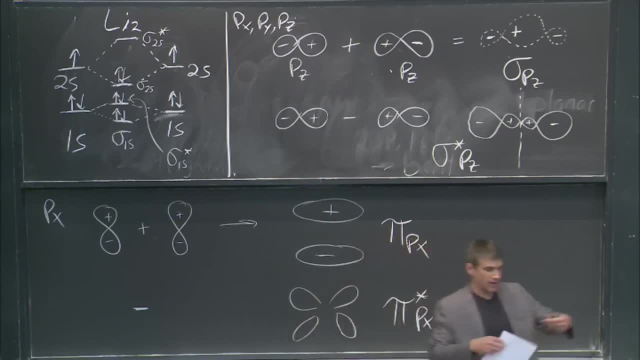 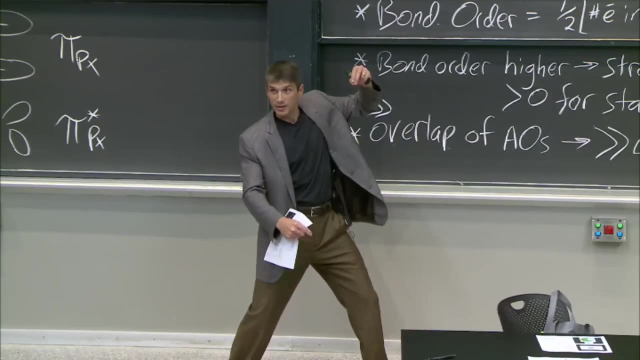 And, as you can see, OK, I used our three p orbitals. One was I put it along the axis And then I've got two going perpendicular in the other plane, And this is one of them, And then the other one would be the other one px. 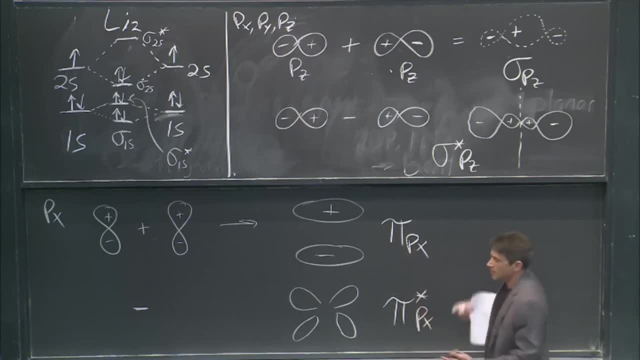 And then the other one is py. So, as you can see, I'm going to have a sigma, a sigma star, two pi orbitals and two pi star orbitals, right? And then what we got to do is we got to put them on our energy scale. 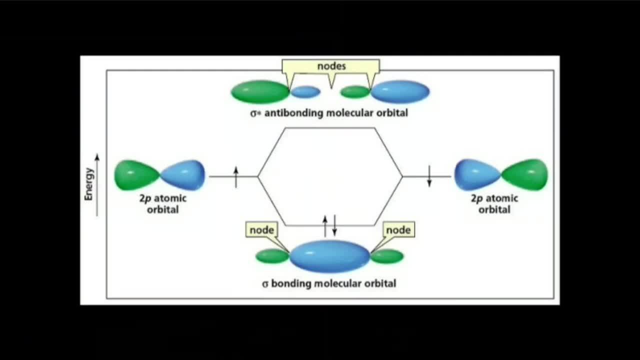 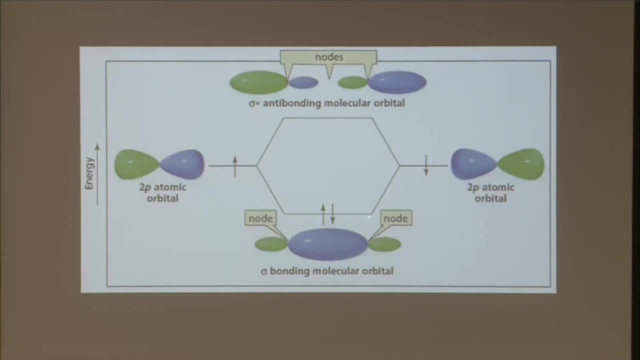 And instead of going through drawing it all, save myself a few minutes here. I'll show it to you right? So there's the energy scale And oh, they're pointing out the nodes. Isn't that beautiful You can see right here. they're not saying what molecule this. 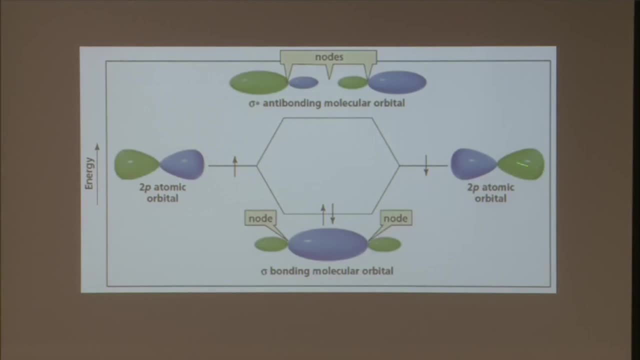 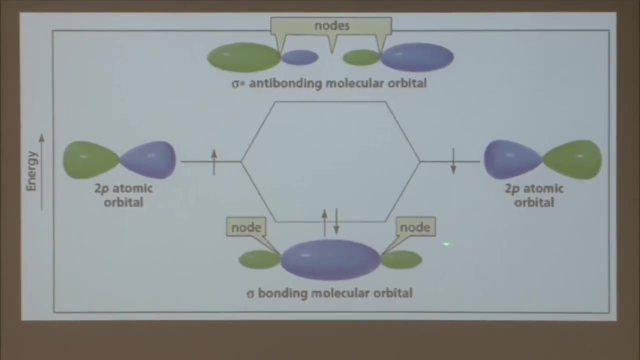 is, yet It's a p orbital And it's pointing along the same bond axis, right? So this is going to be a sigma p orbital. This is a sigma p orbital, You can see that. And there's a sigma star, right. 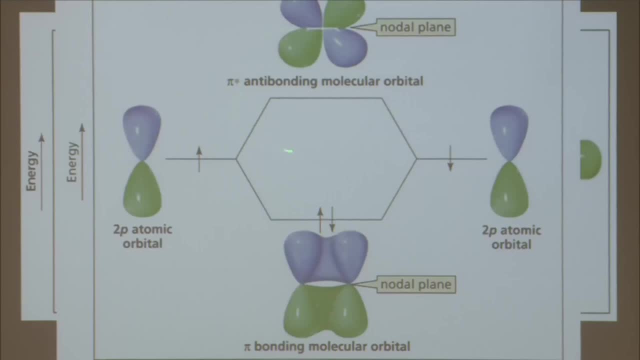 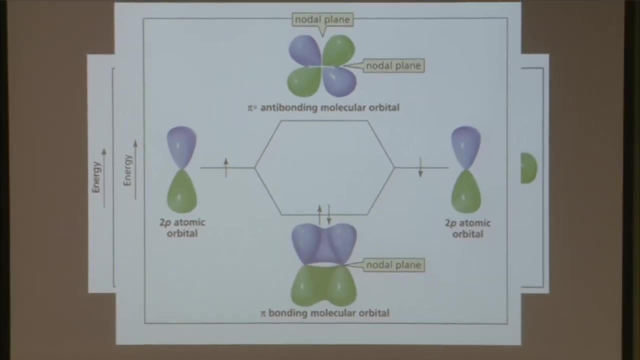 Good, If we go to that, there's the next one, There's a pi orbital And you get the same exact effect. You've got a lowering of the energy because you're putting electrons on the bond and a raising of the energy because you're. 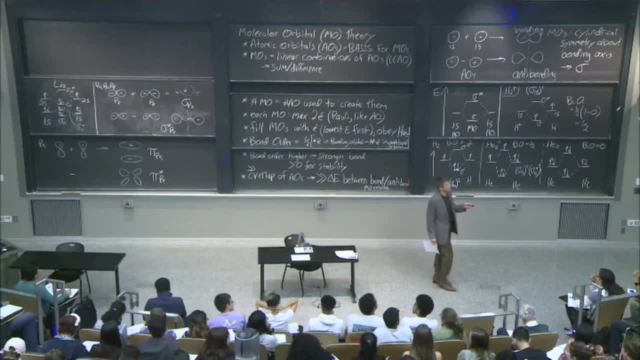 taking them away, right, Right, And that's what it looks like for the pi orbital, And we can put it all together. And if you put it all together, what I want to do is put it together for O2, and then show you a video. 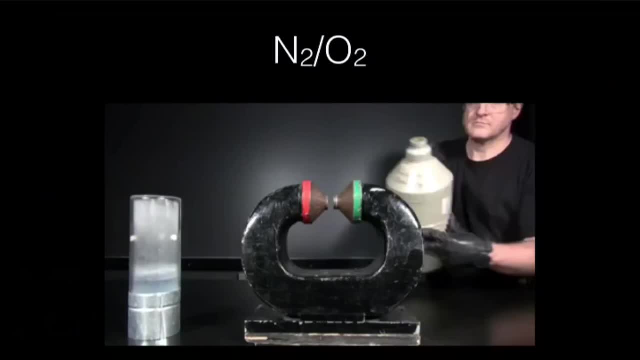 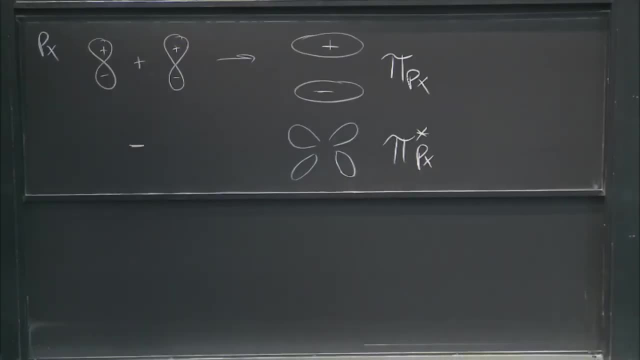 and then do my Why This Matters. Now, if you put this together, I'm going to show you the system for oxygen and nitrogen, OK, And then we'll do a couple other cases too. But we're going to do oxygen first. 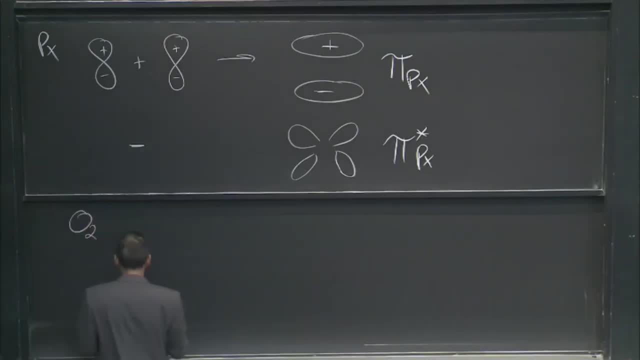 So if I take oxygen, then I've got my two. I'm not even going to write 1s any more. That's way down in energy. It's not really involved in the bonding, I'm going to leave it out, But I've got my oxygen. 1s oxygen, 1s. 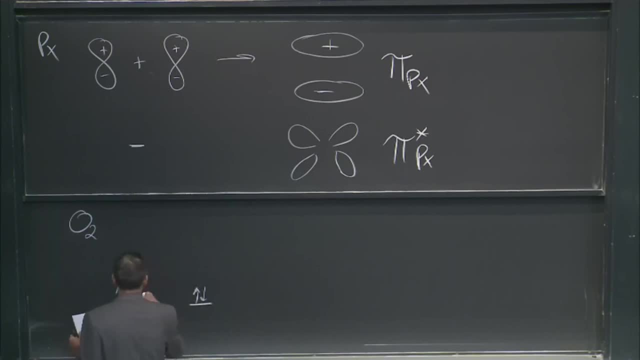 OK, good, So those are going to come in and form molecular orbitals like that, And we know that they are all filled. OK now, But on, Now, up here I've got my oxygen. Sorry, I just said I wasn't going to do 1s and I'm not. 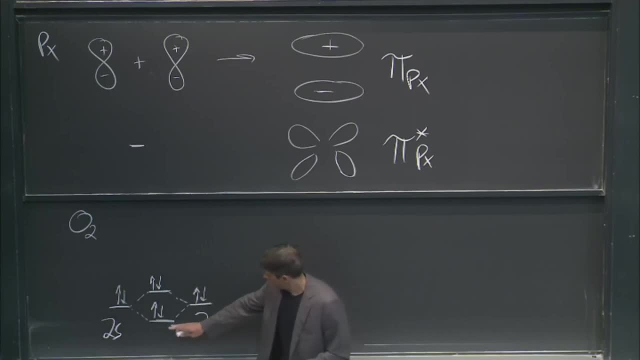 Those are 2s. Those are 2s. Sigma 2s, Sigma star 2s. OK, good, All right, Let's see Now over here. I start with my p's And I start with px, px, py, pz. 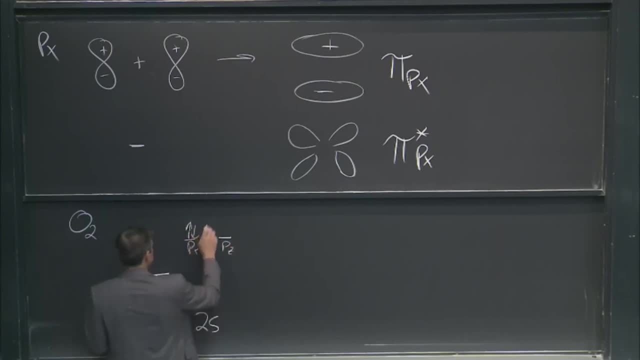 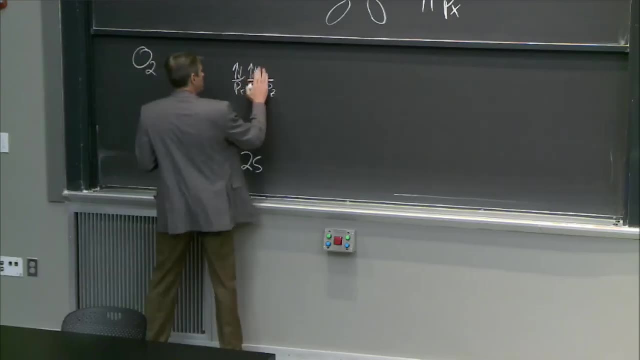 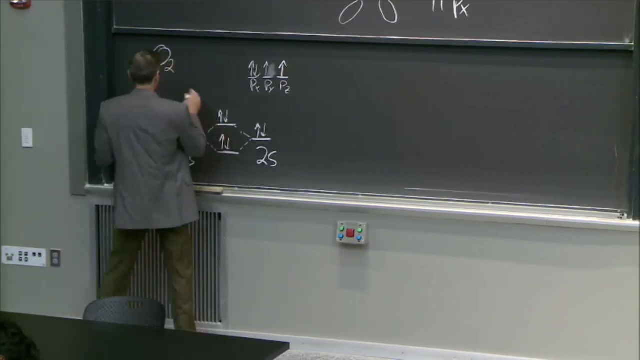 And in oxygen, how many electrons do I have in here? So it's like this: Everybody should be shouting: That was so much better, That was close, And then I've got to. I'm not going to have enough room. I've got these over here. 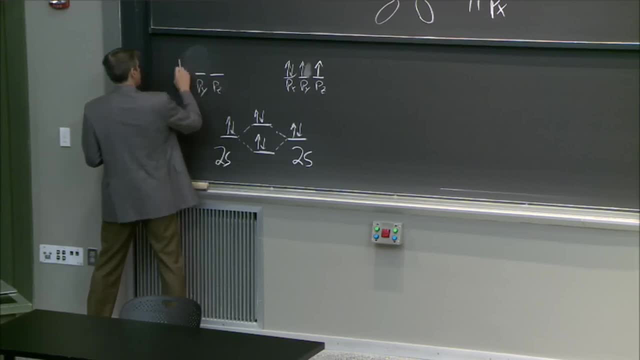 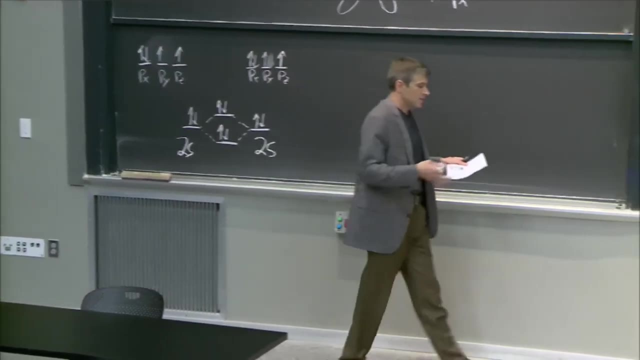 Px, py, pz And there is oxygen. But you see, now they come together And they form these MOs And we just went over what types they are. There's a sigma pz- orbital and there's a sigma m. 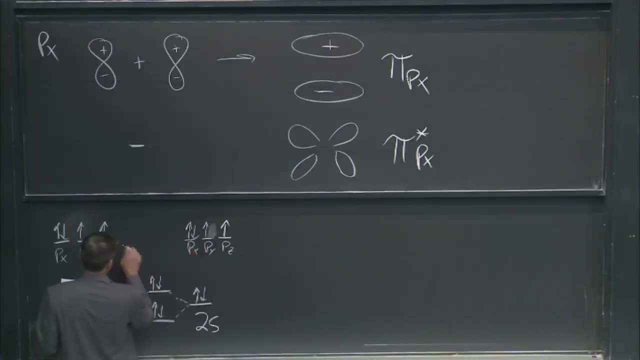 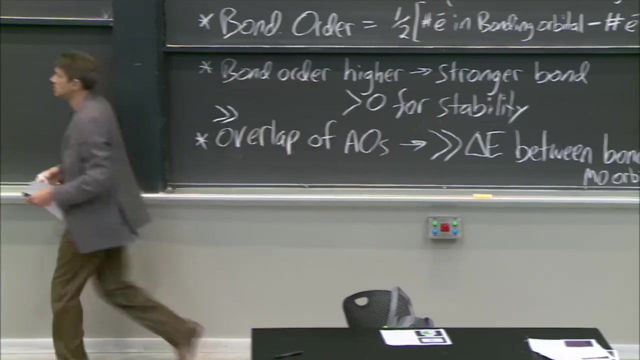 But the ordering is about the same thing that we learned, which is that it has to do: this delta is up there, This delta is up there, And so in that pz for oxygen you can overlap more. It pushes those apart more. 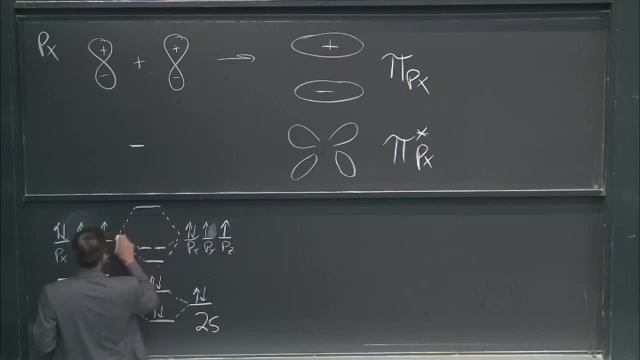 And so what you get is that the pi's are in there. They're inside, like that. The pi's are inside. So this would be right in here. it's going to get too small, So I'm going to do this. 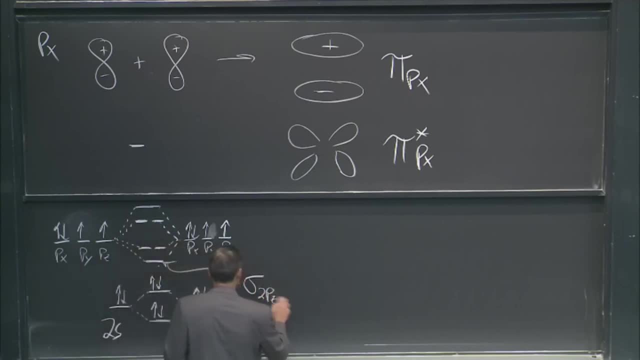 This would be a sigma 2pz, This would be a sigma 2pz star, And over here these would be pi orbitals, Pi, Pi, px, pi py And these would be- I almost can fit- pi star px and pi star py. 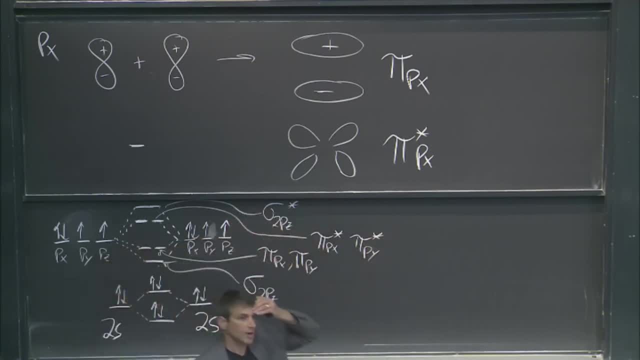 All looking like the shapes that we've been drawing. And then the filling part comes from the filling of the AOs. I've got my filling of the AOs here. I've got the valence filling for oxygen. There's a 1s down there. 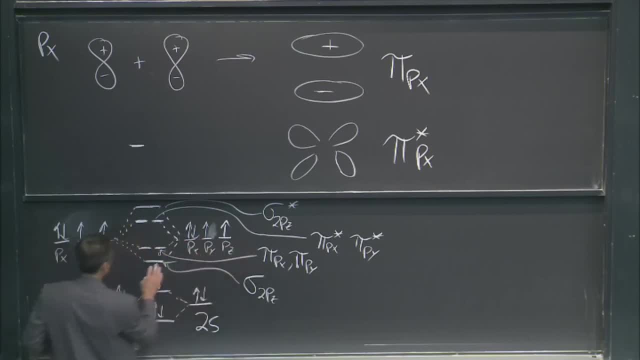 And so I've got to put four electrons from there And four electrons from here into the middle. So let's do that: 1, 2,, 3,, 4,, 5,, 6,, 7, 8.. 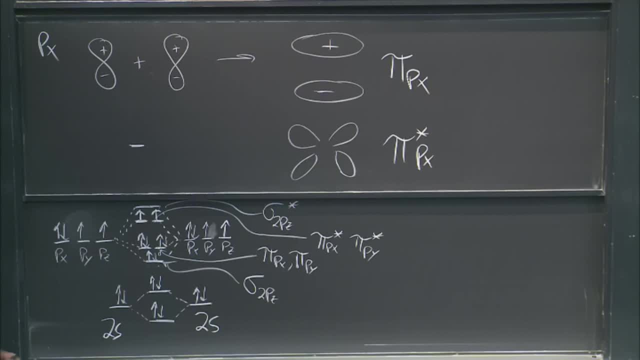 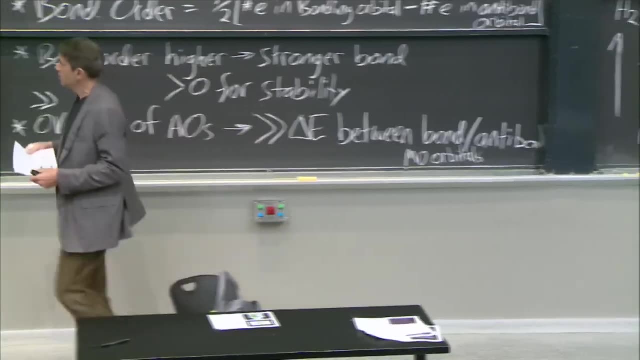 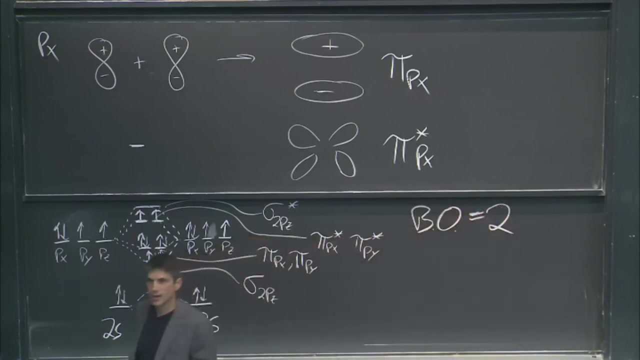 Pauli Pauli Right. So for oxygen, the bond order, if you add it up, the Bo is 2.. It's a double bond. We know that, Oh, but now we know so much more, And this is what I want to make. 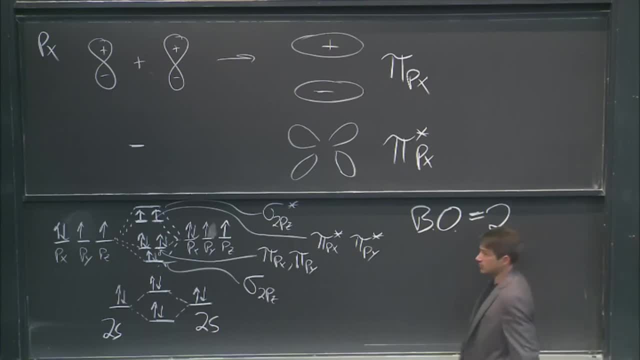 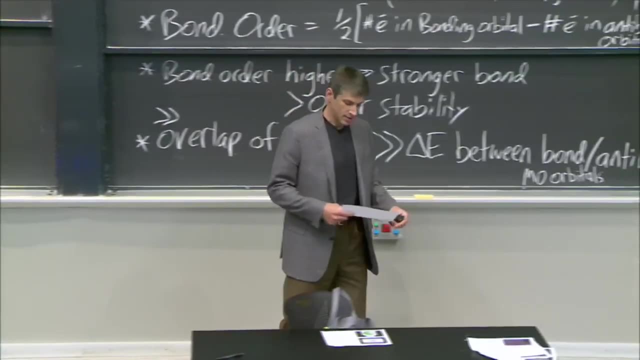 Lewis could have gotten us this, But Lewis can't get us magnetism. Lewis can't get us magnetism. Molecular orbital theory can, And let me show you magnetism right up close, Because if I take liquid nitrogen that's not me. 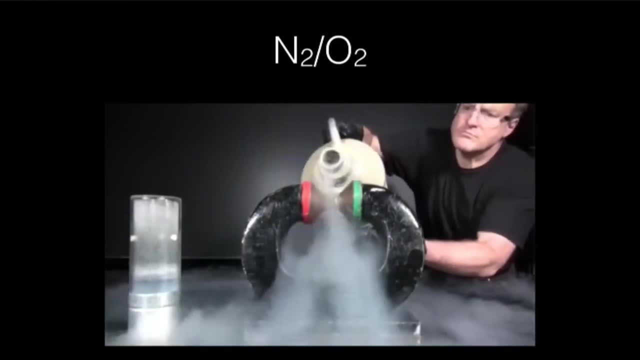 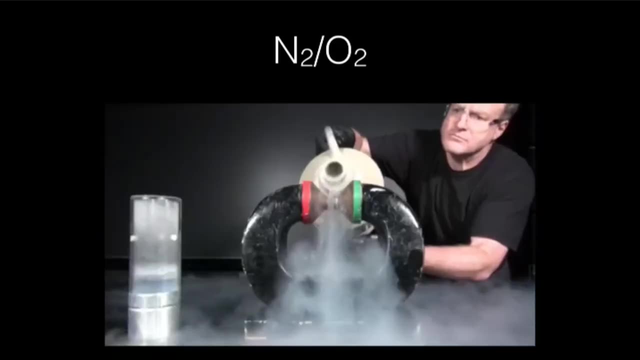 though, and I pour it through a huge magnet. I want that magnet so badly, But if I did that, look at that, liquid nitrogen just goes right on through, And it's really fun to do actually. And so there you go. 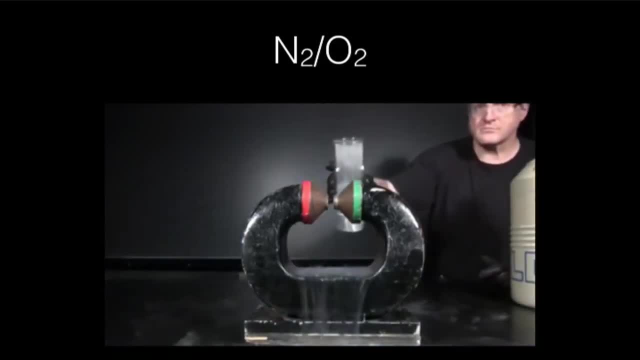 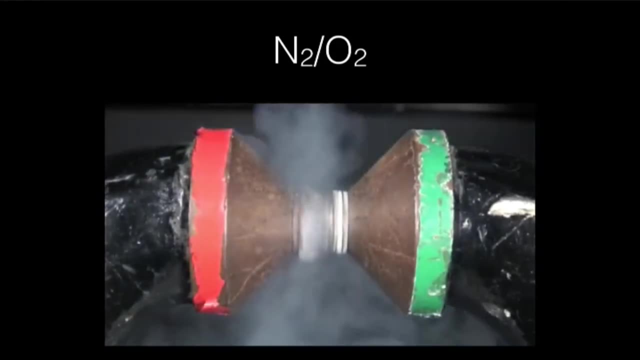 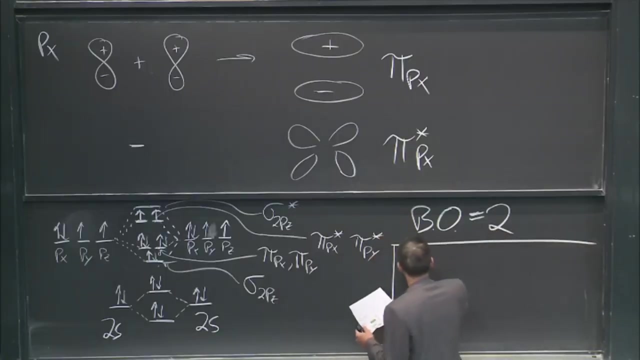 That's liquid nitrogen. But what happens? Look at liquid oxygen. Liquid oxygen. Now you pour it through and the magnet holds it in place. Woe is right. There's four more things we got to cover. One is paramagnetism. 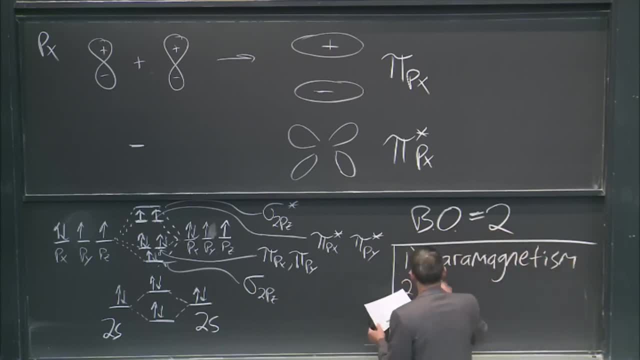 Another is something called mixing. Another is what happens when you go heteronuclear. Oh yeah, See what that means in a second. And finally, what I said I would get to, which is nonbonding, which are not the same as antibonding. 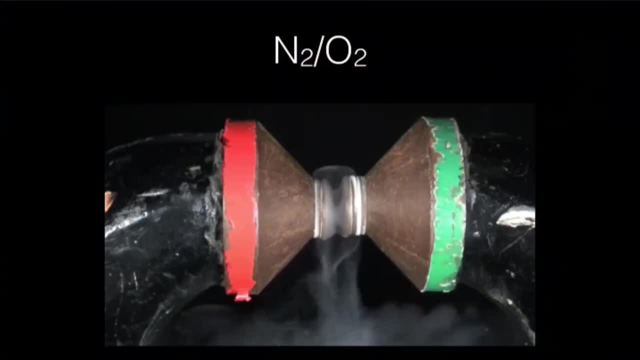 What I'm covering right now there is paramagnetism Because, as you saw In the exam, in one of the questions we explained it. We said: if you got unpaired electrons, if you got unpaired electrons, then you are paramagnetism. 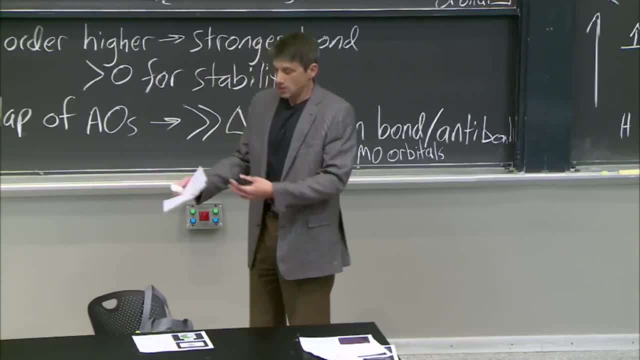 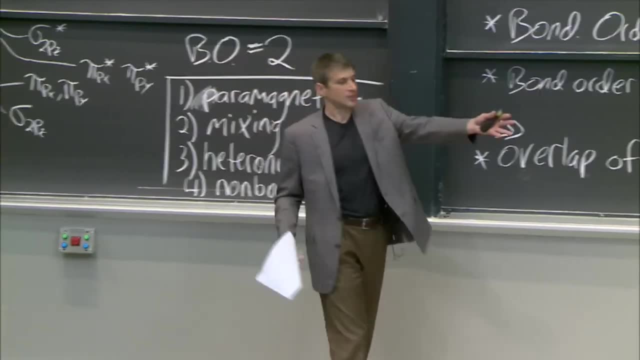 What does paramagnetism mean? It means that if you put a huge magnet on it, you respond. You will feel a force from that magnetic field, And so we did that in the exam. We had a silicon atom because we hadn't done molecules. 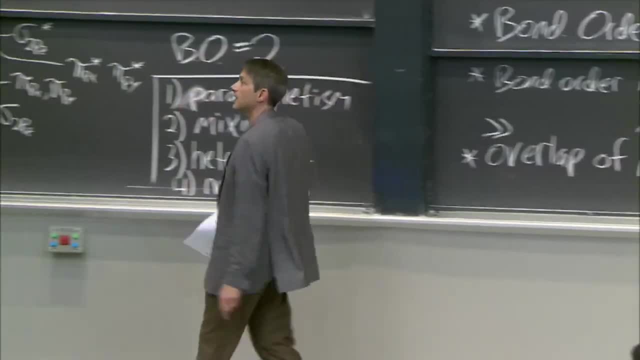 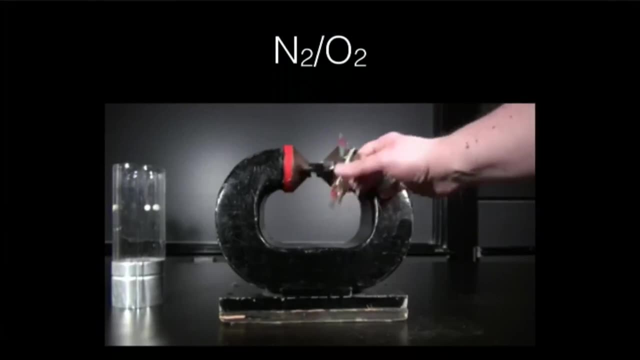 But now we've got molecules, So I can tell you why that experiment happens. What's happening? I can tell you why that experiment happens. Really, I didn't even know there was more. It happens because of Hund's rule: molecular orbitals. 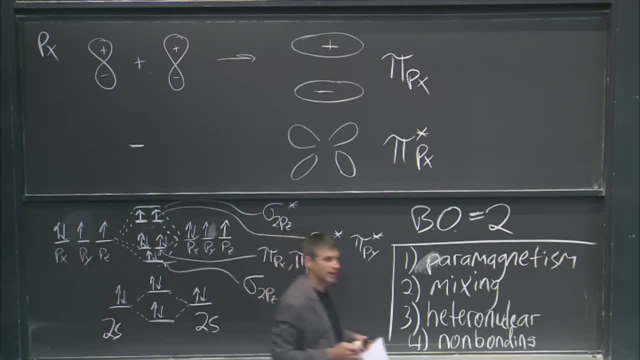 and the fact that I've got these two unpaired electrons in the O2 molecule- And you know that in nitrogen those two electrons are gone because nitrogen is missing one more here and here. So you've got two less. Everything's filled. 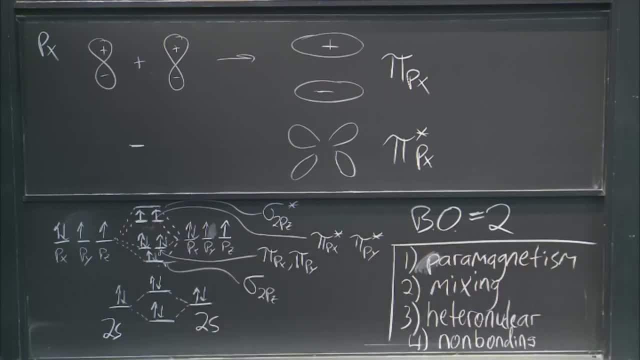 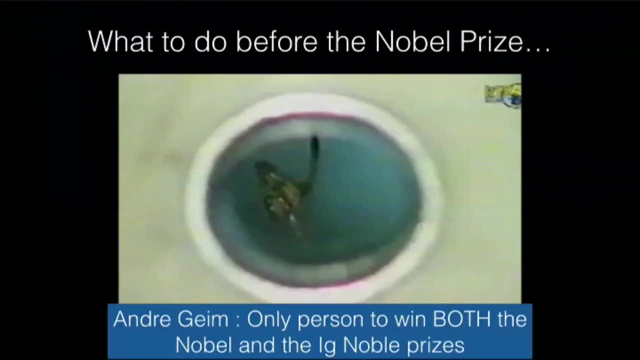 Everything's filled. Paramagnetism Now. OK, Speaking of magnetism, I couldn't help but show you this: This is diamagnetism Now. diamagnetism: everything is filled, But you still feel a little repulsion to a magnetic field. 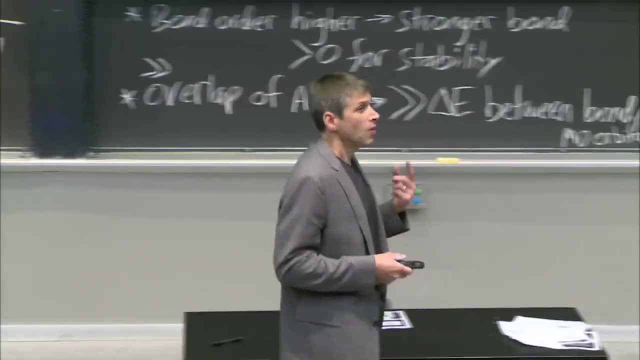 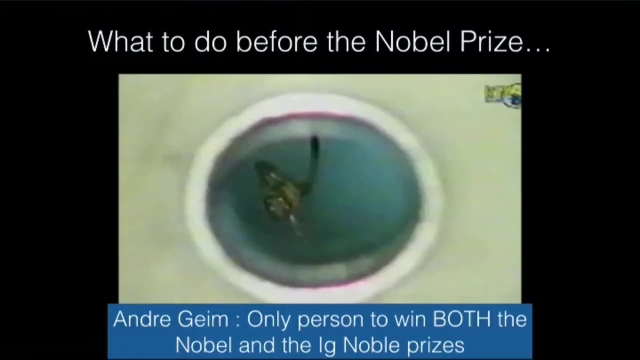 And some of you may know, there's this thing called the Ig Nobel Prize. Only one person in history has won both the Ig Nobel and the Nobel Prize: Andre Geim, who discovered graphene with scotch tape, But before that he won the Ig Nobel Prize. 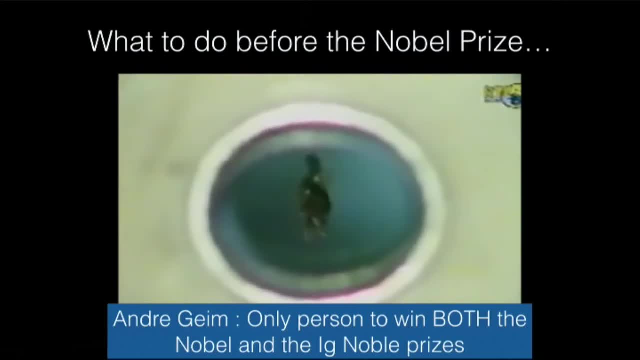 because he did this to frogs Because water is diamagnetic and so it repels the magnetic field. This has got to be really, really, really high. I hope that frog was OK. It looked sort of OK. So the frog is floating and it's. 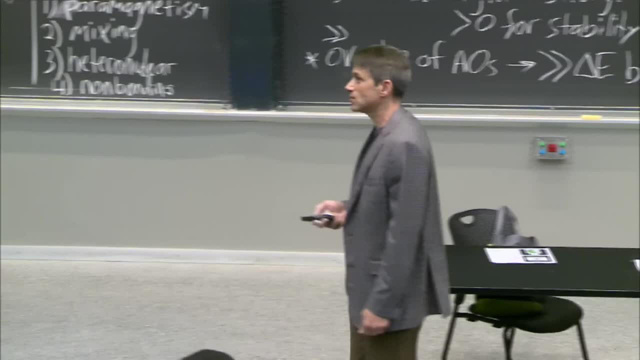 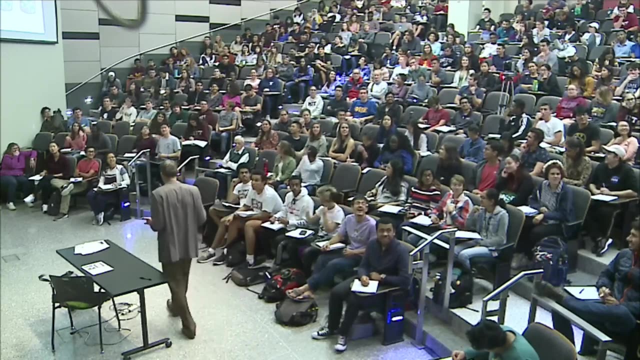 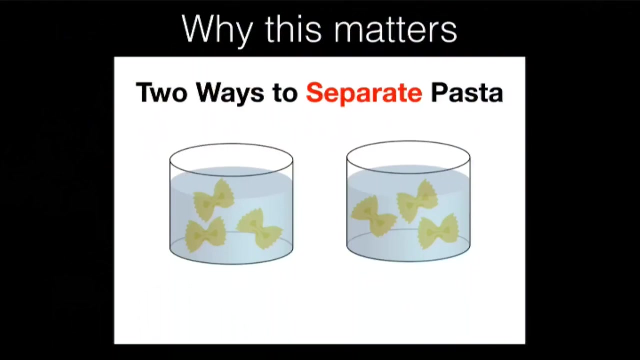 like a study about levitation using magnetism. Why am I showing that to you? No particular reason, But this does get me to the why this matters, which has to do with how you cook pasta And, of course, since we're talking about O2,. 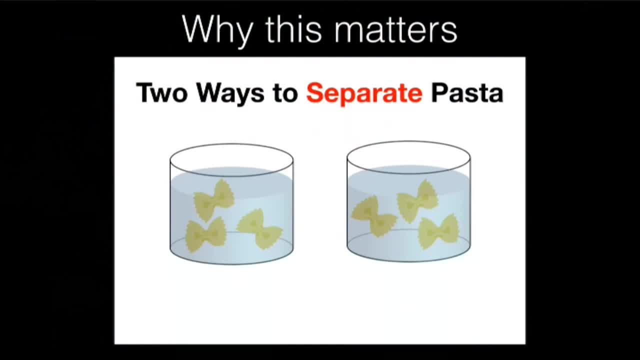 when I have finished cooking pasta, what do I do? I pour it there. it is through. it's sophisticated. I pour it through a colander. That's a membrane. That's a membrane. You did use a membrane. You did a filter. 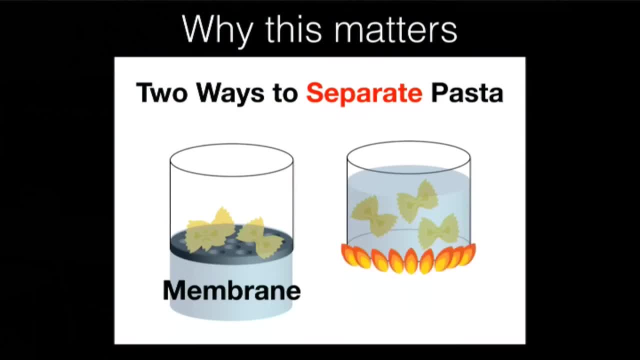 But I could also have done that separation, that same separation. I could have left it on the stove, I could have, And it would have boiled out all the water and left me still with the pasta separated from the water. I've accomplished the same exact thing. 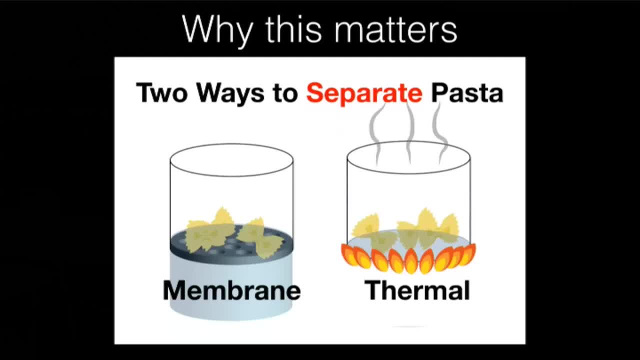 I have separated the pasta. I've separated the pasta from the water Task. done Pasta may not taste as good, But you've done it. But see, the thing is that if you separate things this way versus that way, you can just. 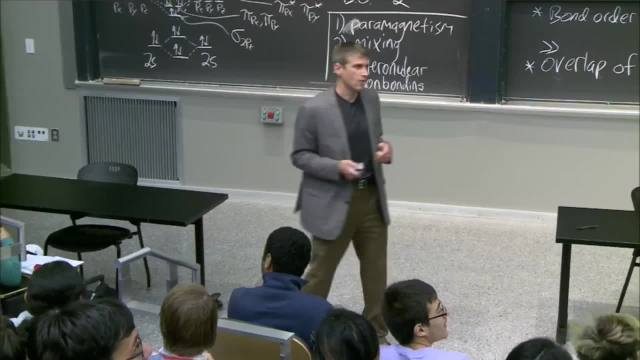 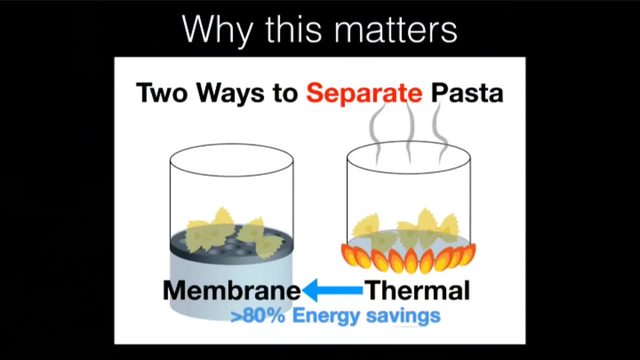 feel how much less energy it's going to take. In fact, you can save over 80% of the energy if you do a membrane-based separation as opposed to a thermal one, Gesundheit. So those are two ways to separate pasta. 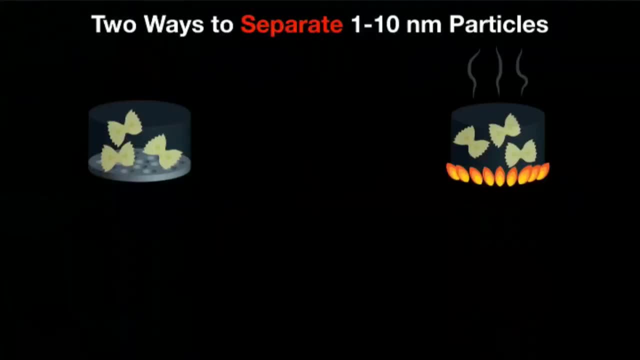 But see, there's two ways to separate lots of things Like: how about 1 to 10 nanometer particles? How about chemistry? How about molecules? How do you separate those? Well, you've got the same two ways, And if you count up all the things we separate this way, 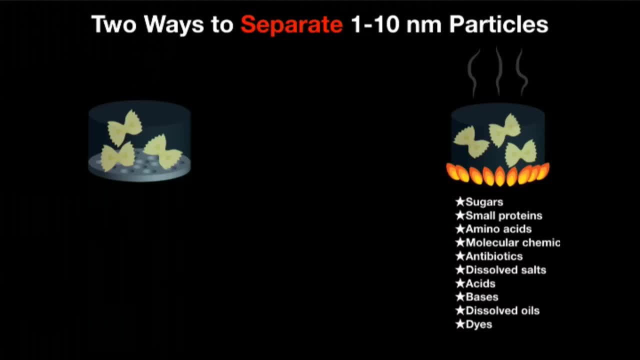 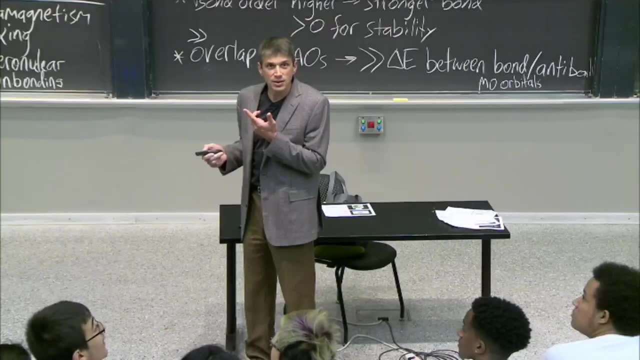 it's a lot. It goes on and on and it will go all the way down the infinite corridor. This is how we do chemistry, In fact. has anyone seen this on the side of the road? That's a distillation column. 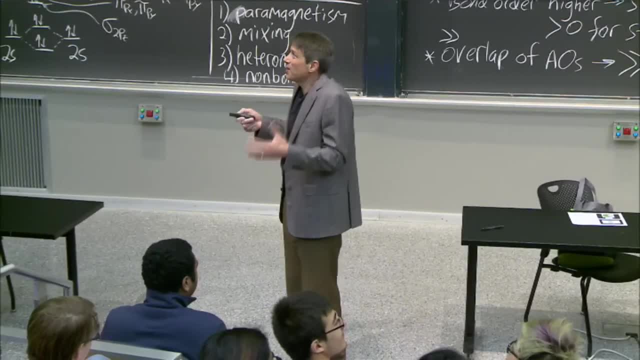 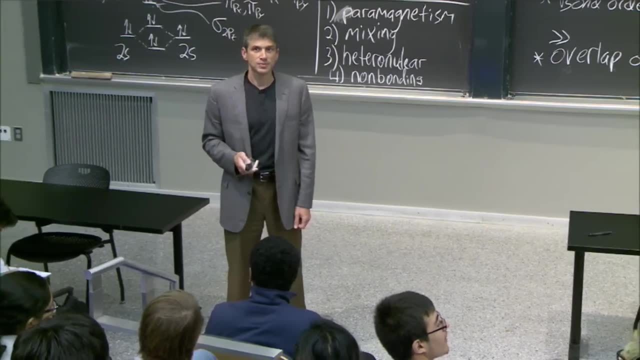 It's a big pasta cooker That's. all you're doing is boiling one molecule off of another Over a long time, with a whole lot of fossil fuel. In fact, if you look at the US energy consumption, roughly a third goes into industry. 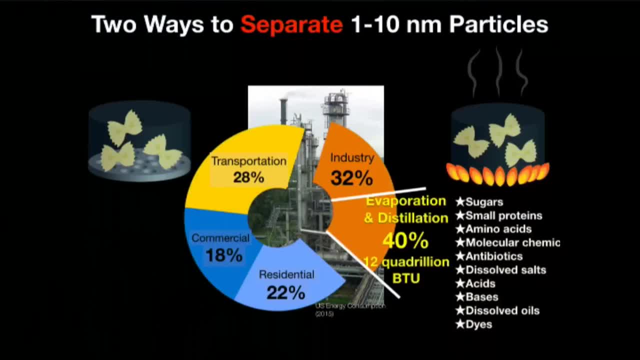 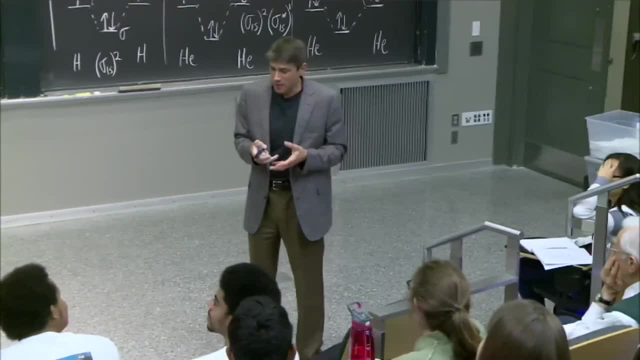 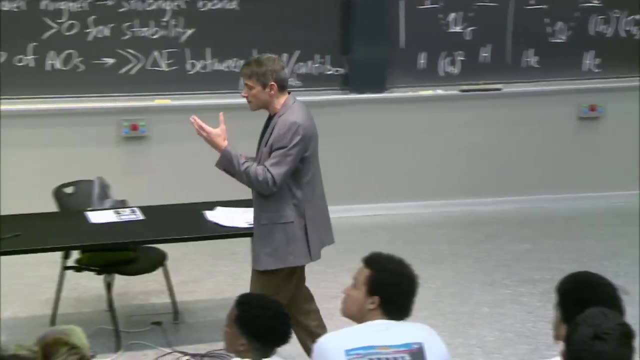 40% of that is for this one thing. It's boiling pasta. But the pasta is 1 nanometer to 10 nanometer particles. 40% goes into boiling one chemical species off of another. Separation. Separation, That's 12% of all the energy. 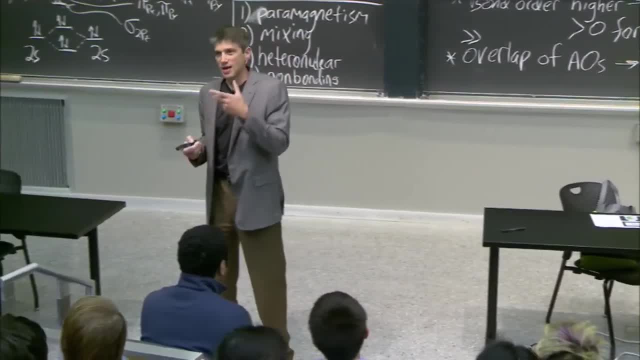 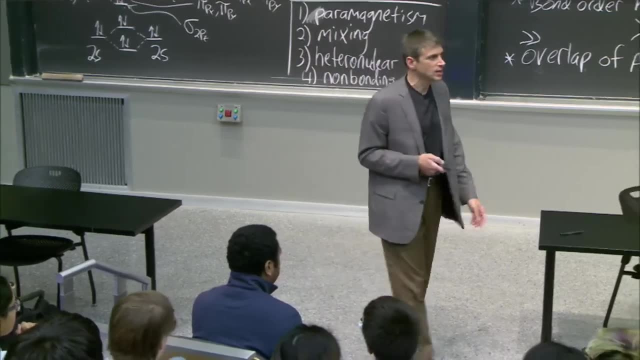 That's the same. That's the same, That's the same. That's every single drop of gasoline in every single car, truck and bus. That's just to give you a sense of how much energy that is. Well, why aren't we using a colander? Why don't we just pour it through a colander, like we do our boiling pasta? Well, we do that for one field- desalination- I got a why this matters on that another time. But we don't do it for all those other things. and there's a really simple reason: We don't have the right pasta colander. We don't. There's no option for that size scale that can withstand the conditions that are in all of those chemical separations. But if we did this, we take so much O2 out of the air. 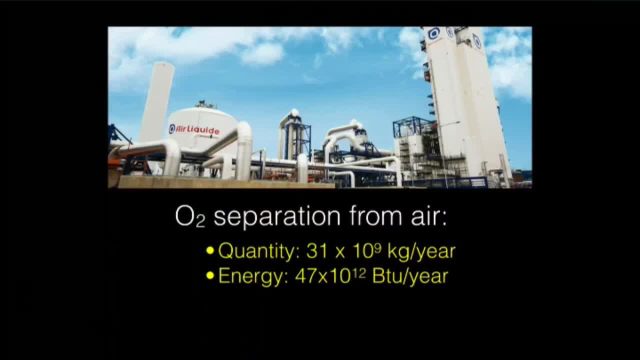 We need O2, but we don't want the N2. So we have to separate. How do we do it? We go cryogenic, We go to very, very cold temperatures, which is the same as boiling, But you're still spending all this fossil fuel. 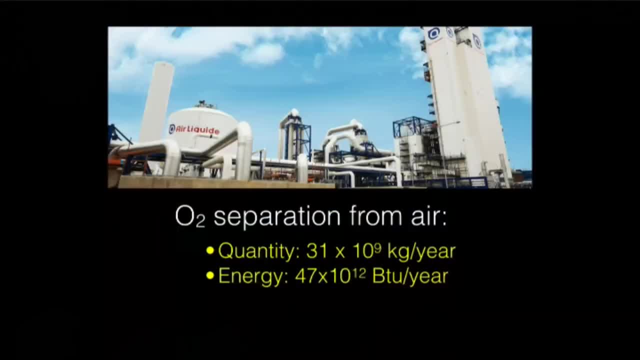 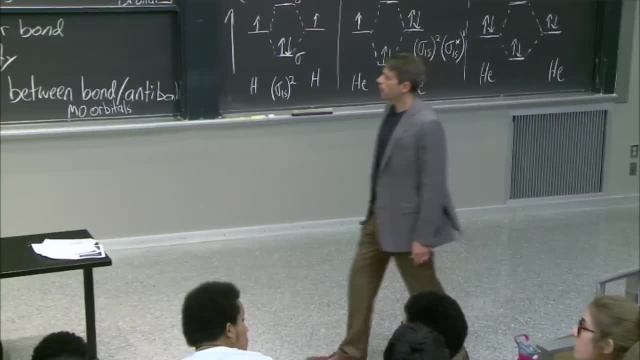 to lower the temperature. That's how much O2 we generate each time, Each year. right, And this is how much energy it takes- It's like half a percent of all US energy just to get. But what if you could use something? like O2's paramagnetism. What if you could use something about the chemistry of O2 to do this separation more efficiently, lower energy, or maybe make a new colander that does that? And if any of you have ideas, come talk to me. 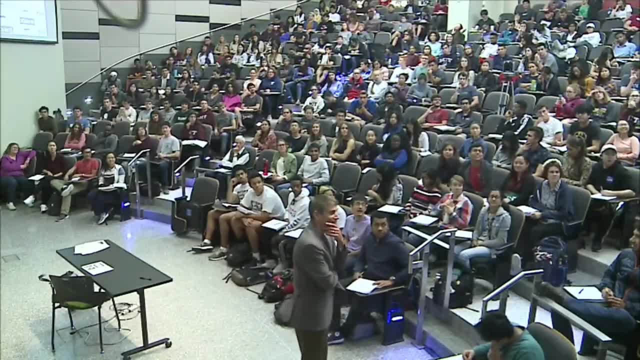 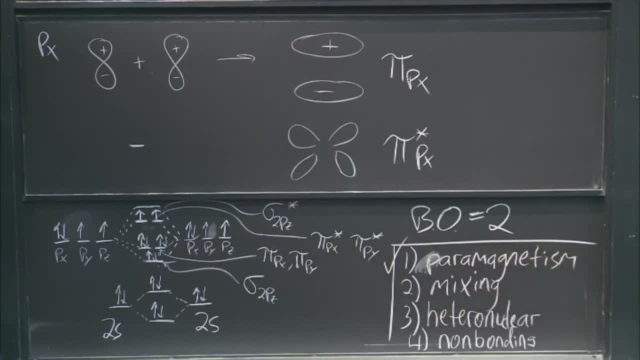 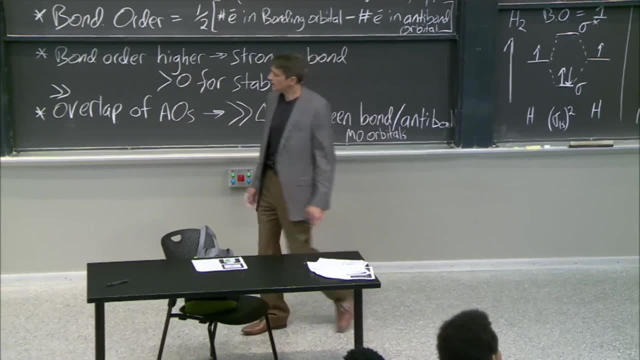 This is a problem I care a lot about. OK, But I had some other paramagnetism, unpaired electrons. We got that one. Ha Ha. Why is chemistry not? Why can't they follow the rules? Why? But they always got to break them. 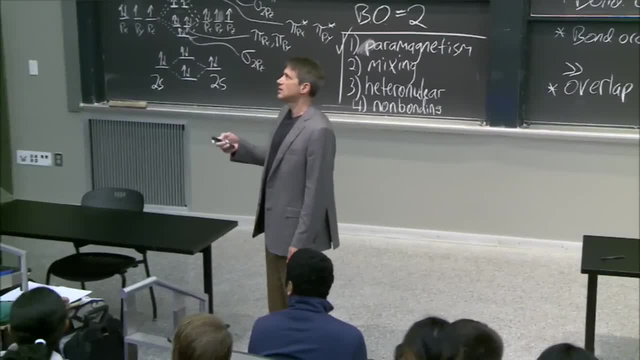 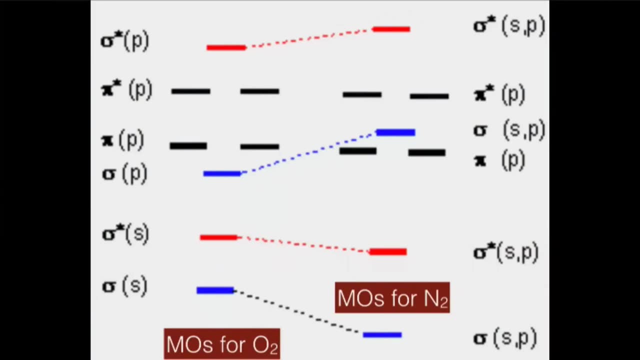 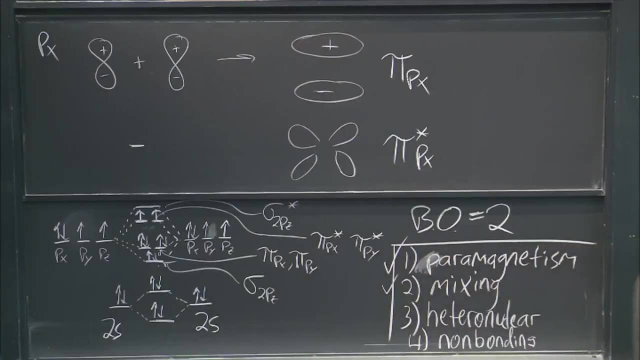 And what we see. well, this was oxygen Sigma sigma s, sigma sigma stars, pi pi star. But look at what happens for nitrogen. Ha Why? Because of something Some people like to call it mixing, All it says. remember I said that if we where did it? 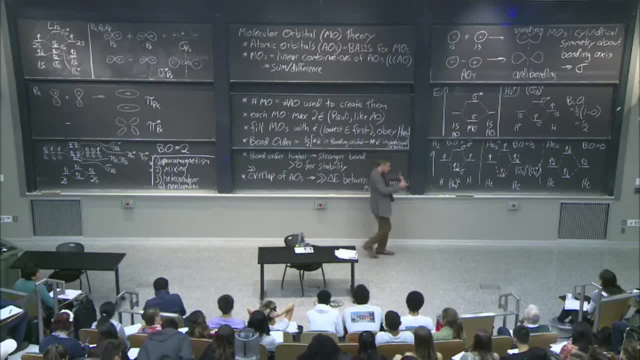 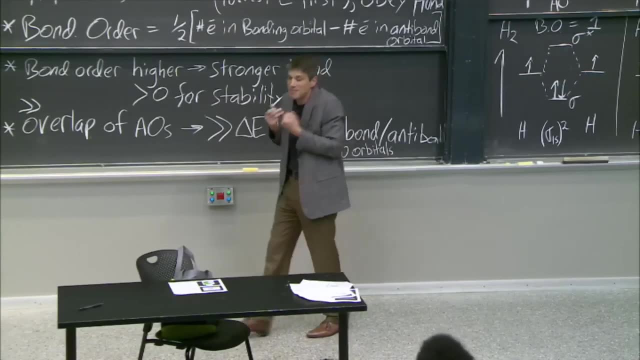 Somewhere I said that the closer an energy or the closer in symmetry orbitals are, the more overlap they can have and the more they interact and can mix together in the ways that I've been talking about. Well, it turns out that if you go below oxygen, in what? 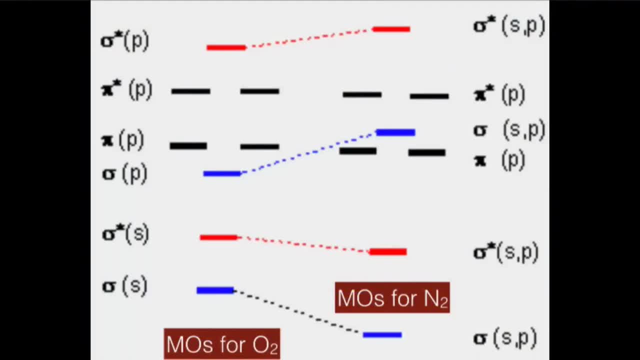 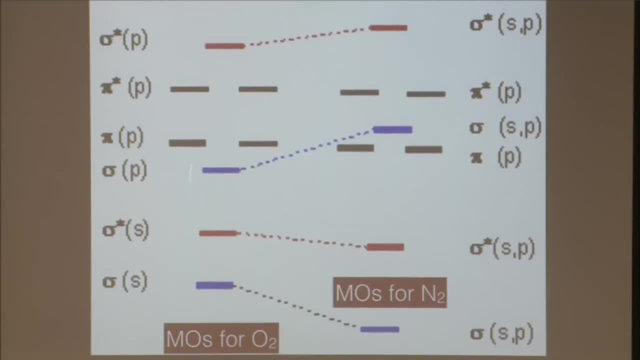 are called homonuclear dimers, which is where the atoms are the same. then you can get mixing even between this sigma and that sigma, And so what happens is, instead of them being kind of separate- like this for N2,, there's an interaction. 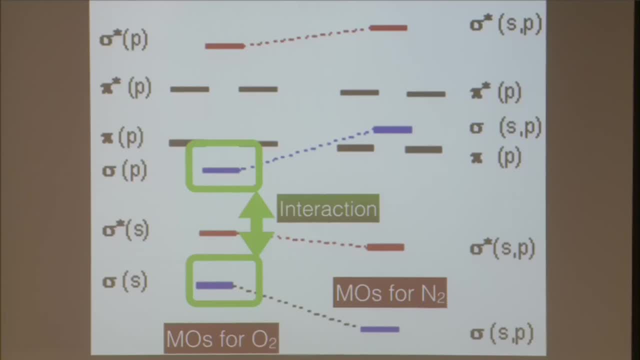 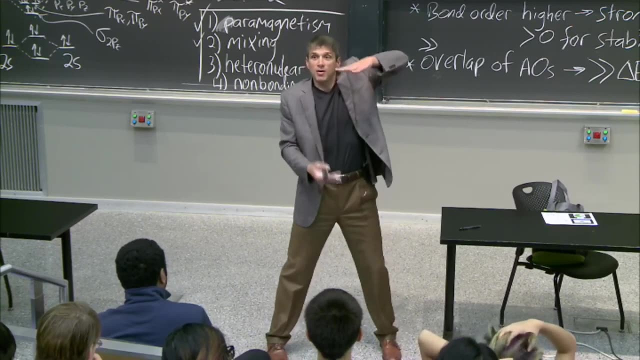 You see, You can think about it the same way. I'm throwing more orbitals into the mix And so, because they can contribute to overlapping, you're changing that delta E even more. That's effectively what's happening, And so you can see this one for nitrogen goes down. 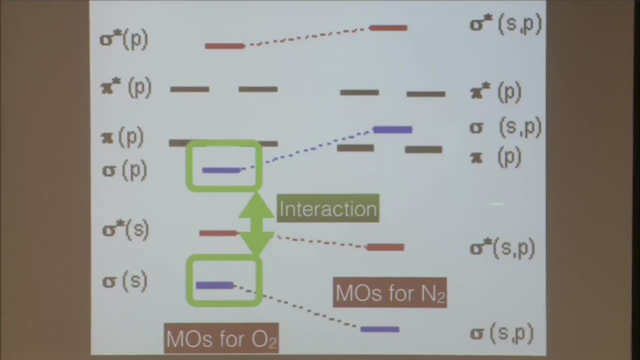 but that one goes up because that's the delta E, because it's able to mix in. It's able to mix in because they have the same symmetry And they're closer For those smaller atoms. they're a lot closer in energy. 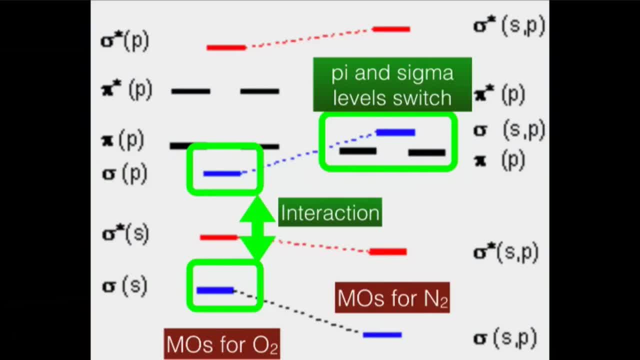 And so, if you look at this, what happens is those switch, They switch, It's real, They switch. Now, it doesn't change the thing I just talked about, which is the magnetic properties of N2, because they're still all filled. 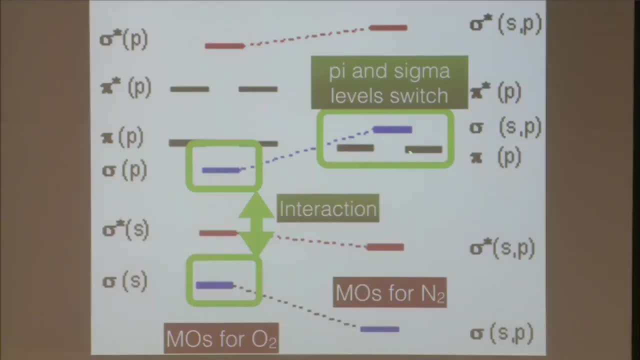 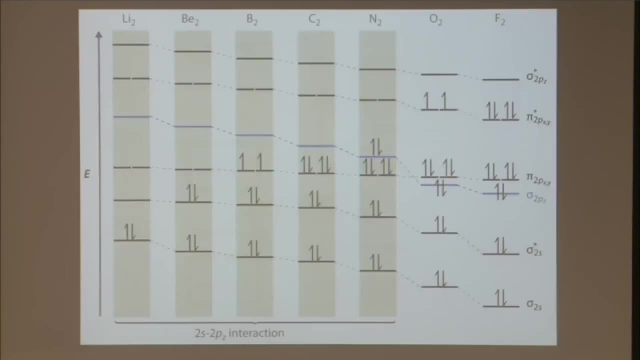 But it is important Because if I were to pull an electron out of N2, it would come from a sigma orbital, not a pi orbital Because of those interactions And those happen below O2.. So this is from your textbook And you see it says 2s, 2pz interaction. 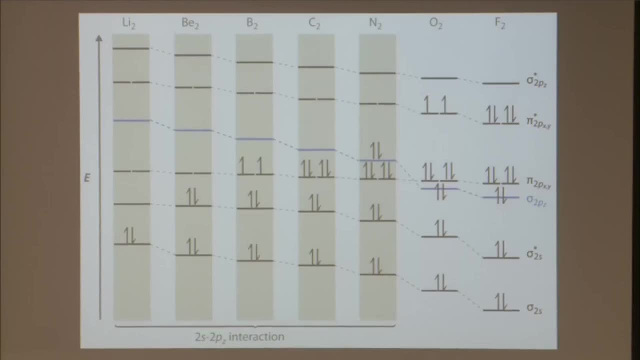 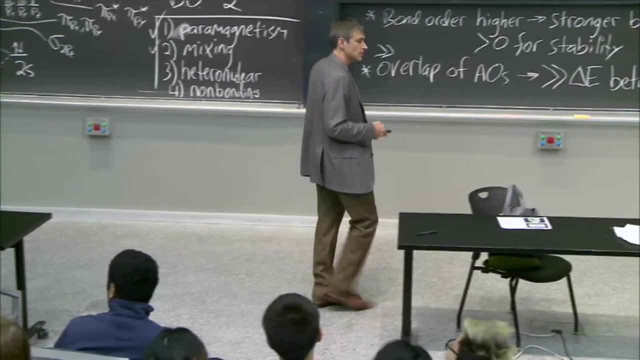 Remember, 2pz is sigma Sigma. same symmetry, able to mix. Don't mix very well here, But here they're strong enough to change the ordering of that orbital and that orbital. See that That's an important effect. 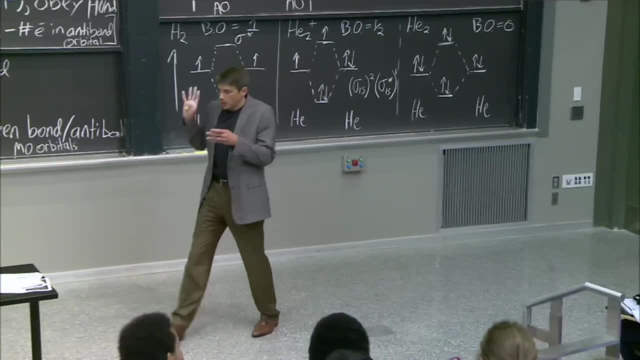 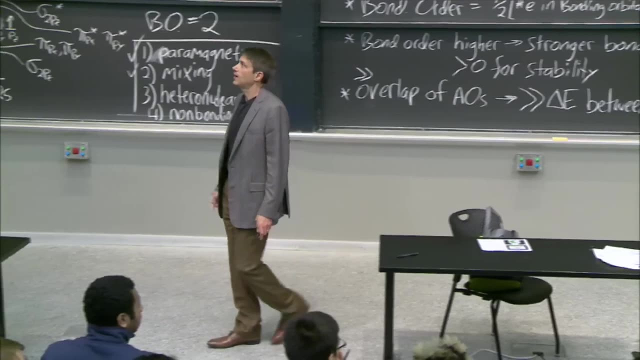 All right Now, but it only happens below O2.. It happens below O2, because that's where those energies and orbitals can line up in that way. Now there's two. OK, so we just covered that. Now there's two more things. 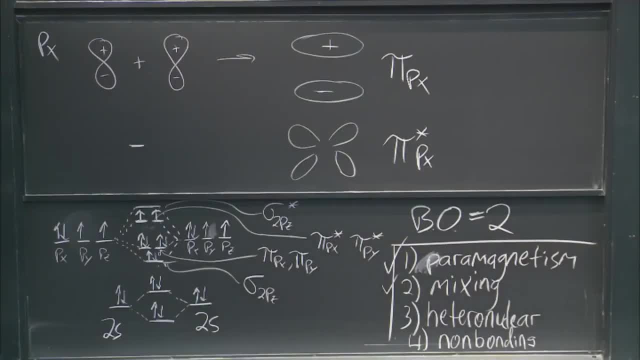 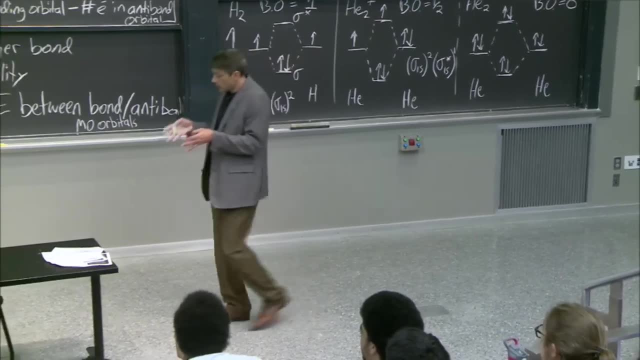 Two more things, And then that's all of MO theory. One is: I've been giving you the same atoms, but what if we go from a homolink nuclear dimer to a heteronuclear dimer, which just means one is one? 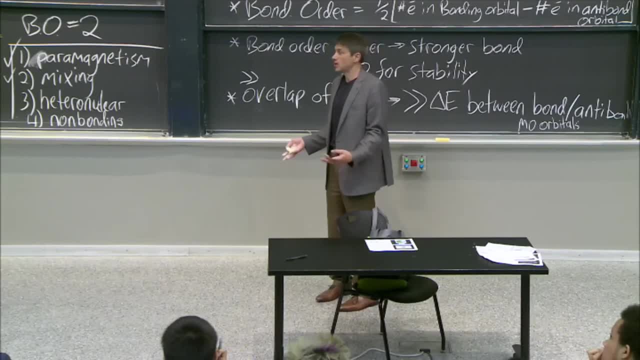 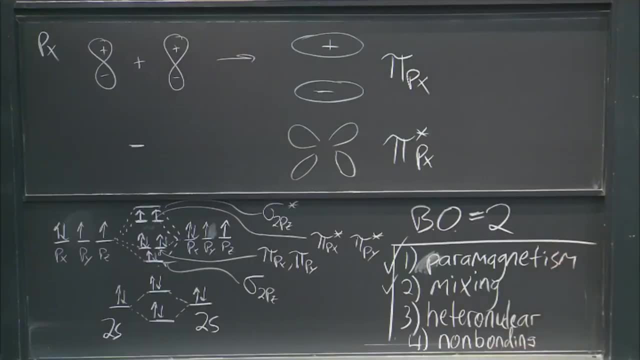 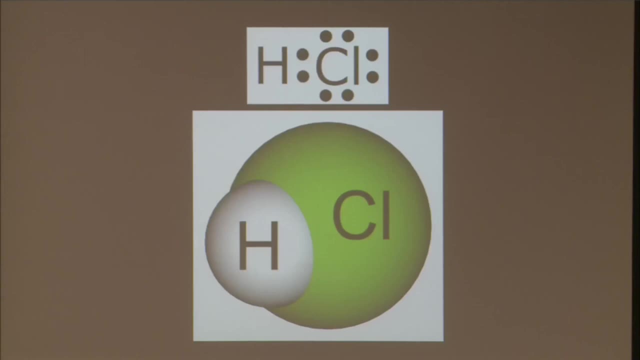 and one is another type of atom. How do we draw an MO diagram for that? And the second thing is what happens in this case? In HCl, H is bringing only one s electron to the party, But Cl is bringing s, is bringing p. 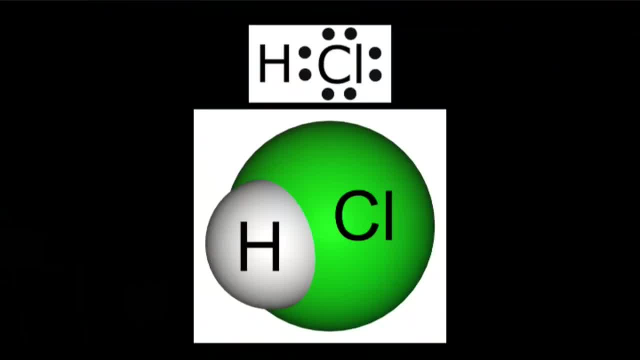 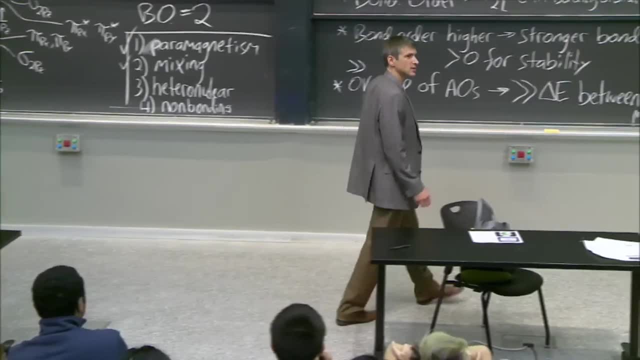 What does it do? How does the MO diagram look in that case where I've got all these extra electrons coming in from one of the atoms Right Now? I will not do this in 30 seconds, but I will next week give you a nice sort. 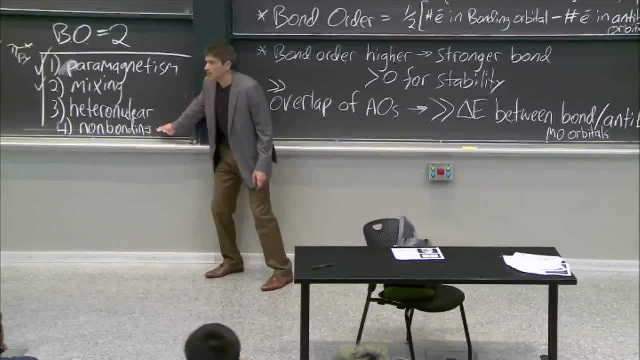 of thorough explanation for each of these two last MO cases. In the meantime, have a very good weekend.